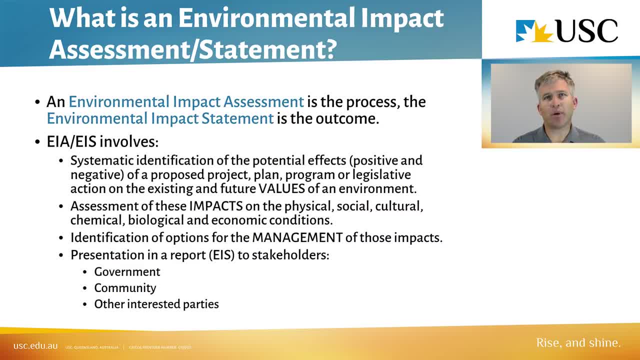 But the EIS inside it it's a systematic identification of ultimately those values, the potential effects- positive, negative, sort of it looks at both sides Of that proposal. that proposal could be anything from a plan, a project, a bit of legislation, a program. 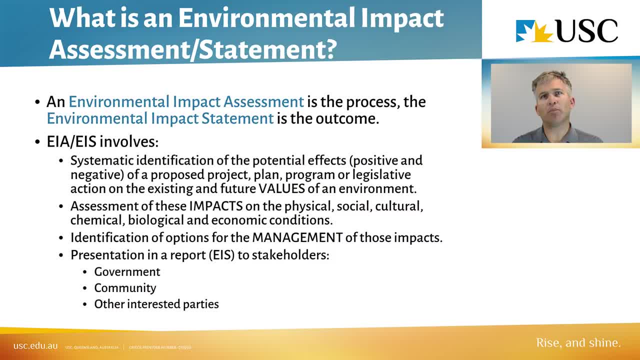 And it looks at those, the values that are in the, in the environment, and the values that the project offers in itself as well. Once it's, once it's done that assessment and identified those values, it looks more at those impacts And and those. those can vary. 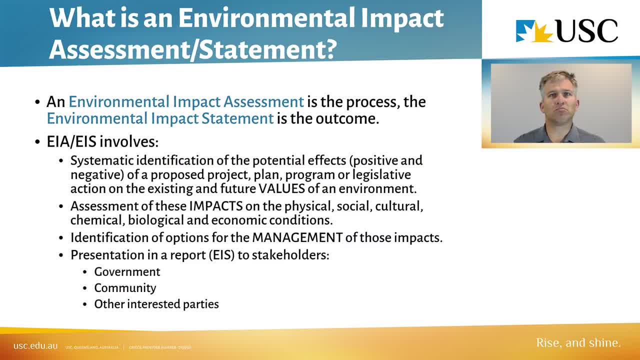 They have a physical, social, cultural impact, Cultural, chemical, biological, economic- all different impacts on that environment and all those different environments, And and so this process is to go through in a holistic way, assess and identify all of those impacts. 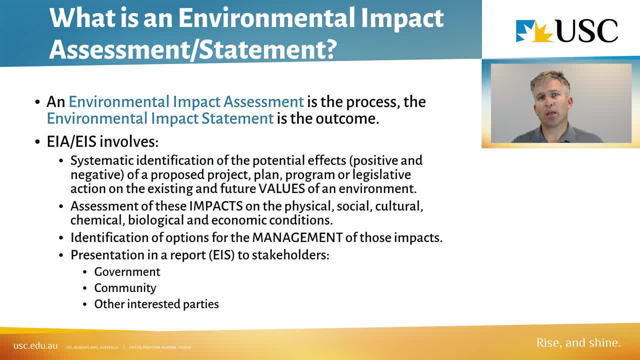 And then ultimately, at the end there, it'll come up with a way of identifying some effective mitigations. And then ultimately, at the end there, it'll come up with a way of identifying some effective mitigations Management processes- whatever you want to call them- measures in there to manage those impacts that are going to be imposed by that project. 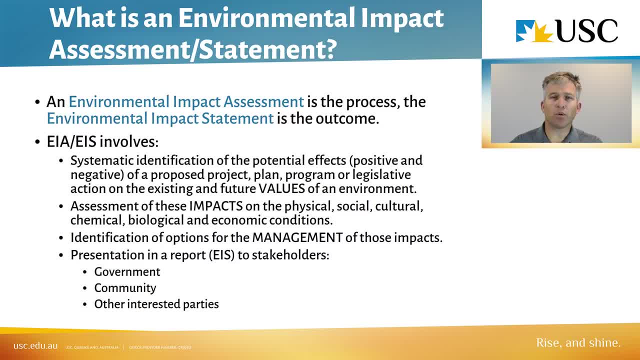 So, in a way, it's a very large risk assessment, which is what we did previously in one of the earlier modules, Where we go through and we look at the hazards and we look at, you know, we evaluate those risks and the impacts. 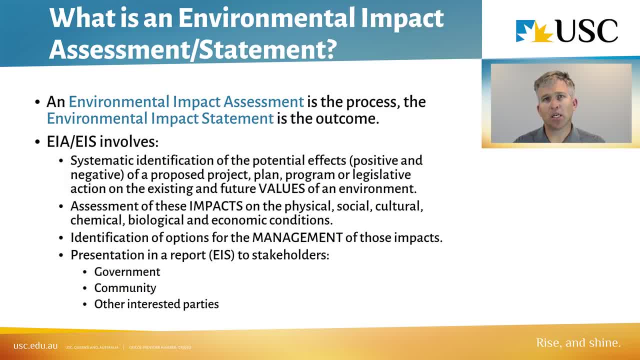 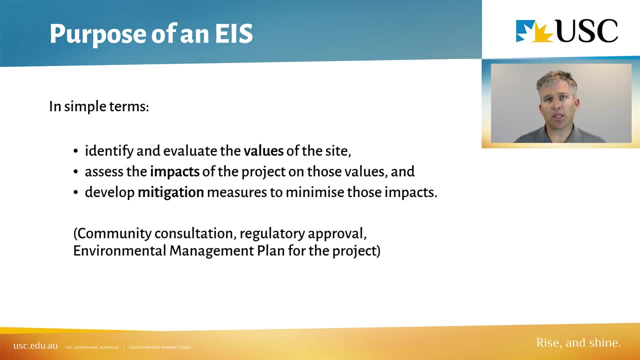 And then we go through and we come up ways of managing those risks. so it's in a sense a very similar process, but it's on steroids, it's a lot bigger, and then there's a great big legal pathway to follow. the purpose of an eis is to go through and assess three things. 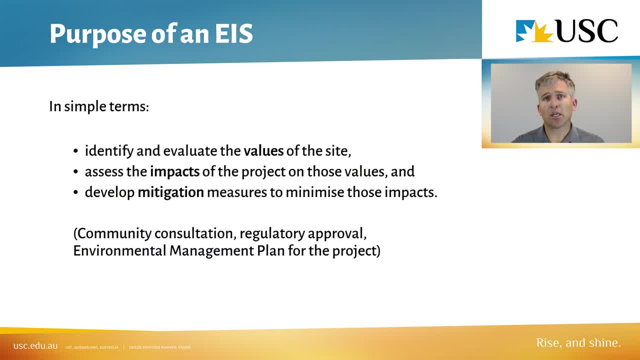 or identify three things as the values, the impacts and and identify some mitigation measures for you there. and and ultimately in that process, you're going to have a community consultation program where, i suppose, if you're lucky or unlucky, whichever way you want to look at, enough you'll be um, you'll be going out into the community, you'll be organizing, 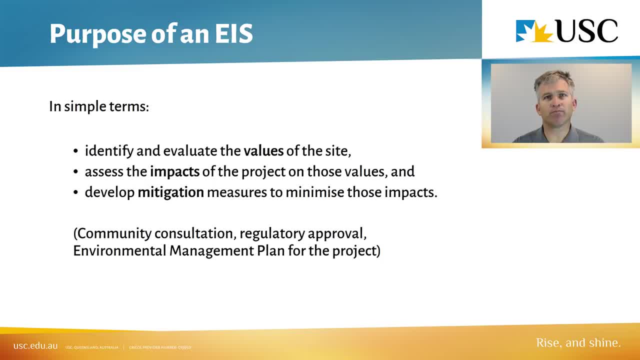 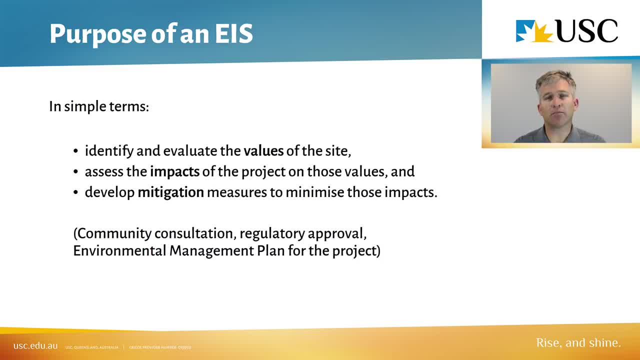 and answer questions and hopefully try and allay fears that may be with within the community, because generally that's their concern and that's why they're there and and you take on board all of those points and you'll take them back, submit them into the government and, at the same time, 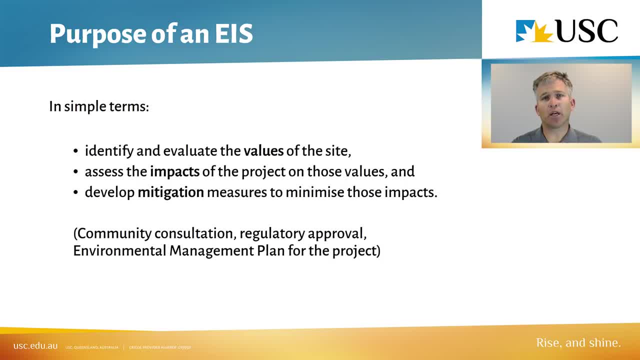 then go about putting together the information for that supplementary eis that we talked about just before. once it's gone through that community consultation process, it goes in for that regulatory approval. the the regulator assesses it, puts it up against um it's tests and measures and makes sure that it um it's it's compliant with legislation, that it's. 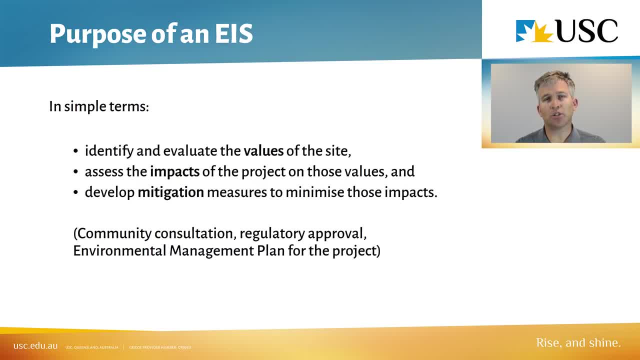 um and working in with industry best practice, that it's doing all of the things that it needs to do, that it's covered, all of the risks it's identified, all of the values. um assessed everything properly from my point of view, from a project implementation. uh, implementation point. 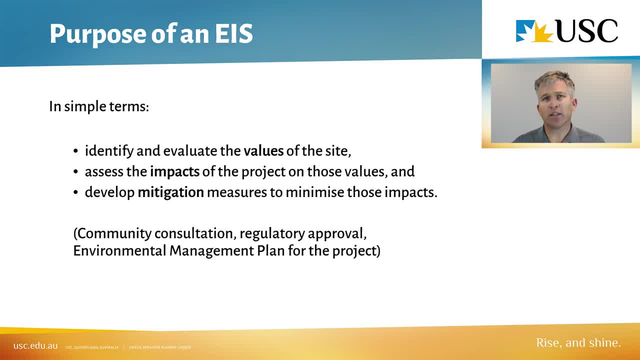 of view, the most valuable thing that i get out of that, that eis, apart from the tick in the box to to start work um most important. the most important thing that i get out of that, that eis, apart from the tick in the box to start work um most important. the most important thing is the. 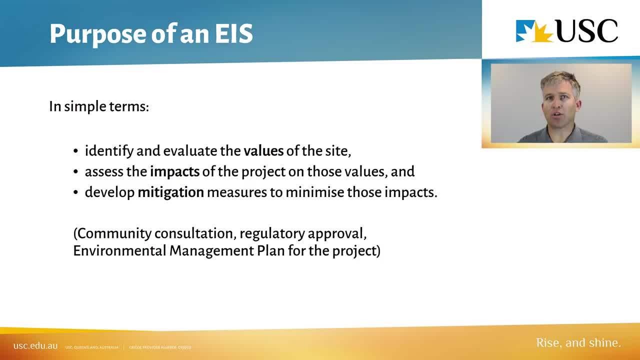 environmental management plan, the em plan, and that document more or less becomes your how to build the project from an environmental point of view. it's it's got those mitigation measures. from an environmental point of view, it's, it's got those mitigation measures. they go in, they go into the contract, which is absolutely paramount if they. 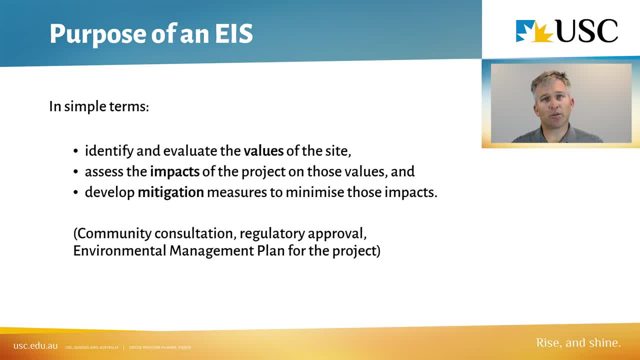 don't go into the, into the contract, then you've got a document that you have to comply with, but at the same time you have got no control over. you can't make a contract to do a unless you're going to pay them a lot of money. so it's, it's really really important, this whole. 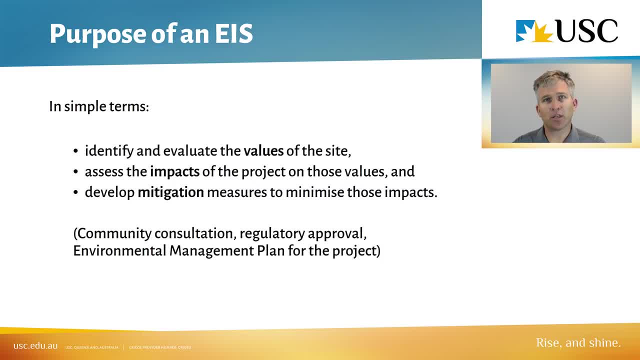 process is completed and you have an issued and approved environmental management plan before you go to issuing a contract for a contractor to go about building that job anyway, i'm probably digressing and moving well out of the realms of the scope of this course, but um, we'll touch into. 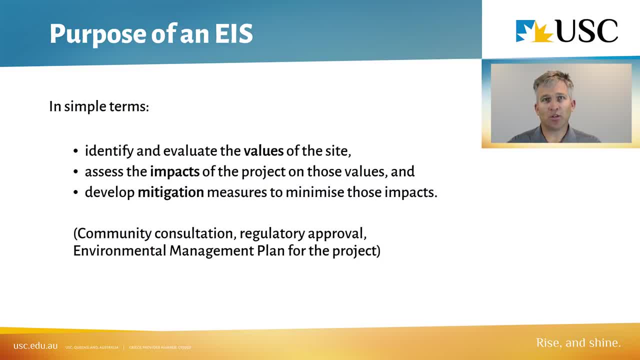 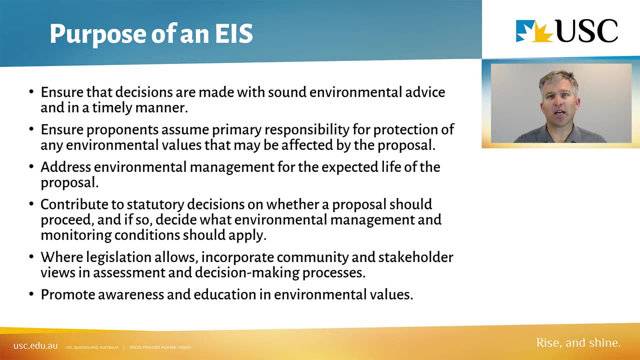 on the, on the, the next module in environmental performance and and that sort of area. i really i really enjoy that part um, so i look forward to talking to you about that. um. i will move on, however, um still on the purpose of an eis, and i'll go into a little bit more detail now. just 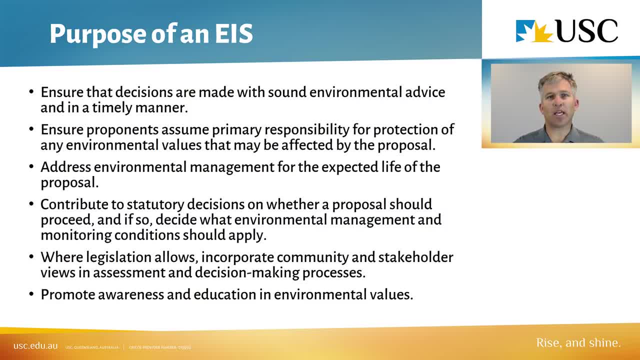 talking about um, this, the, the eis, and and what it, what it's going to offer, what it does, what it enables. on that holistic point of view, it enables decisions to be made with sound environmental advice and, most importantly, in a timely manner. and that timely manner gets really important because 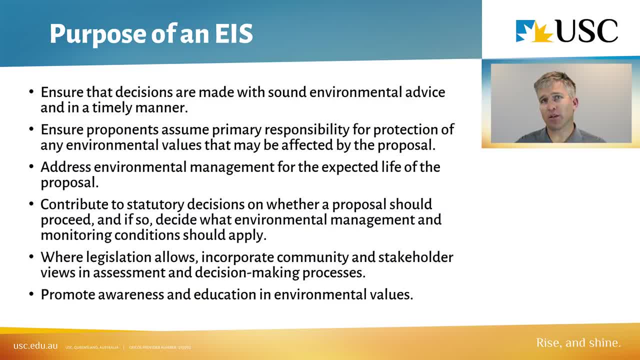 when normally an eis is sitting on the critical path of a project. and just to explain a critical path, critical path is that path where, um, if we look at a gantt chart, that gantt chart, we looked at the first, uh, in the first time around. 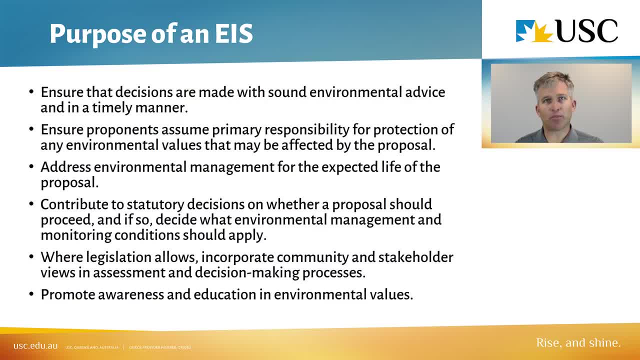 um, that's where any delay to any process within that critical path is going to extend or it's going to add, it's going to delay the completion date um of your project. so, um, if you've got one month to have an eis approved, or you know, realistically you might be long, but if 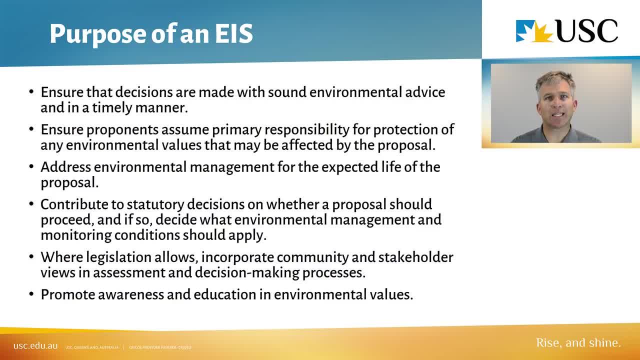 you've got one month, three months, whatever it might be, to complete a certain task and it's on the critical path and you take longer than what you're meant to, then you've just pushed out the end of that, um, pushed out that that completion date. and so from a project manager's point of view, 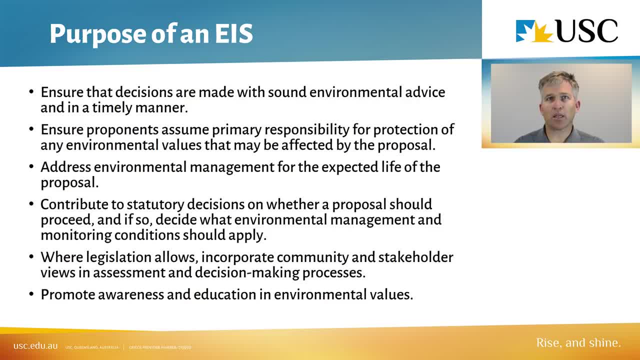 if an eis is on that critical path, um, they're going to be on your back. they're going to be making sure that you're hitting your deadlines and your timelines and the milestones and all those sorts of things. um, yeah, allowing it, allowing sound environmental um or decisions to be made. 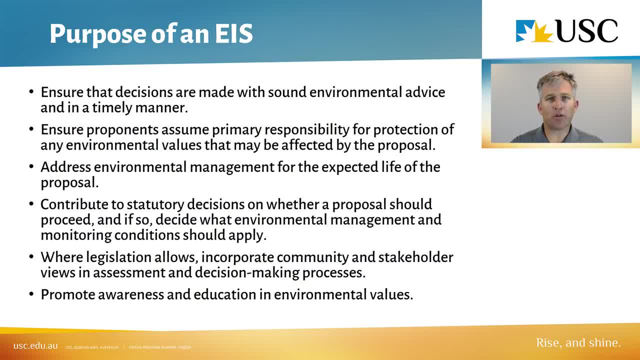 with sound environmental advice. um, because, as you know, if you want to sit down and make a decision, you want to see everything on the table, you want to see it all together and think, okay, i'm making a good decision, um, and so, from a proponent's point of view, they. 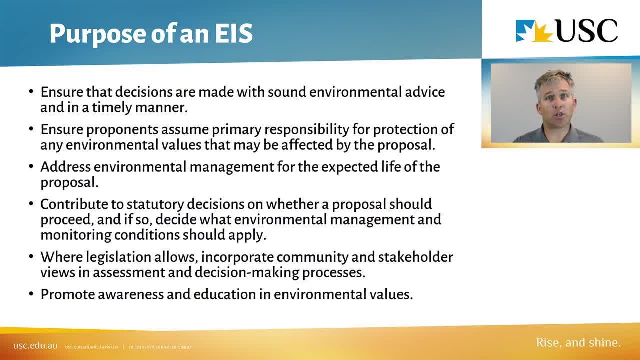 need to be able to make decisions as to um project design. they need to see we if we're putting a road or pipeline or power line in. they want to make sure that they're going through this area as opposed to that area because of whatever environmental thing there. 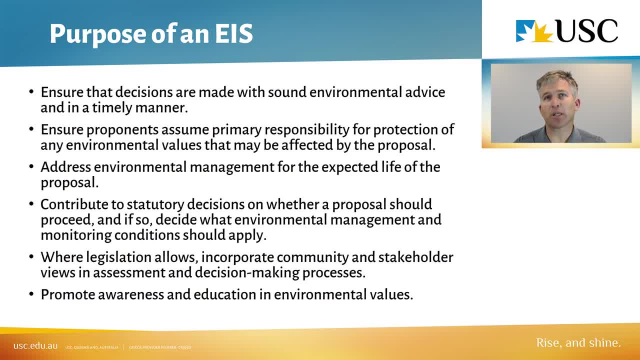 might be an endangered frog plant, something there that would be best if it was avoidable. um, so you want sound environmental advice? okay, also, um, ensures that the proponent, the, the entity, the company that's going about developing this project, let's say uh, is taking that or assuming that primary responsibility? okay, so they? um the proponent. 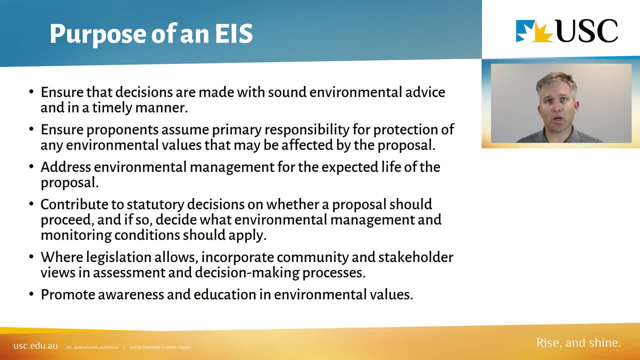 needs to go through, needs to make that full assessment of the whole picture and and then then take on board the information that it finds and takes it right through to the completion of that project. Next, we need to make sure that EIS is addressing environmental management. 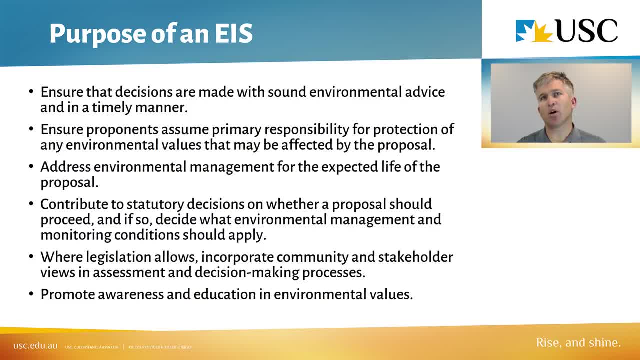 for that whole life. It's sort of been on that second point there, but that whole expected life of the proposal. It's a whole of life plan and an EIS has to do that. It has to go from the conception phase right through to decommissioning is a term that they'll. 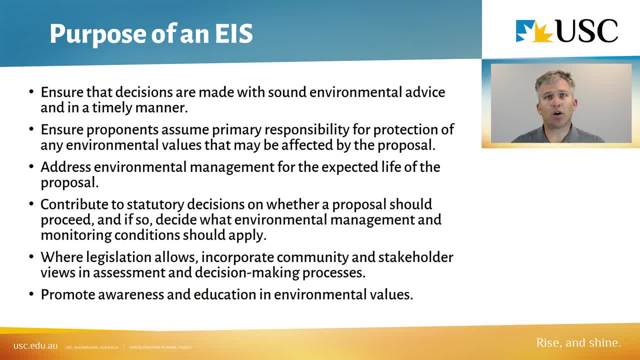 generally use. Decommissioning is when, in X years time, that pipeline might be worn out and it might need to be removed or made inert, dug up in certain places or dealt with in whatever way determined in your project description. It'll also contribute to statutory decisions. 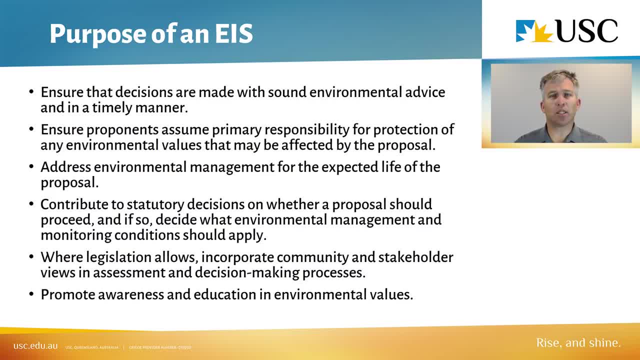 on what needs to be made, how it's going to proceed. So the regulators have got set pathways that they have to follow, And so this information comes in. it helps them to make those decisions and in accordance with various bits of legislation, and help them decide what sort of environmental management or monitoring conditions they will. 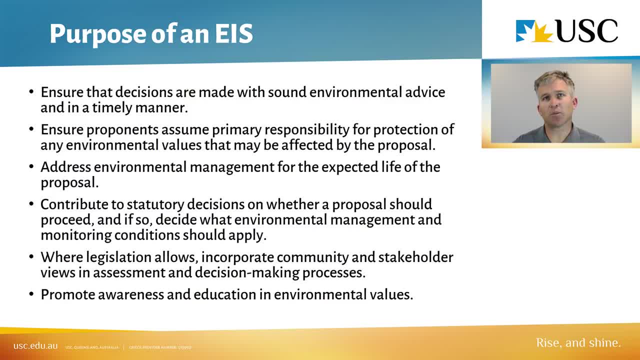 look at how comprehensive that assessment has been and then issue a set of conditions for that or with that approval, That's if it's fortunate enough to get that approval. but generally you'll get a set of conditions that go with it, And so this EIS helps the regulator to issue those sets of. 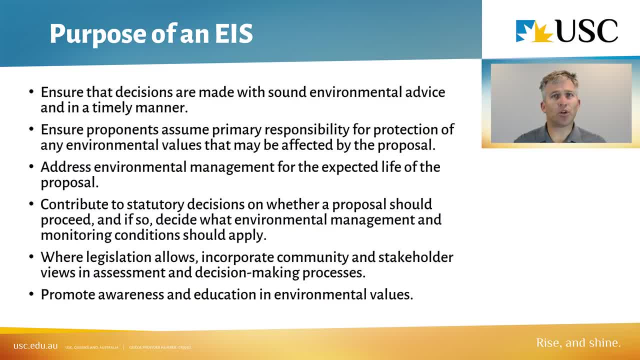 conditions that will go with that approval. Often you'll hear on the news that project X was rejected because of environmental conditions, or or let's say it had it was approved from an environmental point of view conditionally, And so they'll be an extensive set of conditions. 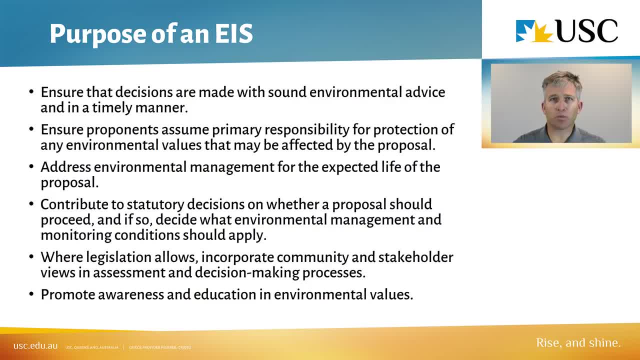 that'll be issued. I can tell you from experience on the recent projects. Well, the last five, seven years, the big Gasline projects with the Coal Seam Gas Industry and the LNG industry, Those big pipeline projects, we had thousands of conditions from various different regulators. That's. 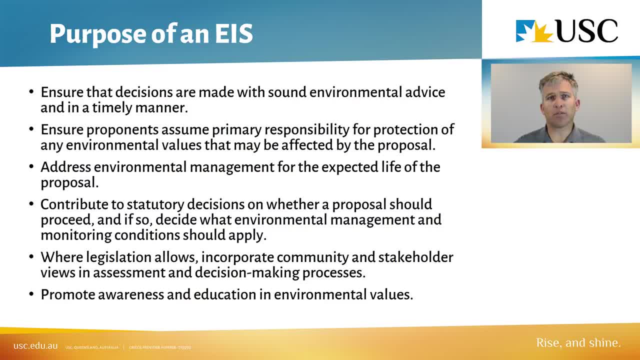 a thing. It was very, very complex. I suppose where legislation allows- and generally it promotes it, it allows the community and stakeholders to be involved in that process, in the decision-making process, from the point of view they have an opportunity for input in there to request. 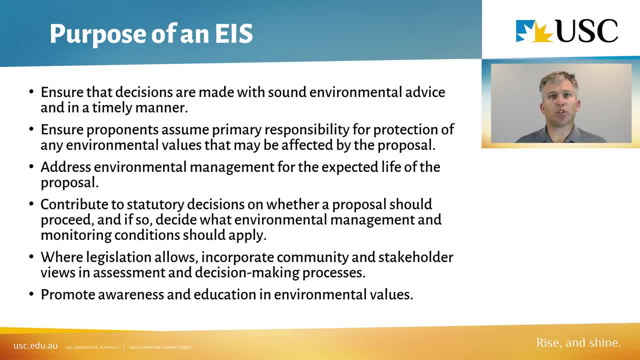 further information, which then, I suppose, assists that decision-making process And, last of all, it promotes that general awareness and education on environmental values. An EIS will go through, and it might do a pioneer in a certain area of study, And so everyone can, all of a sudden, 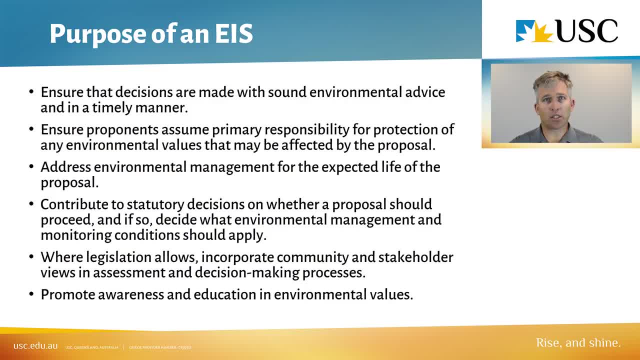 know more about that issue, that value, understand how it's impacted more. It allows a lot new information, which is why when you're doing a desktop analysis, you'll go back through past EISs and past project assessments and you'll pull out whatever information you can out of there. 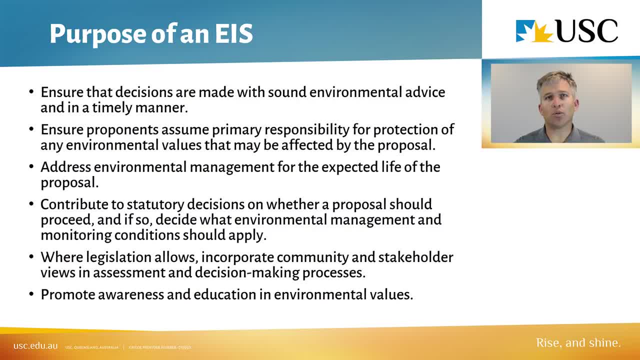 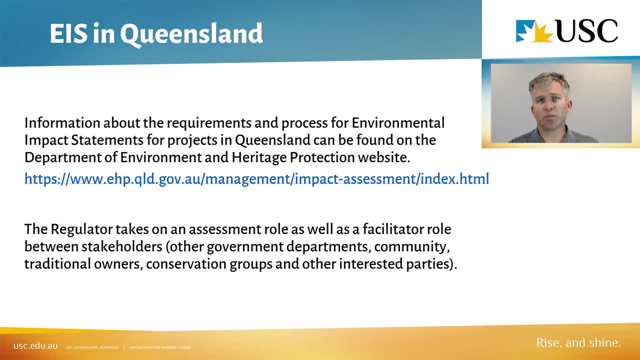 Because generally, that's where a lot of that sort of new information is going to be held. Okay, I've just covered a whole heap of information, and the majority of that information is held on this website that's up in front of you now on this slide. Go there, click on it or write it down. 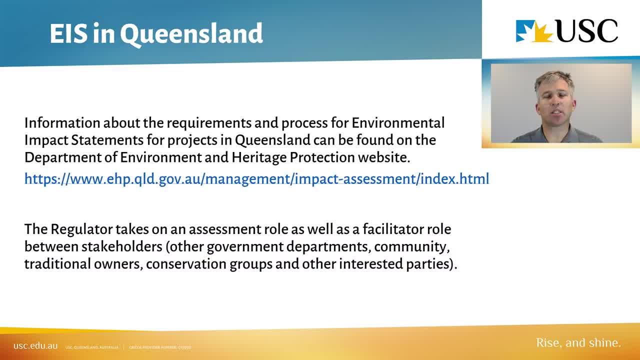 go to this link- unless it's for the Queensland legislation or EIS process, I suppose, with DEA on the website- And go there, because I'm not going to go into depth here, because this information here changes frequently, Every year, a couple of years. there's always changes going on here, So get in. 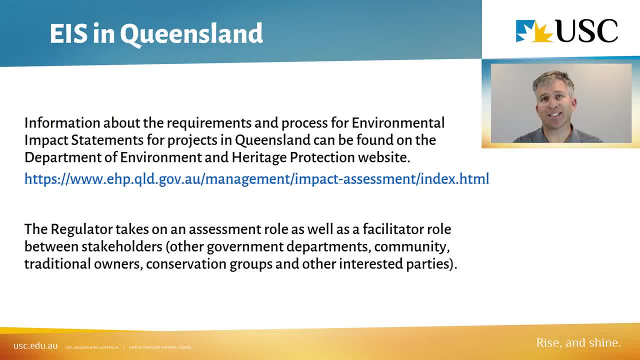 there and understand it and go, and I suppose go there semi-frequently if you plan on working there and understand the processes there. I suppose just to clarify the role of the government in this whole process, They're the assessor. 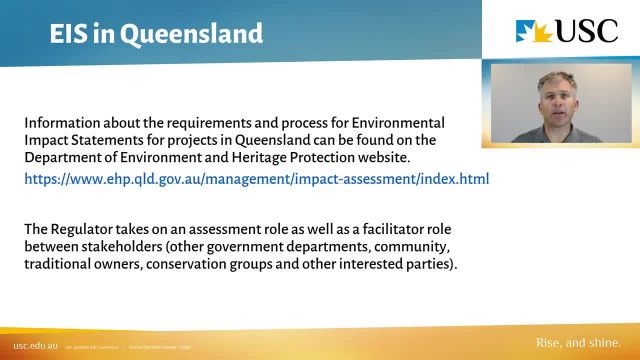 But they're all tomorrow. They're also the facilitator and they work with you, And on a big project particularly, but small as well, but particularly on big projects- they will assign individuals to assist you through this process And you may go and meet with them weekly, fortnightly, whatever it might be. 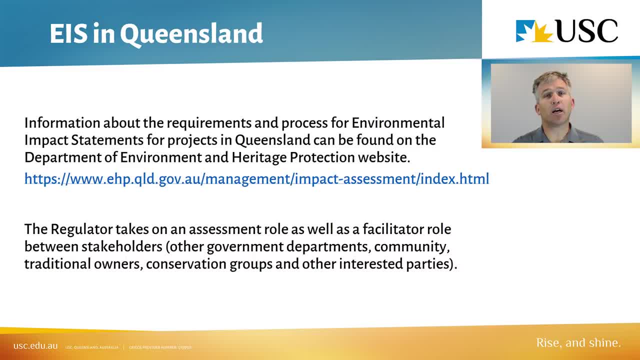 and there'll be one case manager and you'll work with that representative and they will coordinate information, be it information requests from the government, information that you're providing. They'll be the person you provide it to and then they'll distribute it back out to. 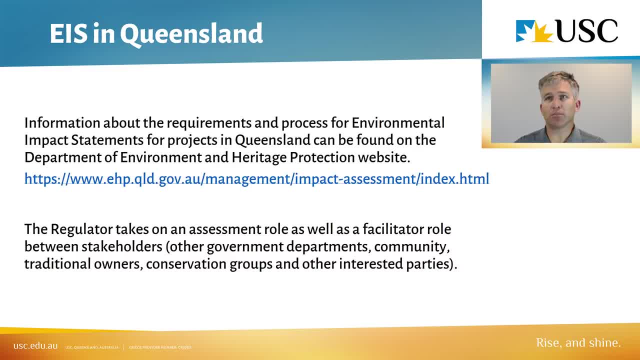 Department of Natural Resources or State Development, EHP, whichever government department it might be. They will then be that main point of contact and they will ensure people, be it on both sides of the fence, are meeting timelines and that sort of thing. 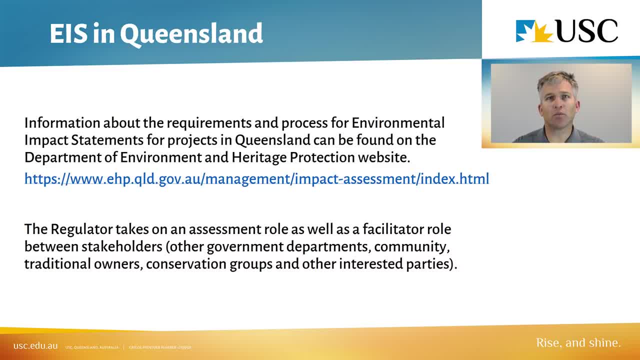 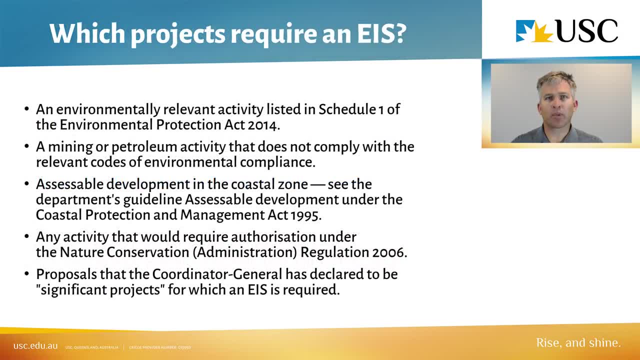 Anyway, my main purpose So this slide was to say: get on there and go right through it. There's a lot of information there. Okay, which projects require an EIS? Again, like my last slide, I'll direct you to that website. 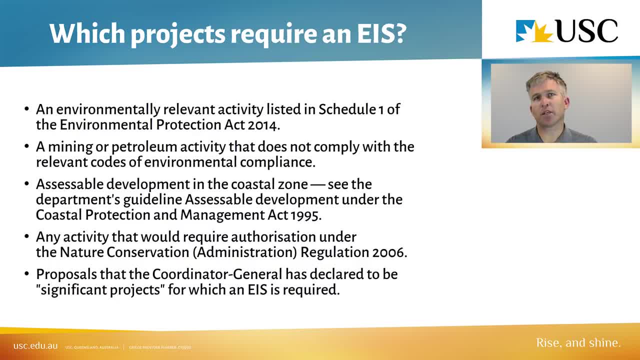 All this information is contained there, but we'll run through a few examples quickly. Environmentally relevant activities listed in Schedule 1 of the EP Act, Mining petroleum activities, Those sorts of things that are be it outside or don't comply with the relevant codes of environmental compliance. 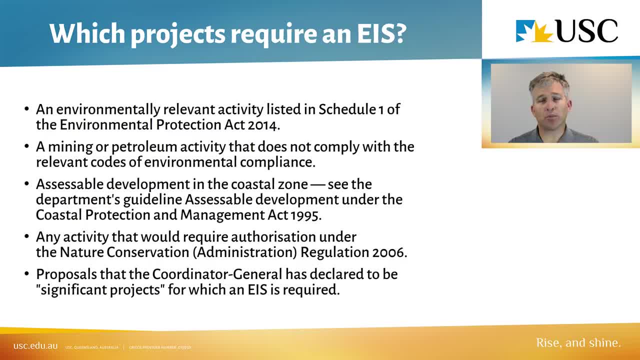 You'll see that it's things that are probably going to cause harm in some way. Okay, and so then this is a permit to go and cause a permissible amount of harm, if you want to think of it like that. But you know, it's an assessable development in the coastal zone. 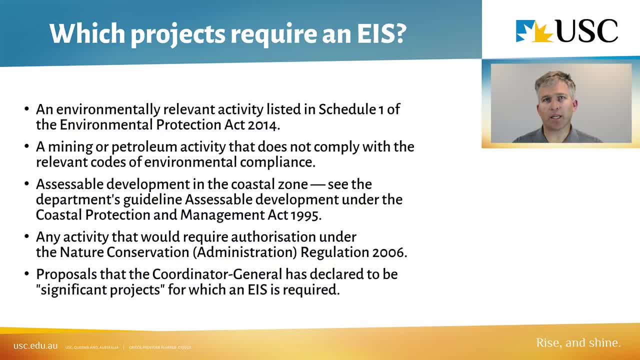 So, within the coastal zone, you're going to be digging things up out there And causing damage in a sensitive environment, An activity that would require authorisation under the Nature Conservation Regulation 2006.. Working outside legislation, So you're going to have to have that whole process assessed. 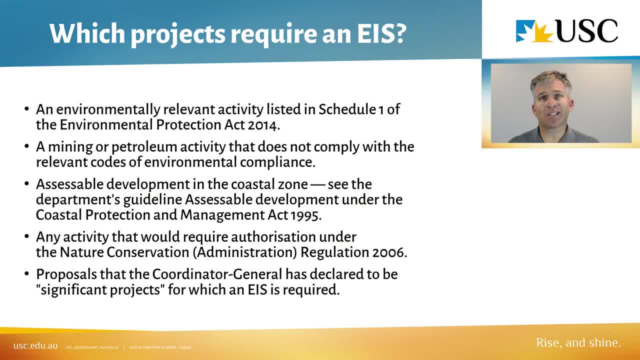 And finally, proposals that the Coordinator-General might declare as a significant project, And they've got you know you'll have to go onto the website and have a look at that- On how they go about determining Significant projects. But if your project is determined a significant project, then you'll be up for an EIS. 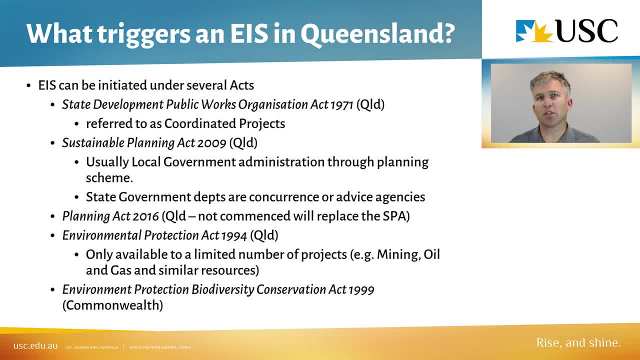 The triggering. I'll go onto the next slide, The triggering process of an EIS in Queensland. It's legislation based And so I'm not going to go through all of these bits of legislation, But they're there, they're on the screen. 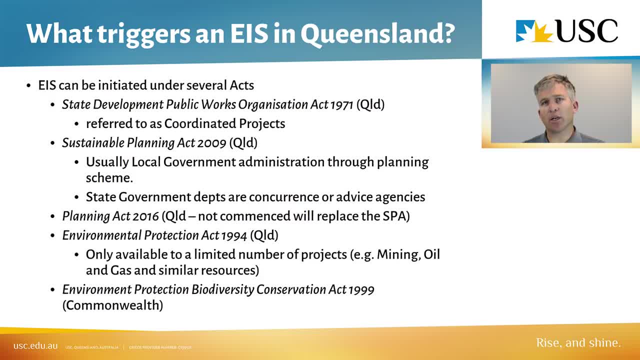 Make a note of them or hang onto the slide. EISs can be initiated under several acts, Many acts, And there's a state bits of legislation that we're looking at, Except for the bottom one. It goes down into the EPBC Act. 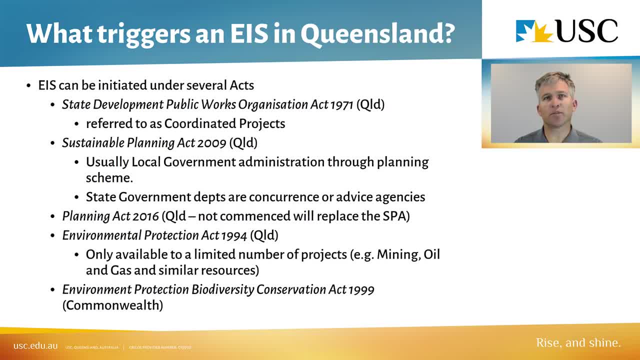 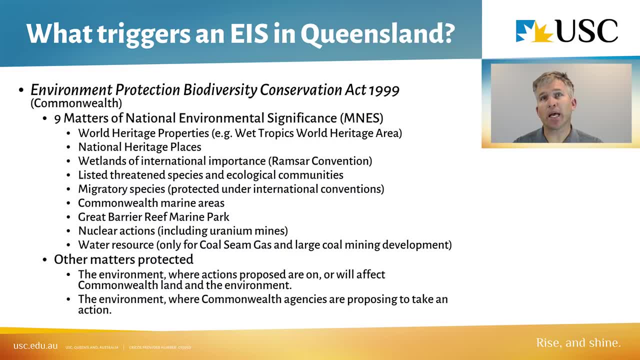 The Environment Protection and Biodiversity Conservation Act. Go onto the next slide here, And this is expanding out the EPBC Act And looking at all the different areas in there. So when you come to the EPBC Act, it's talking about matters of national environmental significance. 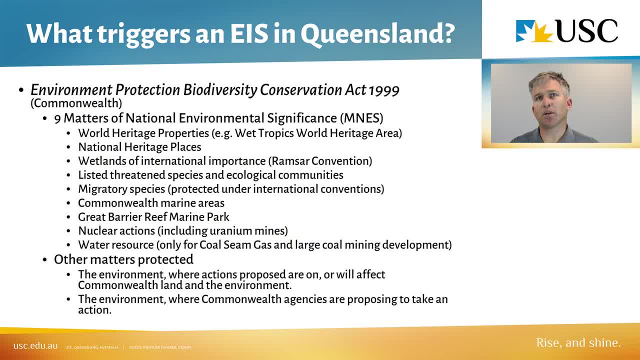 MNES. If you're starting to impose upon an MNES then you'll be up for an EIS in going through that process. Other matters: briefly, we'll talk about the environment, where actions are proposed that will affect the Commonwealth land. 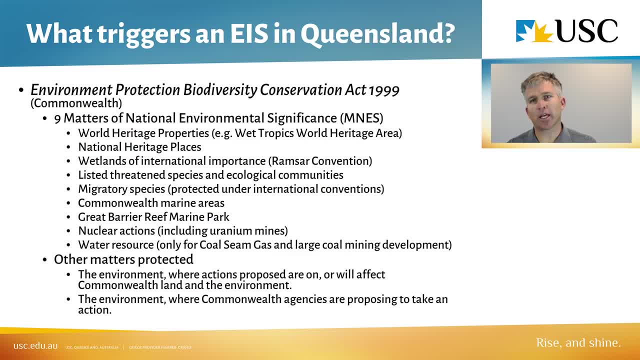 Or where the Commonwealth agencies are proposing to take action or do work or have something there. Those sorts of areas. If you're going to be doing work within those boundaries, If you're going to be doing work within those boundaries, Again, you'll be looking at an EIS. 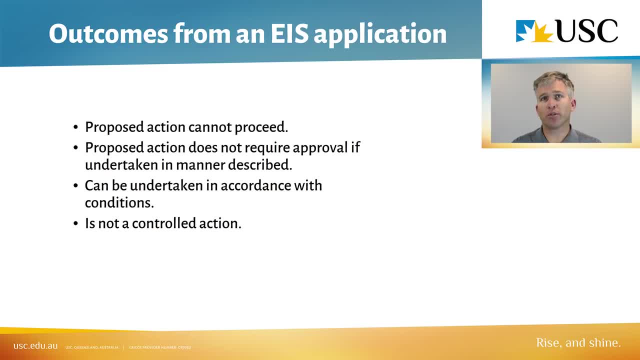 Okay, You've now gone through with the government's determined that we need an EIS for our project And you go ahead and you develop your EIS And what are the outcomes that you can expect from your application in there- And there are four. 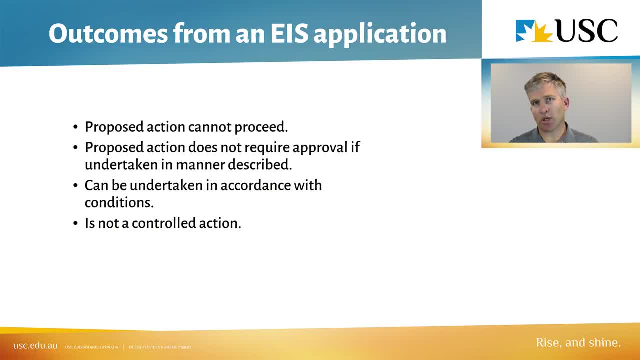 And we'll just go through them briefly. The first one is that you can't proceed. Okay, So your environmental approval has been declined. Number two: the proposed action does not require approval if undertaken in the manner that you've described. Your application has been really good. 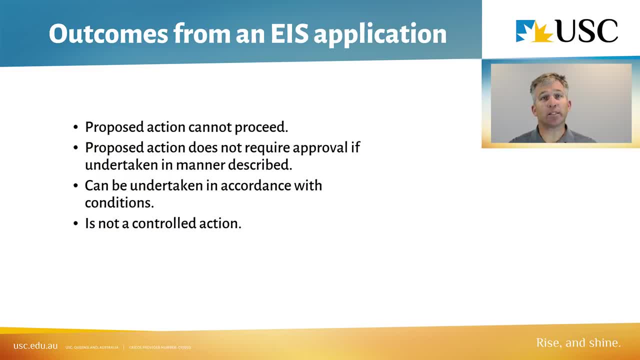 It's been able to convince them that you've got it all under control And that it's outside of legislation, So you're right to proceed, Or it can be undertaken in accordance with conditions. Generally, that's well on the projects that I've been involved in. 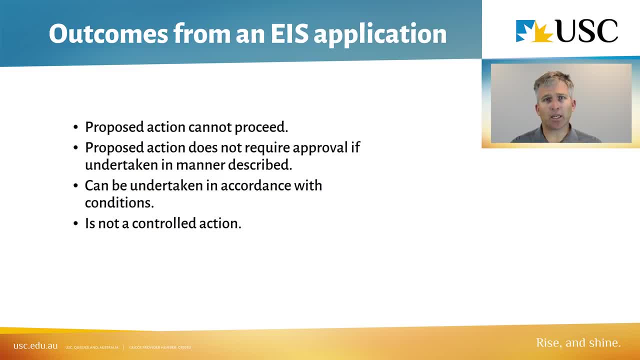 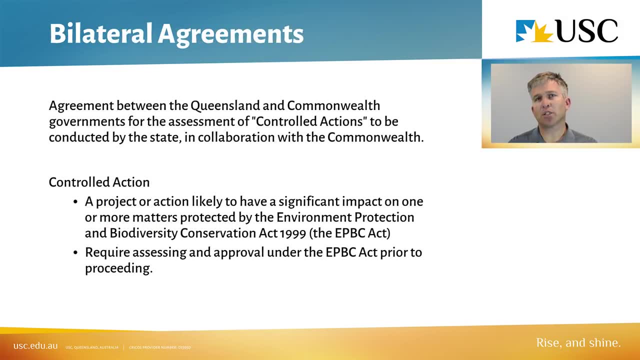 That's been the outcome that we've received there, And the fourth one it's not a controlled action. So again, don't need the EIS at all. And just to controlled action. we spoke about that briefly And I'll go in. 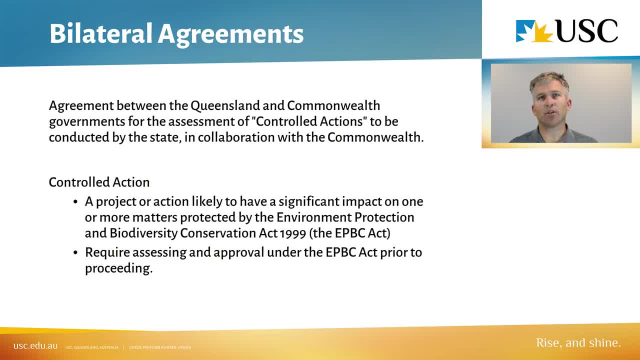 We'll explain that a little bit more And it comes down This sort of introduces the concept of a bilateral agreement. The bilateral agreement is an agreement that's been established between the Commonwealth government and the state government. A few years ago they operated independently. 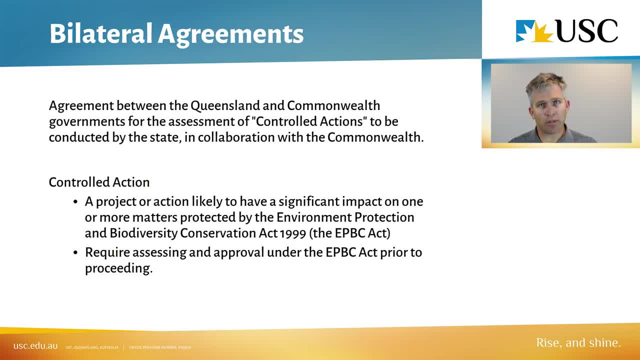 And if we did an EIS, you had to submit it to the state government And you had to submit one to the federal government And you were torn between: oh, do we put the same stuff in? but it's not applicable for each government. 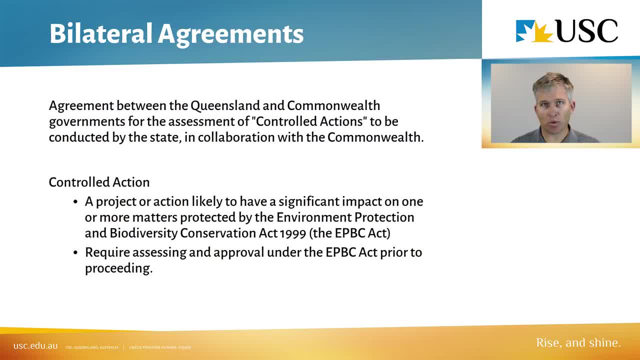 Or do you sort of have a different EIS, almost one to go for the state government to deal with all the state issues in the state legislation and one to go to the federal or the Commonwealth government to deal with all the matters of national environmental significance? MNES. 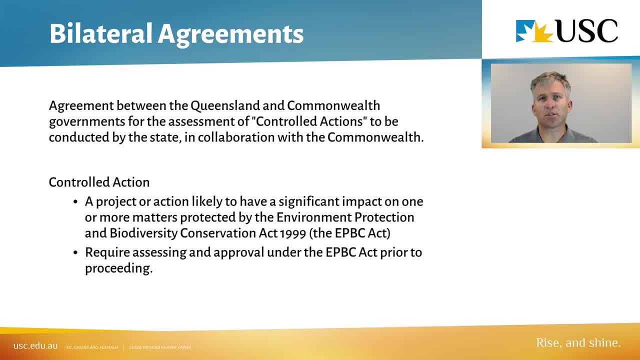 And it was a mess, because state government would be asking for one thing, Commonwealth government would be asking for a similar thing but slightly different. And it was difficult And at that time where I was sort of struggling, I was sort of in that hard place. 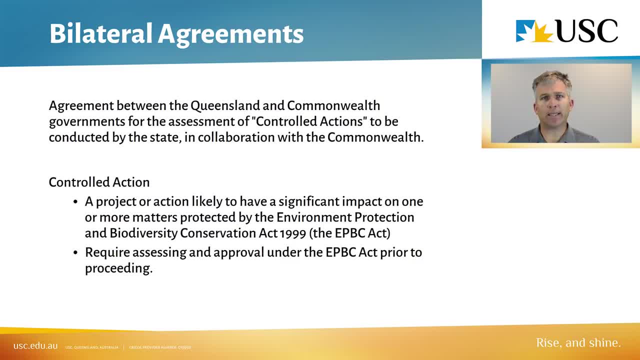 the government decided to come up with a bilateral agreement, which was quite handy, And so ultimately, it's an agreement between the state government, or the Queensland government, and the Commonwealth government, where they've talked about the assessment of controlled action, And so this controlled action is a project or it's an action. 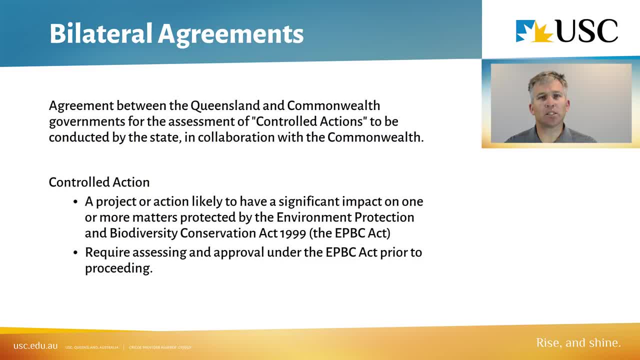 that's likely to have an impact on one or more matters that are controlled or protected by the EPBC Act- So like a matter of national environmental significance- And will require assessing and approval under that EPBC Act prior to proceeding. But generally that assessment is done by the state government. 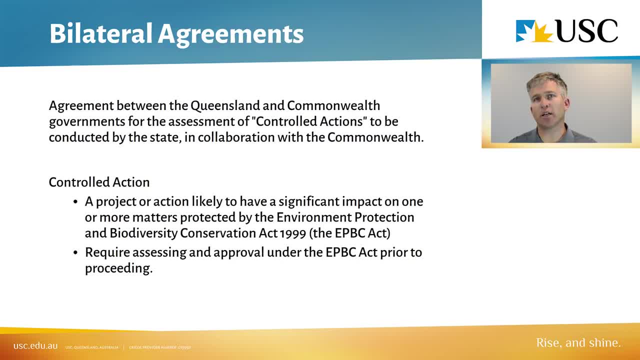 So you remove that toing and froing. It all goes into the state government. The state government manages it, It coordinates it. If it's outside their capability it can go to the Commonwealth government And there is room within the legislation for the Commonwealth government to come in at any time. 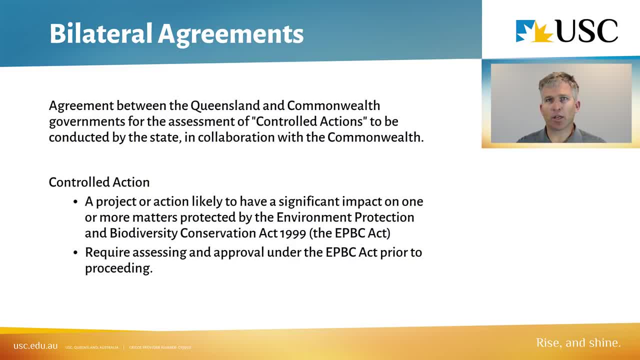 and do an assessment on it, If it sort of thinks: oh, what's going on here? We want to have a little bit more control. However, it's been delegated. I suppose that responsibility has been delegated across to the state government. 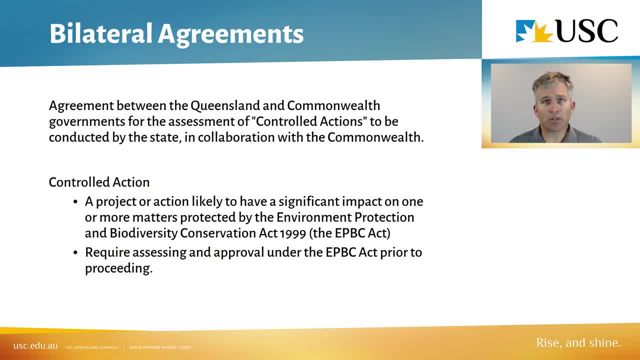 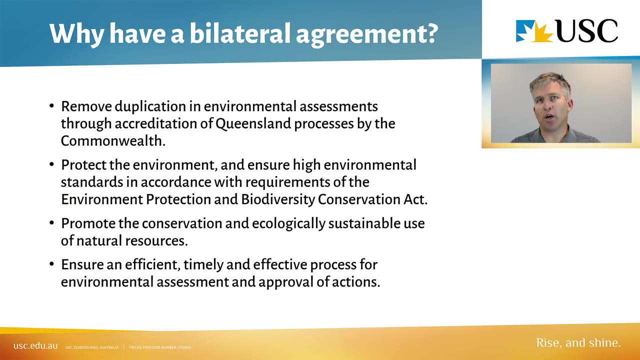 And now they. it's actually a certification process, So there's a formal process where the state government has to operate to a certain standard, But that state government is able to assess a controlled action. I briefly spoke in the last slide about why bilateral agreements have come into existence. 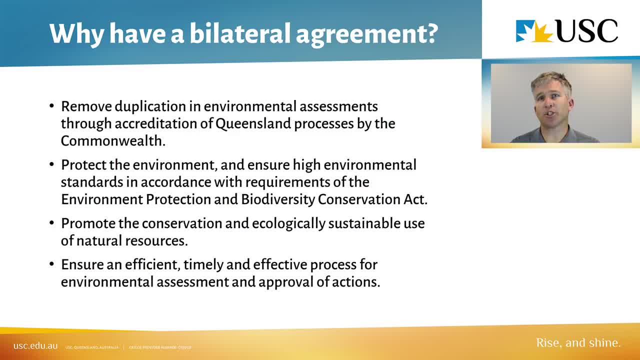 And ultimately it is to remove that duplication in that environmental assessment process when it gets caught up between the Queensland and the Commonwealth government. Yeah, It had been a real, real sore point in the past, I suppose, But it also serves for a few other purposes there. 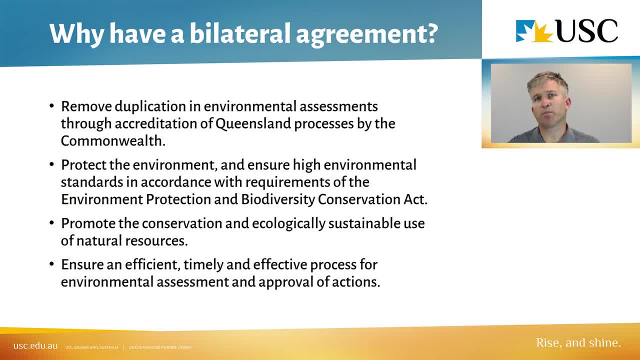 which I think sort of comes second to that, But it talks about having high environmental standards that are set within the EPBC Act. So it's again that certification process that the Queensland government had to undergo so that they could go about doing that appropriate assessment to that certain standard. 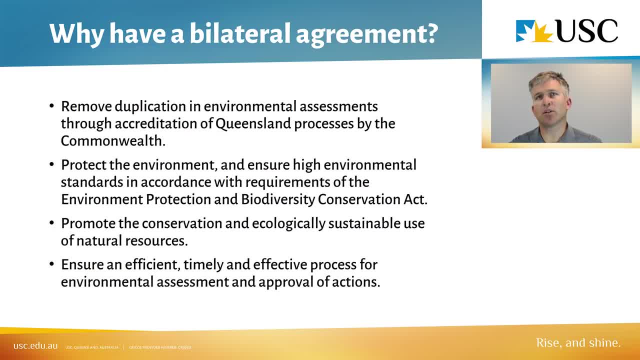 It's also to promote that conservation and ecological sustainable use of natural resources. And there's, I suppose it's tied in a little bit with that first point- is it ensures an efficient and timely and effective process for that environmental assessment and the approval of plans. 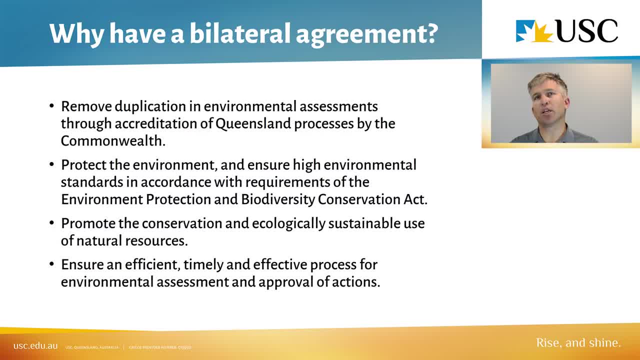 Because in the past I know with the Commonwealth government, they in the legislation they would define a minimum amount of days for an assessment and I think it was 20, 21 days where no 20 business days. 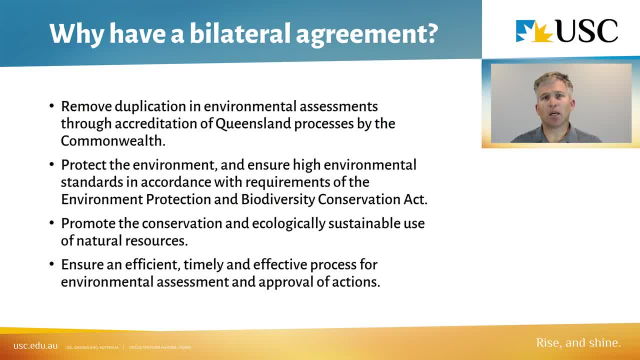 so it would have been four weeks, And so that was your minimum timeframe for that approval. But there was no maximum timeframe assigned, so you'd be left in the lurch, thinking when are they going to approve this thing? So there's a much clearer pathway. 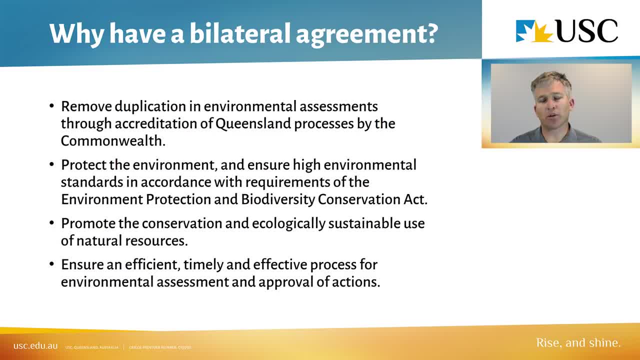 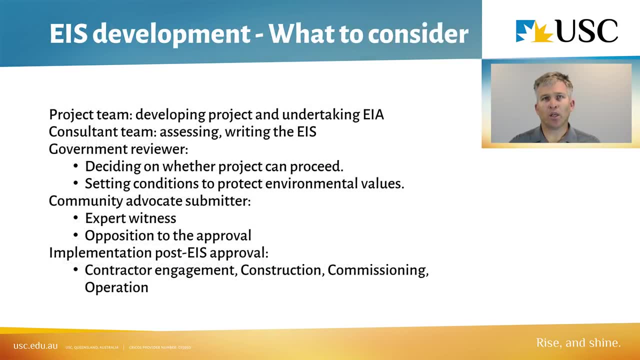 that's been defined now because of these bilateral agreements. Anyway, the important thing to remember is if you trigger something that's in the EPBC Act, then you'll be dealing with the state predominantly. OK, we've touched on the legal pathways. 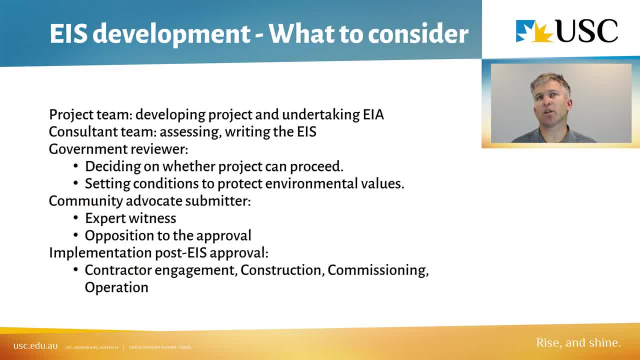 and processes for the assessment of the EIS and generally why we have them and what they're meant to provide. We're going to move on to now what we need to consider in the development of an EIS and how we're going to go about doing it. 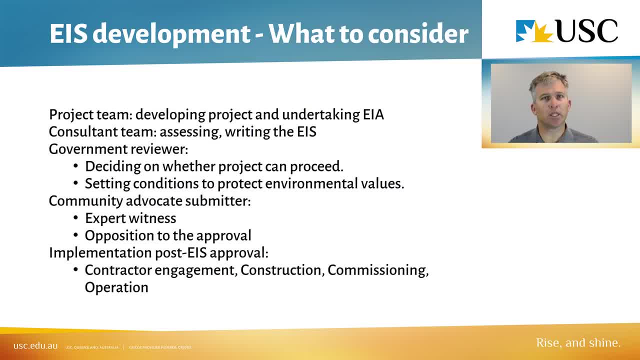 what we're going to put into it, et cetera. So to start with what we're going to consider in the development of the EIS, Initially we're going to look at the project team that's developing the project and that's undertaking. 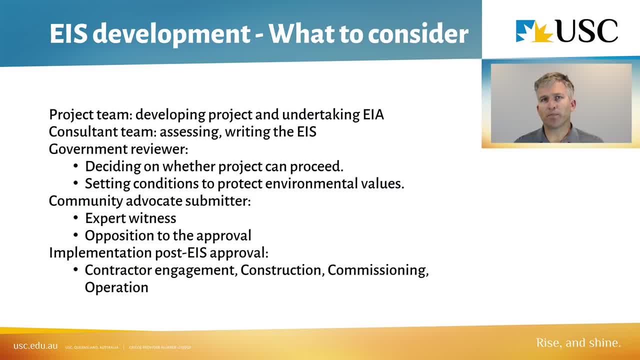 that environmental impact assessment. So your team generally say that's the proponent Man. you're going to build a high-rise, building a car park, a road power line, whatever it is, But it's that management team generally. 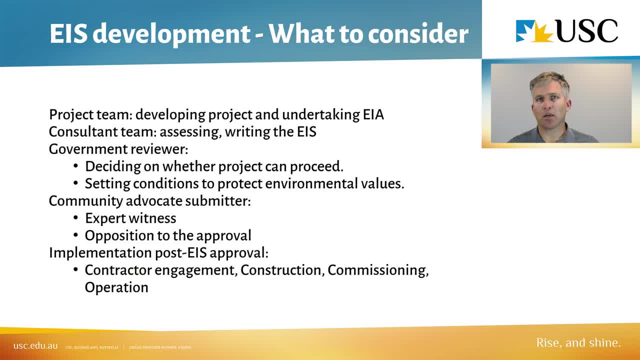 and it'll be made up of a group of engineers and a construction manager, a project manager, safety, environment, quality, all the different reps, That's the thing. But you've got a project team And you're considering who is in there. 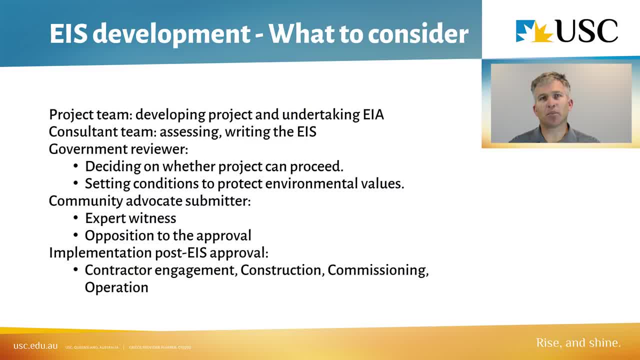 what expertise does that team have, because a lot of the information is going to be coming from you. So that's the engineering and design team, And they need to be working really closely with the EIS team. And that steps down to the next row. 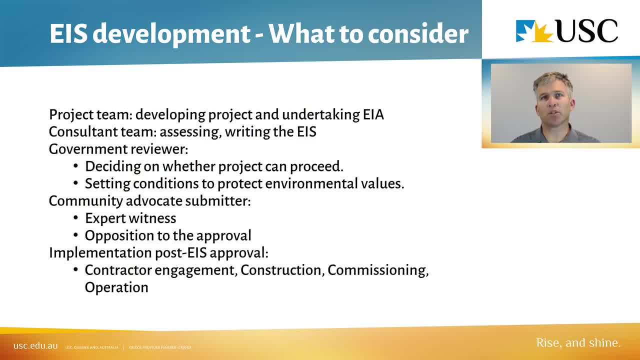 That EIS team is generally a consulting team, So you've got to pull in different experts: your flora, fauna, ecological, soils, water, noise, community, cultural- all of the different experts. So you're going to pull all of them in. 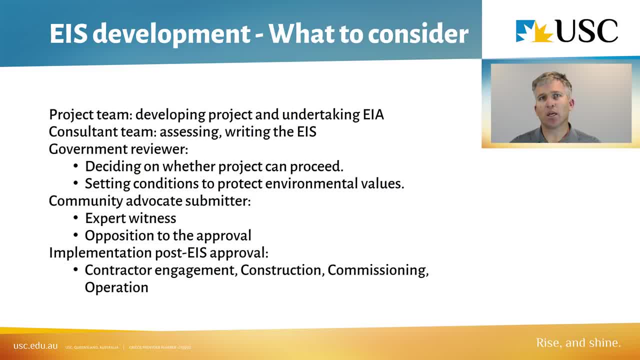 and have a big team. They're going to go and do the assessment and identify and assess the impacts. ultimately, Then you'll come in together, work with the engineers to come up with how you're going to manage those impacts Moving outside of your team, I suppose. 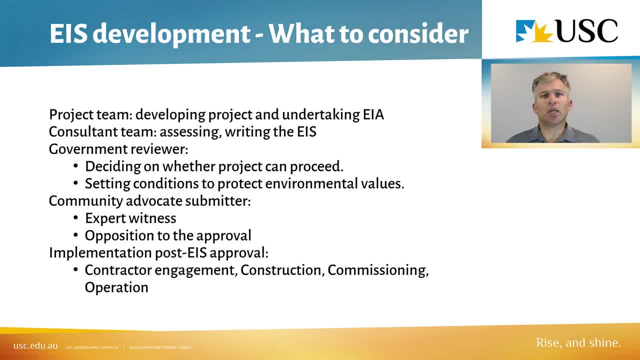 you go into the government reviewer- the government reviewer or the regulator- So the document gets submitted into them. You're working with them during the development of that document so that you know what they want and they're aware of what's coming. But they're going to be making the decision. 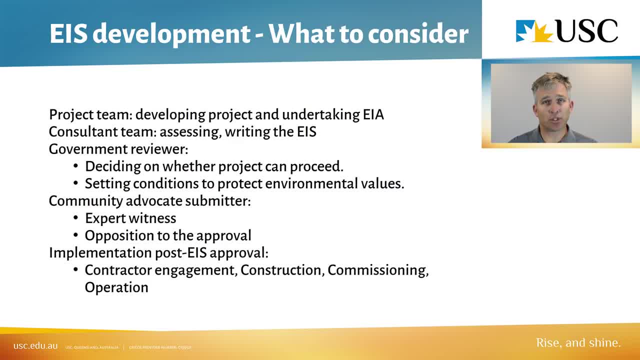 on whether that project can proceed or not, whether they're going to approve it, And they'll also be looking at assigning conditions for that project. They sort of sit on the other side of the fence, But then there's sort of another area. 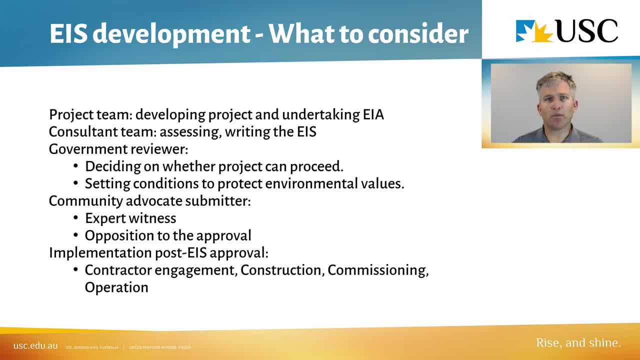 sort of another fence with a side, and that's the community. And they're out there. They're going to be most concerned with what you're doing and most interested in how you're going to go about doing it. You've got you've got groups within the community. 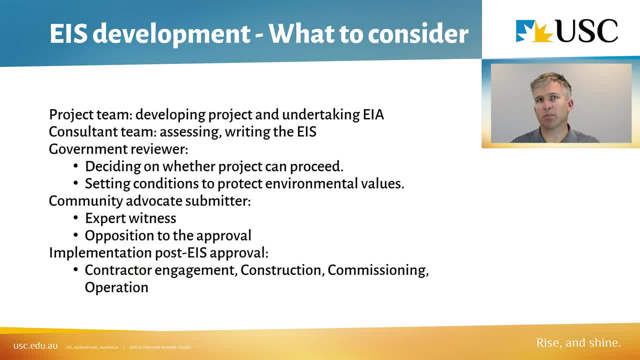 who will be opposing it, who will be putting submissions in to the government to request that it be declined. They're going to be providing evidence. There might be expert witnesses talking about the detrimental and irreversible impacts that that project may have and all other sorts of opposition to the approval. 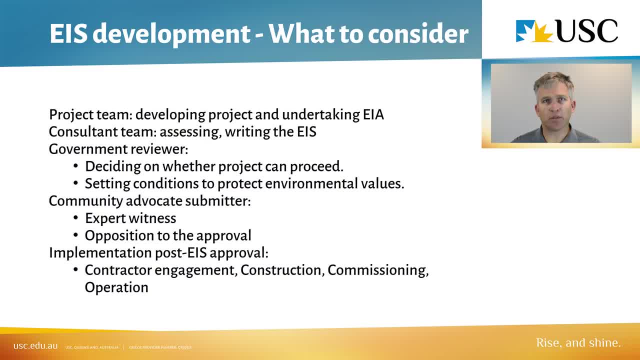 be it the general, not in my backyard sort of individual through to those who do, They're going to have a really deep-seated concern. It changes their life and it's saying we need to take into account all of those concerns. The final: 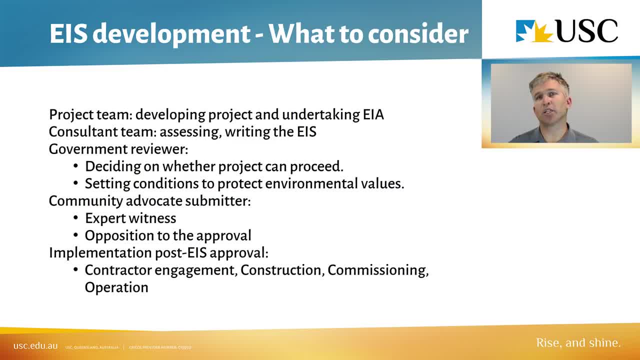 final part is the implementation of that project post the EIS approval. And so that's where the rubber hits the road. There's one thing to go through that EIS process, but sort of there are no. no animals have been injured during the development of that EIS. 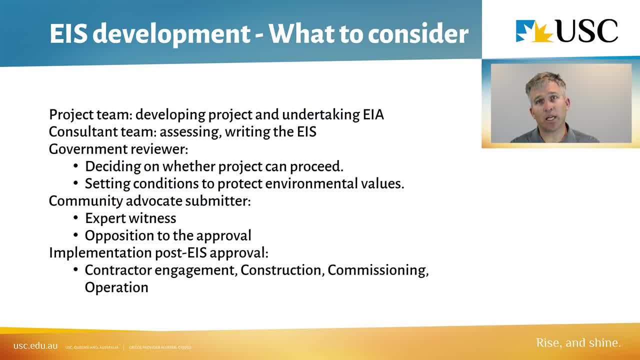 if you know what I mean. But once that EIS is approved, you're looking at habitat destruction, injury and everything else that goes on with that to the environment. Those impacts are going to come about and you're going to have to manage them. 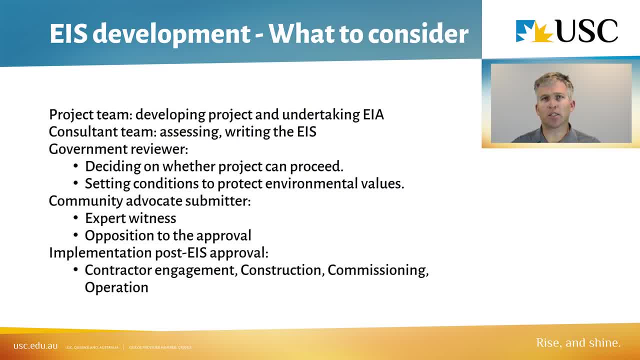 And that's sort of something that I've realised through my career is that you're out there and you're watching that impact go on And your purpose is to be there to make sure that that impact's managed and that you go about that process of putting it back the way it's meant to be put back. 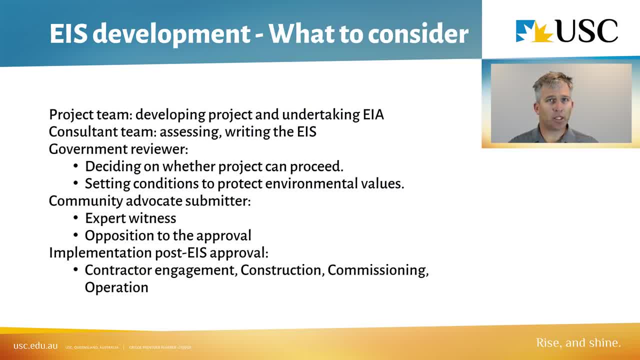 that you're going about keeping the promises that have been made during this EIS development process, And I see that implementation process. that's where all the promises are kept, That's where you have to work hard to go about fulfilling those obligations And at least 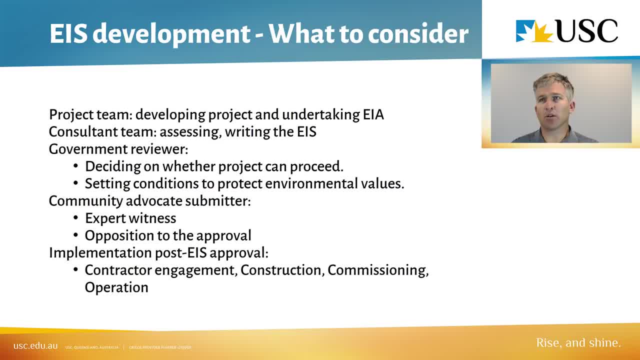 and if you can get to the end of the project, as I did on one particular project. I had a landowner come up to me and say he said: look, I don't like what you did, but I like the way you did it. 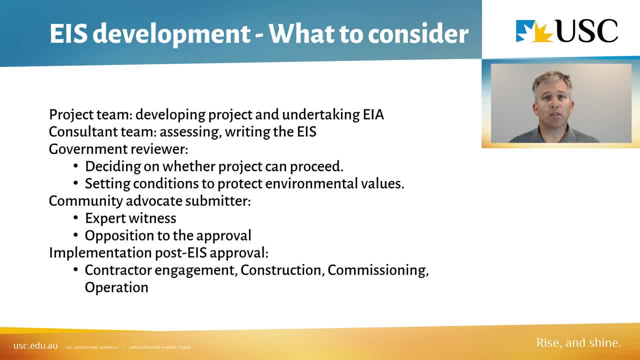 And I took that as quite a personal compliment, because I had no influence over whether that project was or was not going to go ahead. It was going to go ahead, And it was made by people that sat way further up the tree than me. However, when the rubber hit the road on the ground- 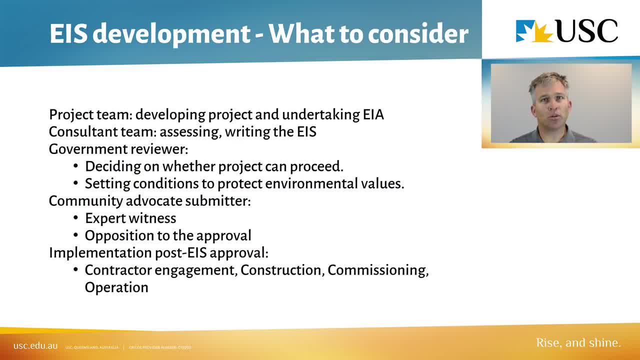 when the bulldozers were moving through, I made sure that that what occurred was what we said was going to occur. And to get a compliment like that, I'll take it with me forever, because you just feel like, okay, I've done my job properly. 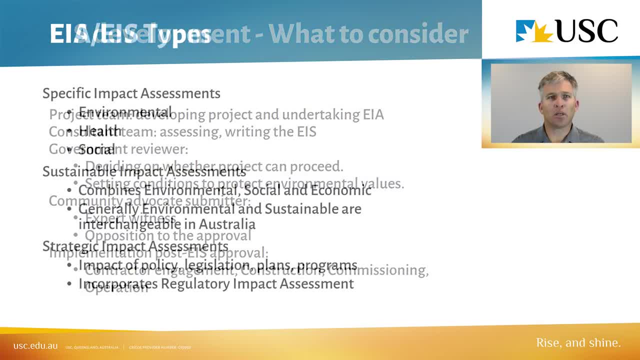 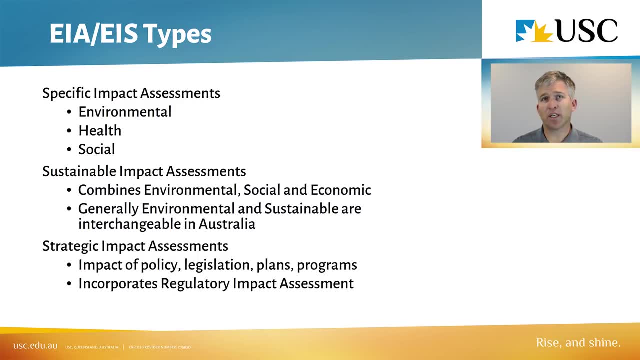 And I hope you guys experience that as well. Right, EIA, EIS, types And I suppose EIA EIS is used fairly interchangeably and EIA being the assessment is more the process and the EIS is the statement. 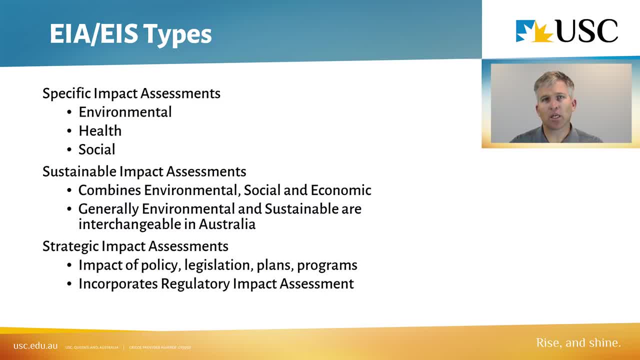 That's the document, That's the actual end product, And they are used very interchangeably, And I do. I use them very interchangeably myself, But generally I'll be talking about an EIS, because that's the end product. That's the thing. 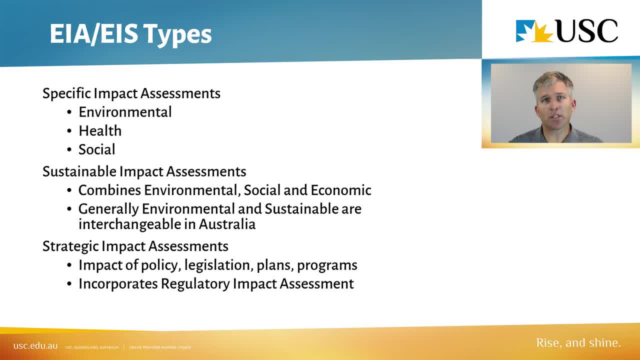 the tangible thing that you get at the end of the process that you put your hands on. But there are several types of an EIS or impact assessment, And we'll go through those briefly. So the specific environmental impact assessments, and they will come in. 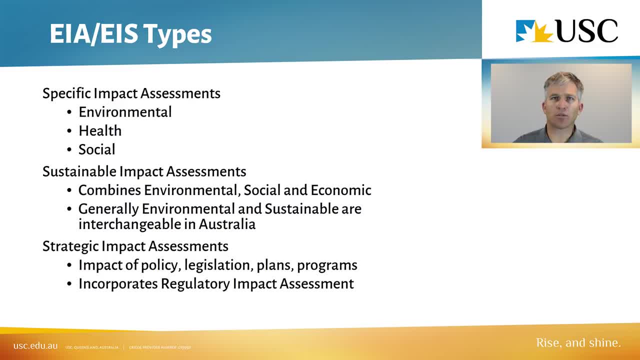 from a really pointed point of view And they'll look at certain specific criteria, as opposed to sustainable impact assessments, which are generally the ones that I've had involvement with, because they look at a broad spectrum of environmental aspects. If we want to go back to the term from now, 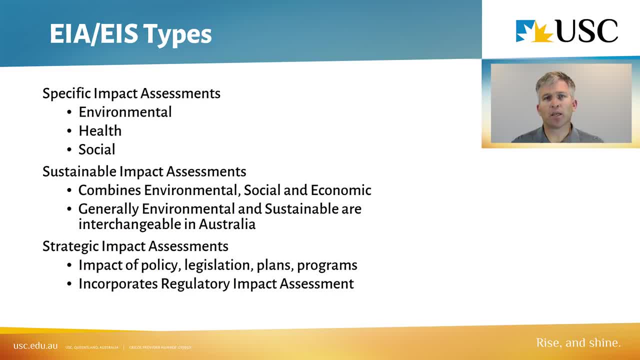 EMS and environmental aspect, so they cover that broad range of different things and to identify all of those impacts and values. And the third one is the strategic impact assessments, where they're looking more at your policy, legislation and sort of the higher level things. 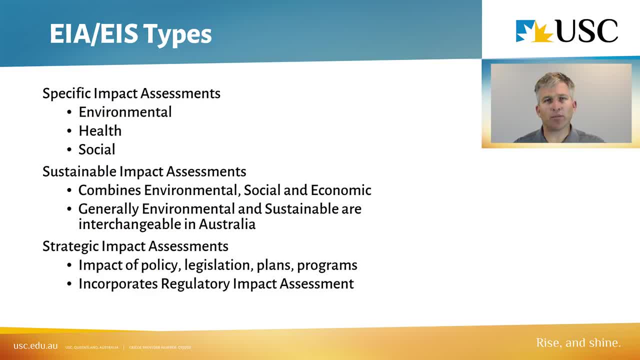 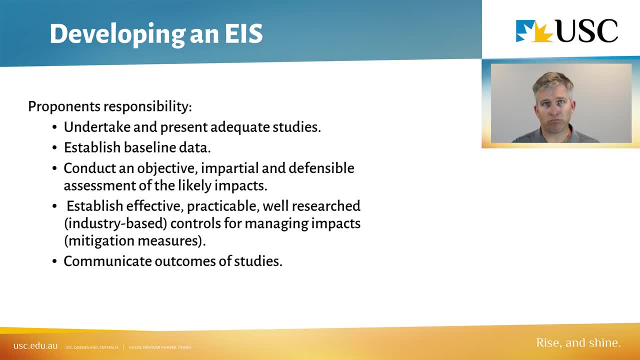 or a regulatory process. I haven't been involved in those. In developing an EIS, the proponent's got a responsibility to really have a few things and have a few undertakings And we'll run through those briefly. They must make sure they go through. 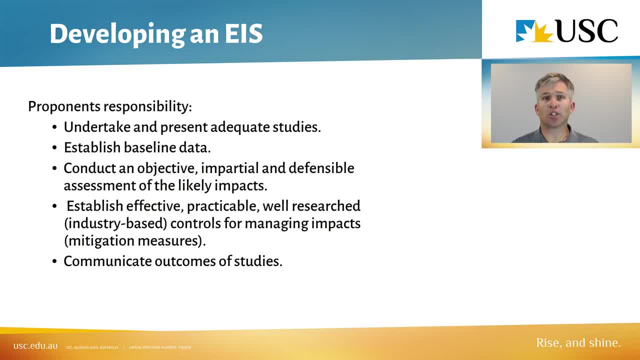 and present adequate studies. It's a communication process. They're presenting those studies forward for assessment And with the expectation that you want to be as comprehensive as you can, but you don't want to be arrogant in that and think we've covered everything. 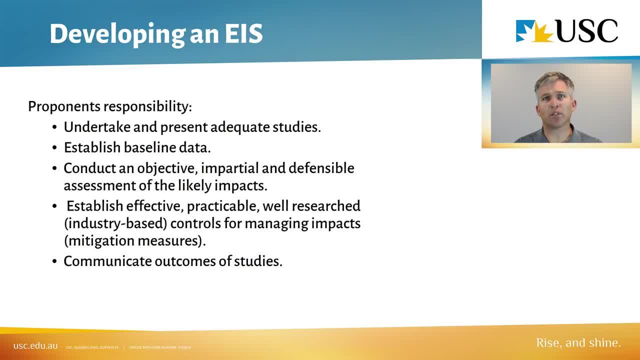 because there's often. there can easily be things that you haven't covered- or your experts- You know you've got your flora expert and your soils expert and everyone else, So they, for whatever reason, may miss something out. So you want. 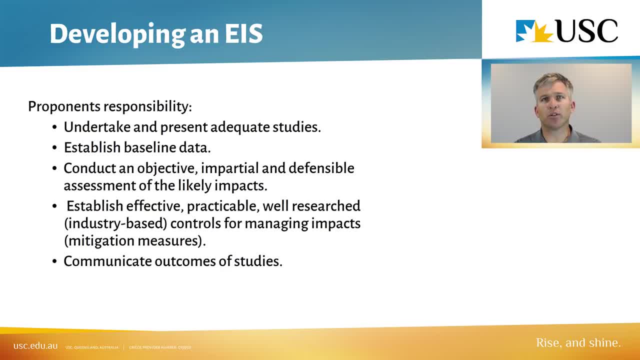 that goes to the public consultation process. to come back to make sure that all bases are covered to mitigate that risk. In doing that, you want to make sure you've established an adequate and a very detailed baseline data set, and they're your values, So you've gone out. 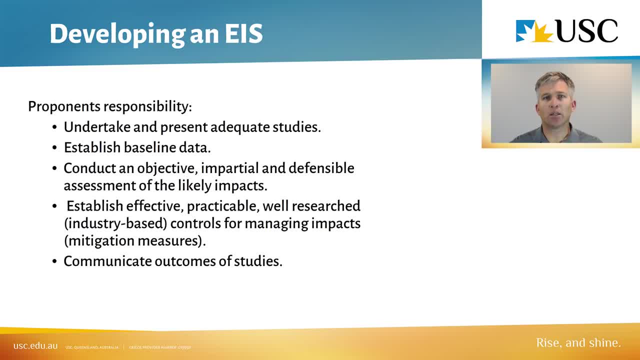 you've really been able to identify what's there before you start. Then to be able to conduct that really objective, impartial and ultimately, a defensible assessment of those likely impacts, To be as comprehensive as you can in that impact assessment process is absolutely imperative. 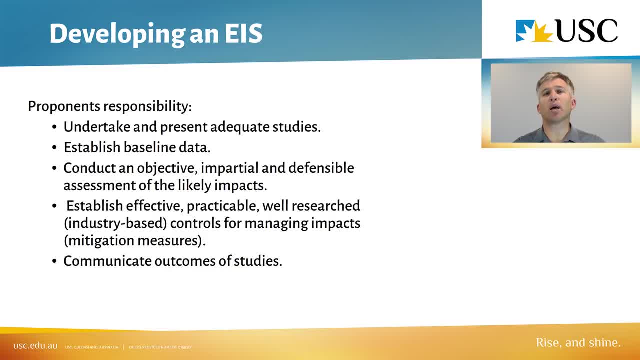 because if you don't do that, you're not going to be able to come up with that last point. And that last point is your mitigation measures or your management measures, whatever you want to call them, And to make sure that they're effective. 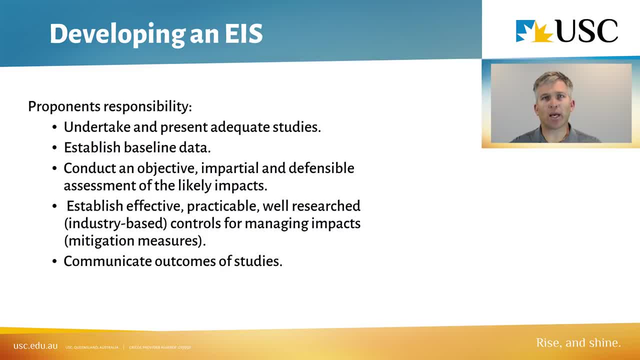 practical and well-researched. There's industry-based principles, applications, processes, skills, different things. It's important for several reasons to come up with a really accurate representative of what your mitigation measures are going to be, because if you go and promise the world, 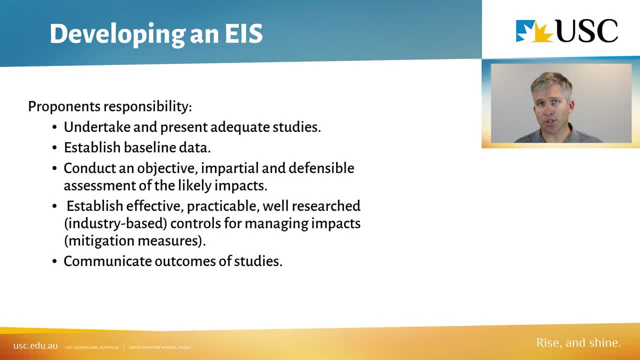 and commit all these things that you physically can't do, then you're going to be held accountable to that. People are going to expect that. and your bulldozers and excavators and trucks? they're not as fine as a toothbrush. They're only capable of so many things. 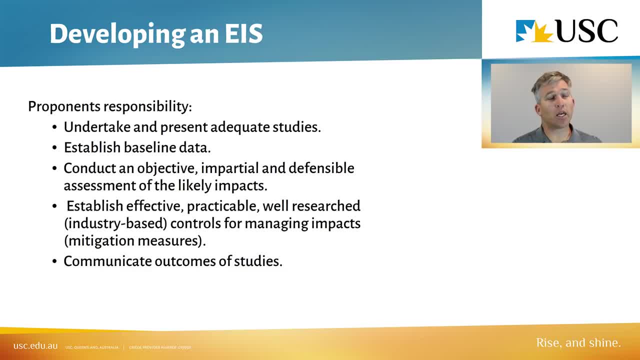 So you need to be very realistic in what you promise to say, okay, I've got a big machine, It can deliver this result. At the same time, you don't want to be sort of going through and insufficiently mitigating those impacts. 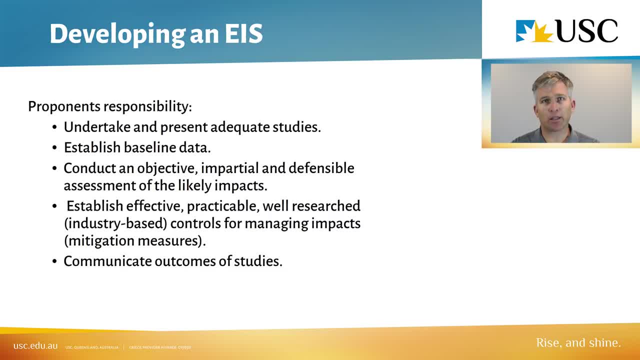 so that you end up having far worse impact than you actually assessed you may in the first place. So you sort of you know it's the old analysis- I think I've used it before- of galvanising something, not gold-plating it. 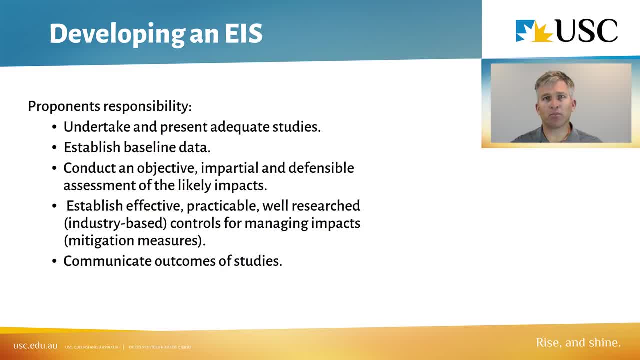 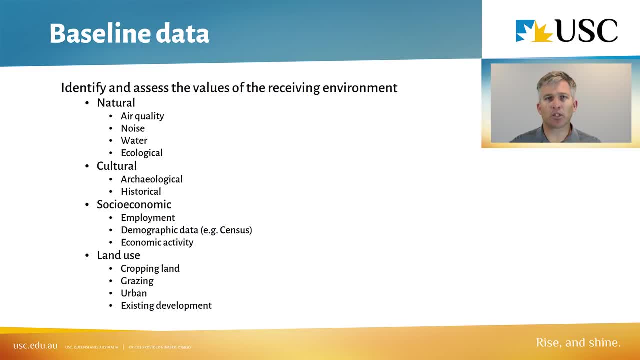 getting it fit for use, fit for purpose, but not going over the top or underbaking it as well. Looking at it in a little bit more detail now, we'll break down those couple of components from the previous slide. We'll start with baseline data. 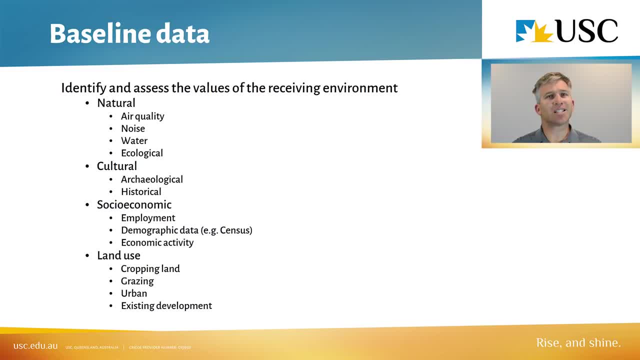 And in there we're going to go through and identify and assess those values of the receiving environment, Those the natural, the cultural, the socio-economic and those land use values that are there. You'll have a team that goes out. 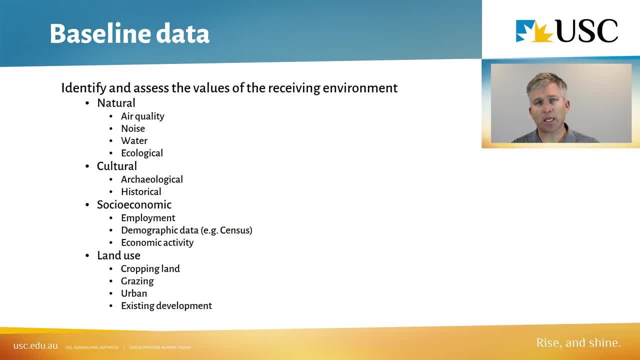 specialists in each of those areas and then a specialist again within those areas. They'll go out there and they'll be acquiring data, desktop data, on the ground survey assessments. In some of them you might be conducting modelling programmes. 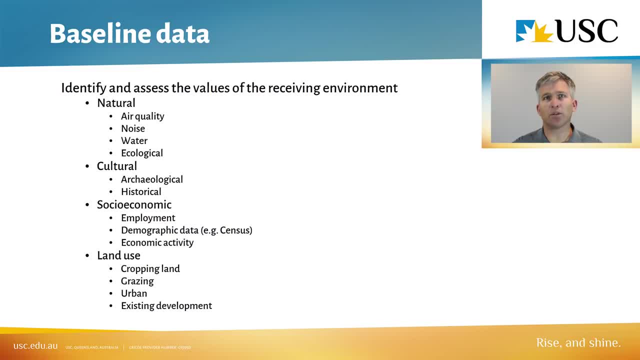 to establish hydrological flows or movements of certain ecological things, noise modelling, all of those sorts of things. So there's a lot of data that can be acquired through this process and you want to be out there getting as much of that data, and as much of that data accurately, as you can. 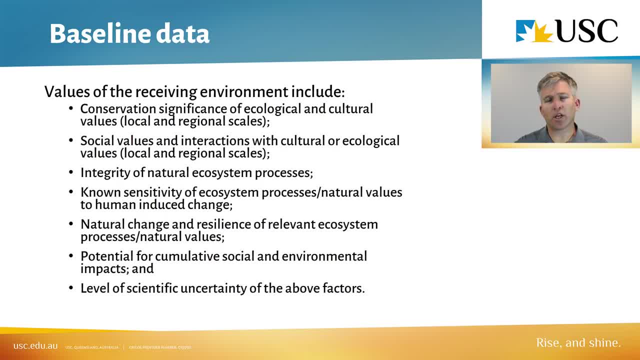 After you've gone through and identified those four main values within that ecosystem, you're going to assess them individually from a whole different points of view, looking at their conservation significance, be it the water sort of. look at the conservation significance of that water and the values there. 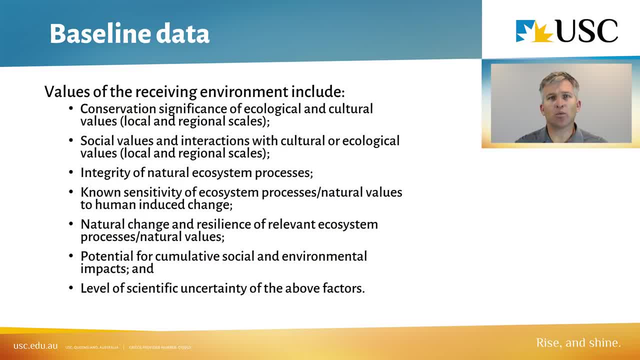 on a local and a regional scale. What impacts does it have? We're looking at the social values and, I suppose, the interactions of your project with the cultural or ecological values there are. again on that local and that regional scale You're going to go about looking at, assessing. 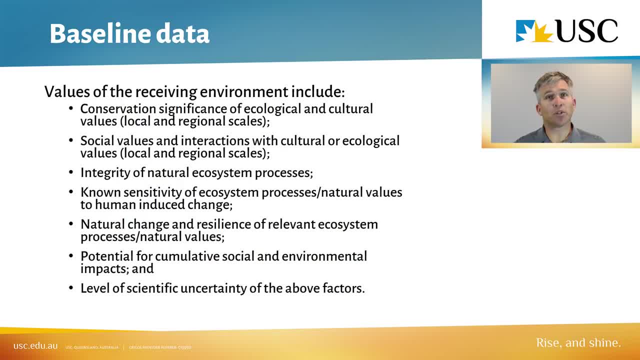 the integrity of that natural ecosystem and the processes to see how intact is it. Are you in fact going to be going across an already cleared area that's already been previously disturbed, or is it undisturbed And you're going through and smashing it down? 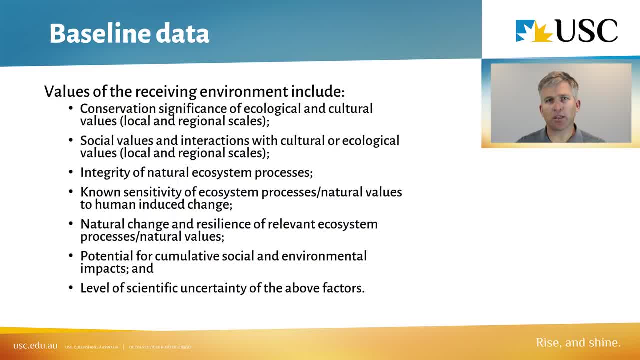 and causing some sort of impacting it in that way. So you're going to look at the integrity of that natural ecosystem, Have a look at the known sensitivity, and I suppose it's sort of reflected a little bit in that last point as well. 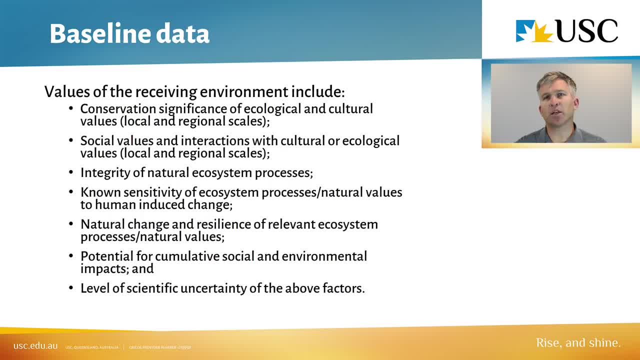 but the sensitivity of that ecosystem, natural values, to human-induced change. Okay, so what's gone on there in the past? How is it likely to respond to that change in there? Certain soils don't like disturbance. Certain animals struggle to recover after disturbance. 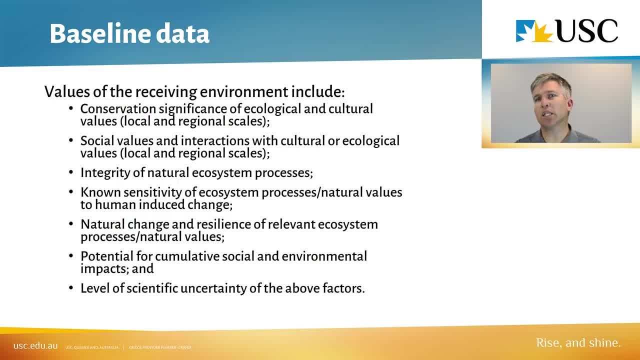 and all those sorts of things, And you're looking at the natural change and resilience of relevant ecosystem processes. So again, it's the ability to be able to cope with that change. We're going to look at the potential for that cumulative. 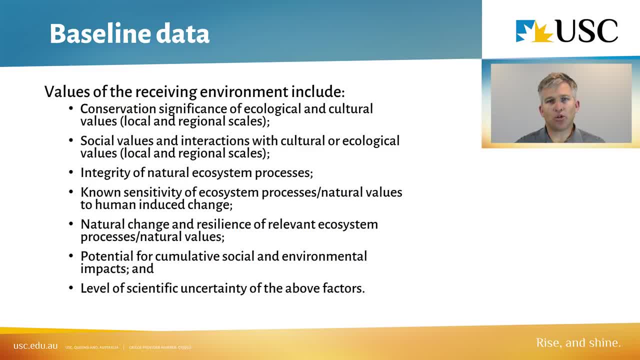 that social and environmental impact. So a cumulative assessment is a really difficult thing to do because if there are multiple projects going on within your area of disturbance, you need to be able to get together with those other proponents. You need to be able to pool. 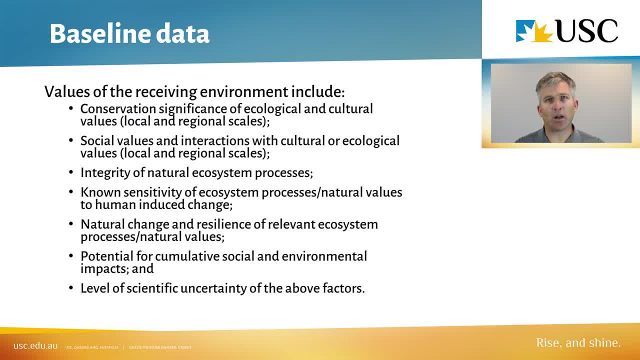 Hopefully you're all going on at the same time, but that's generally unlikely. But somehow there needs to be an assessment that goes on to look at that cumulative impact from all the other things that are going on within that area. And then I suppose 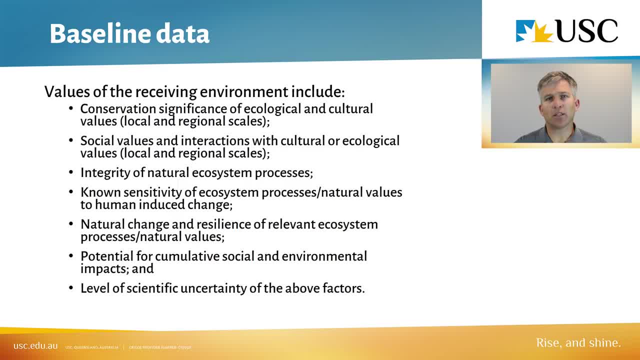 like any good statistician would do. you've got to look at, then, the level of uncertainty with those assessments that you've made, What's the likelihood of those assessments, etc. So there's a lot of things to take into consideration, and that's why you have a big team. 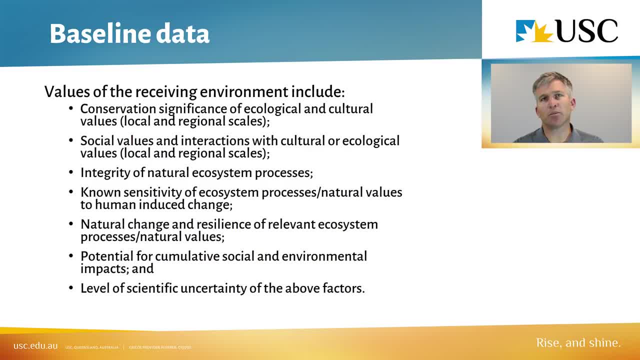 that pulls together and puts all this information in together. But they're some of the points that you need to be able to take into consideration Now, before I move on to the next couple of points. also, there is a generic terms of reference. Now, I haven't touched on the terms of reference as yet. 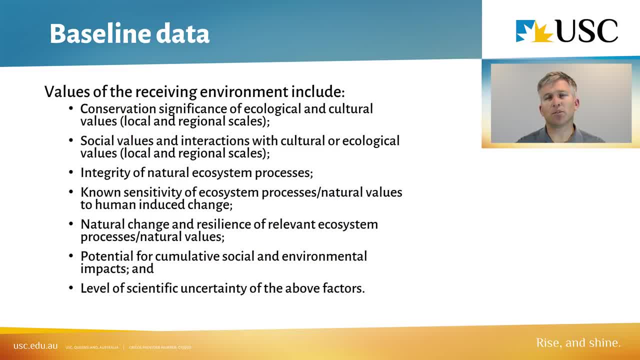 but we will. The generic terms of reference there gives you a very detailed list of the different values and the different types of assessments that you need to be looking at and doing, And we'll do that. we'll look at that in detail when we come to the assessment. 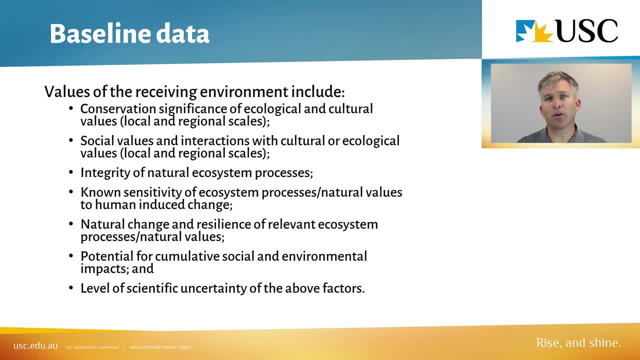 So look forward to that, and I'll direct you to that later on, But just to give you a bit of a heads up, all of these different things- like when you come to putting an EIS together, the government will issue a terms of reference. 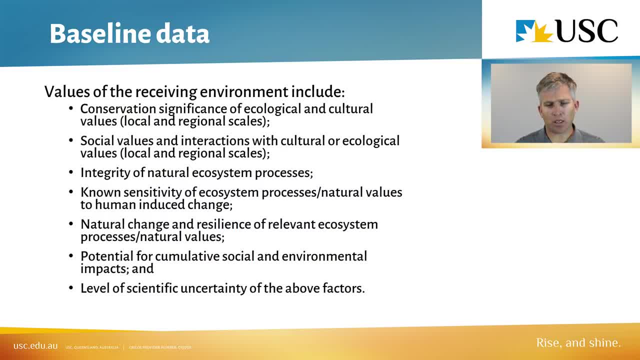 and for that project specifically, which very it spear points you to exactly the points that you need to take into consideration in doing that EIS And you'll go about doing that and within there you'll have to deal with these different points that we've just discussed there. 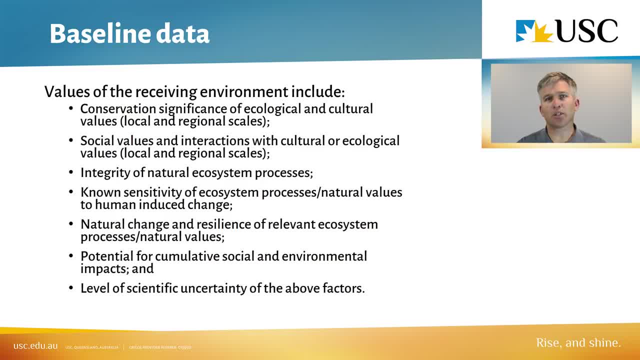 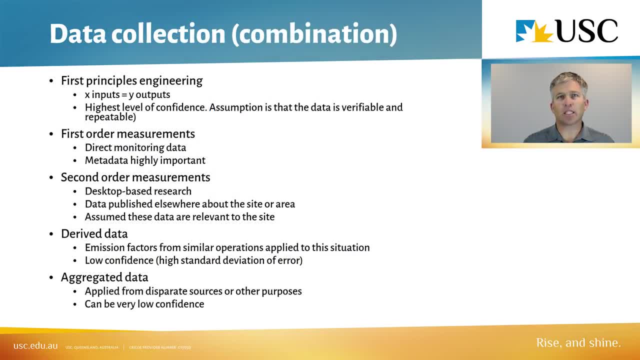 that conservation significance and the social values, the integrity, the non-sensitivity, etc. I want to look now at data collection and how we use that and the different levels of surety that we have for our methods of data collection. There are five different levels. 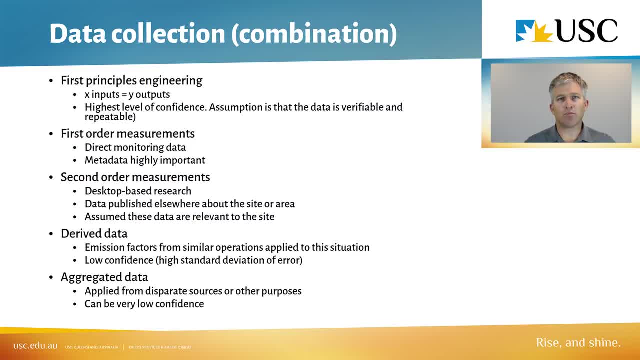 that I want to look at, and the first one we'll touch on, gives you the most repeatable, most verifiable, most accurate data that you can use, down to the least. And so the first one there is called First Principles Engineering. That process, 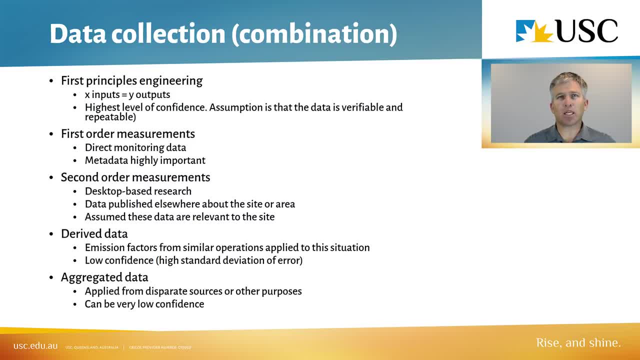 it's as you can. the name indicates it's a process of you've got X inputs going in, you've got Y inputs coming out. It's like X plus Y equals Z. Therefore, it's a very logical process and an example for this. 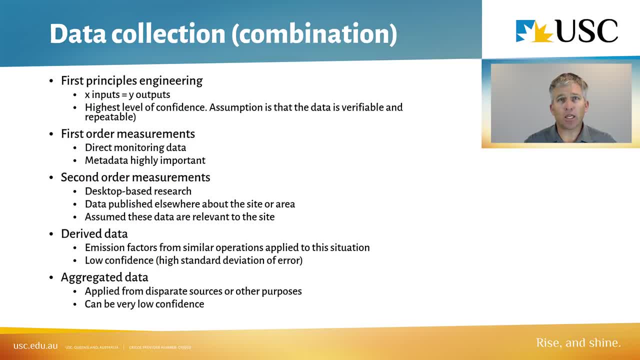 may be being able to as a design engineer or that sort of a person, will be able to go through and calculate. if there's this sort of example of thing going on on site, then this will give you this result. The second level that we'll look at there. 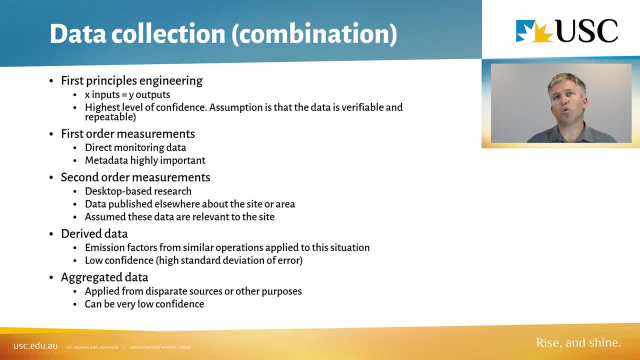 and it's sort of a bit confusing now but a First Order Measurement. First Order Measurement is looking now more at your monitoring data that's been collected from that site. So you've gone onto site, you've gone and done a flora, a botanical search or a fauna. 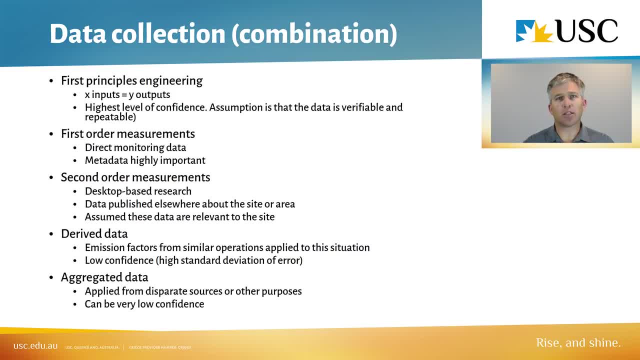 some transects and gone out and actually collected data And that's the metadata associated with. that is very important and you can pull that together and you can use that information. still, It's very accurate. You've been there, you've seen it. 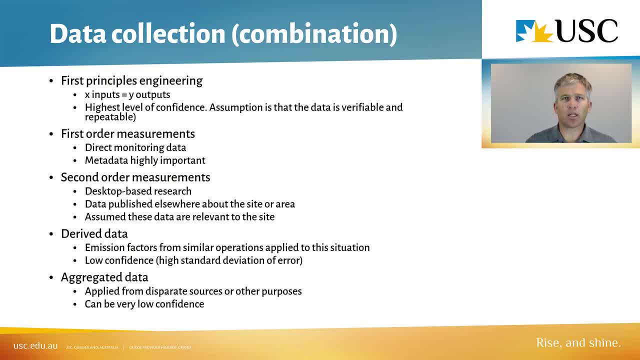 and you've collected that data That go onto the next level now, which is going down a little bit later. but less reliable is that Second Order Measurement, That's more base-top research, where you're using data that's published in other documents. 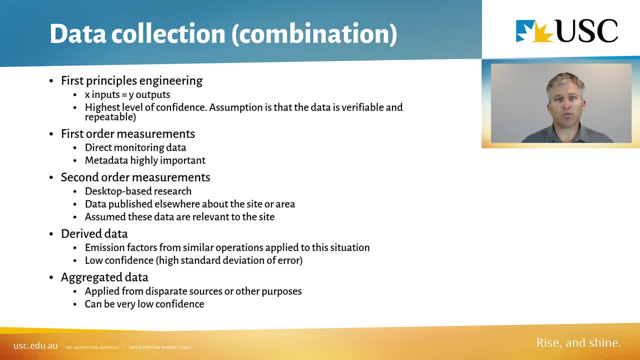 that's something about the site or the area. So it's still fairly reliable and you can assume that this is going to be accurate, that the author who wrote it was correct, but we're getting down to a lesser level of certainty with that data. 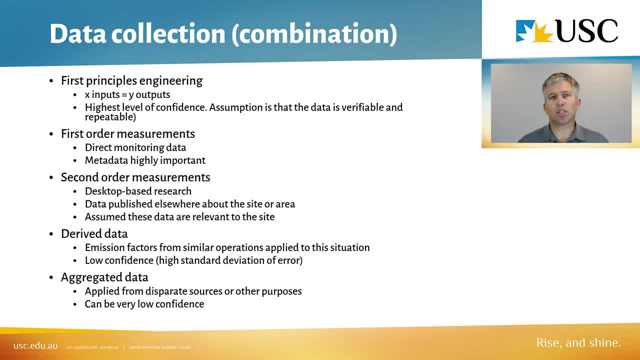 The next level is looking at the derived data, And this is data that it's going to be, data that's applied to a similar situation, where you might look at that data, that desktop data that is in a similar environment. Therefore, we should get the same results. 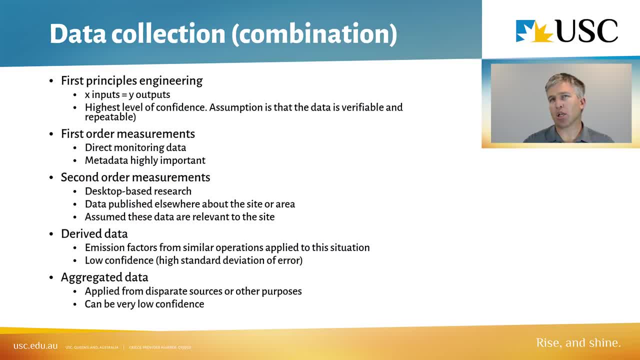 the same things going on here. It's a much lower level of confidence as opposed to say previously, where we were looking at documents that were developed for that site by someone else And that bottom level is aggregated data and that's sort of applying. that's sort of a far more assumption. 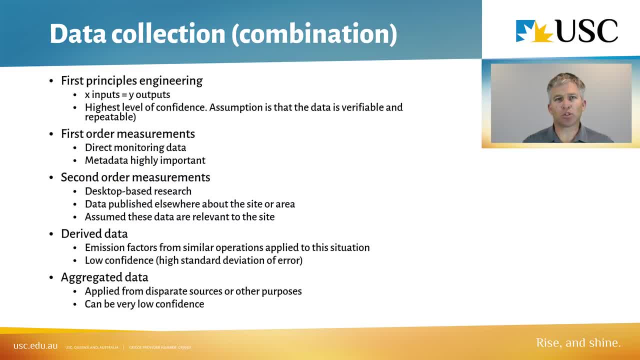 in that process and you're pulling data from other sources and making assumptions, So you have a much lower level of confidence there. But so you've got those five, I suppose, levels of data that you can use, and it's important to use them all. 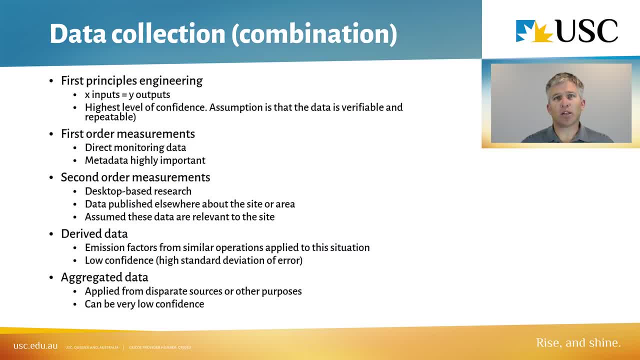 or as many as you can, Combine them all and draw them in to come up with the most comprehensive, I suppose, amount of data or data set that you can use for that site And some of the less accurate stuff. you're going to then go about verifying that further. 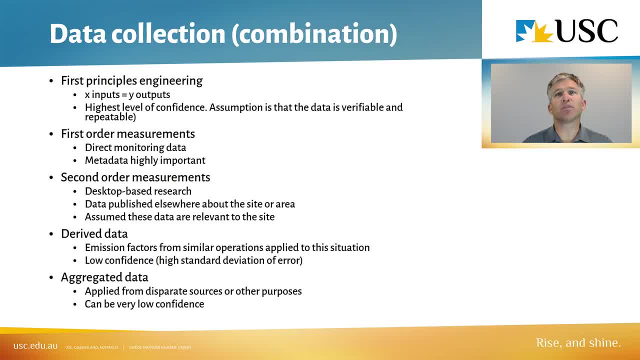 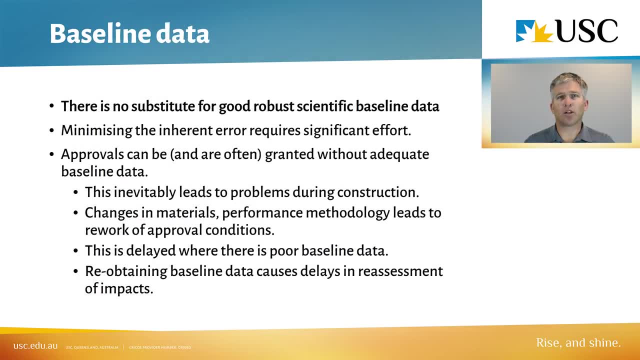 later on down the track, hopefully with some first order measurement stuff going on a site doing a few more samples or chasing things up later on down the track. Now there's no substitute for good, robust, scientific baseline data. You want to go out and get the most comprehensive data. 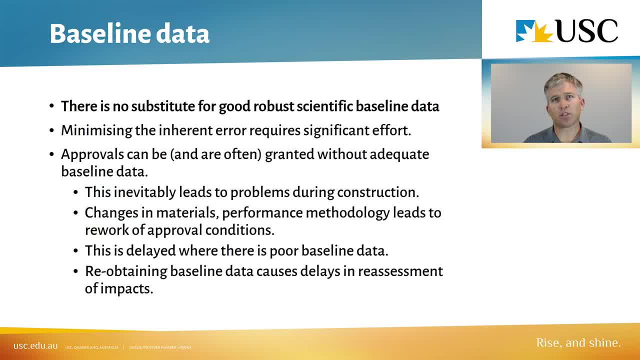 set that you can, because it'll streamline the process and make it so much easier later on down the track. There are multiple reasons for this and we'll go through a couple. However, trying to do this requires a significant amount of effort- trying to get all this data. 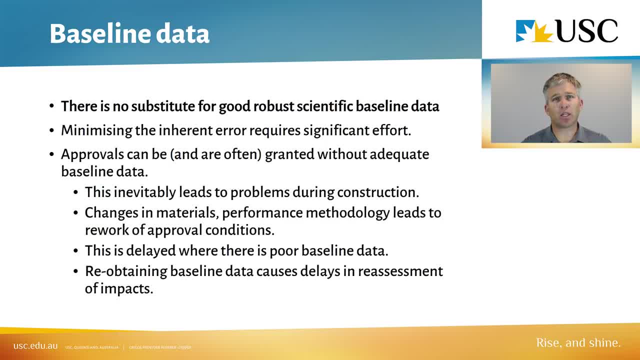 And in that process you want to be minimizing that inherent error that may be within that data. set Down the track. we'll look at some better, some pros and cons, But you know, look, approvals can be, and are, often. 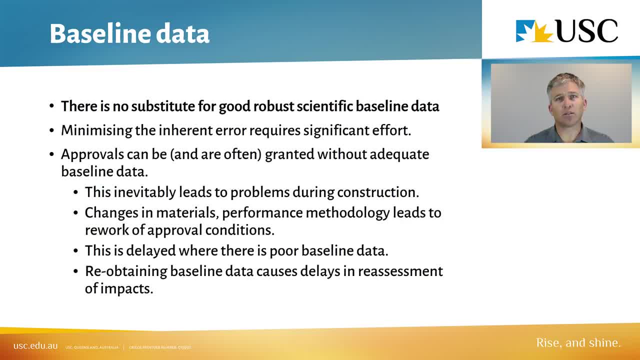 I've come across this on many projects where approvals are granted without that full, adequate baseline data and it leads to problems. it leads to a lot of problems And these can include, like within construction, If you're going ahead with construction and in that process. 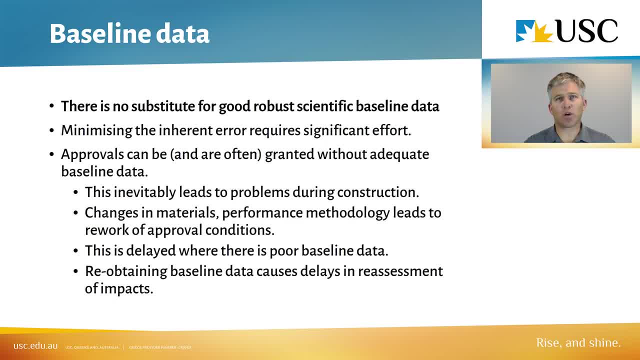 and you don't have that full data set, you can get all sorts of surprises. We've had rare and threatened and endangered species occurring on the project area and all of a sudden you have to stop the doses, You have to pull up and go around. 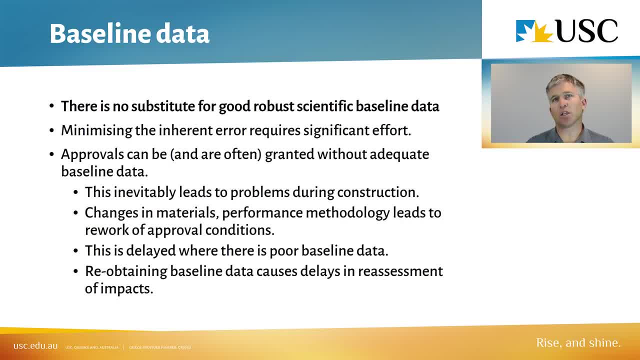 acquire approvals. It causes a lot of delays. It's a costly process, Likewise from a cultural heritage point of view. as difficult as it is to get that full, comprehensive data set of data. we've had to move sites, move projects significantly there. 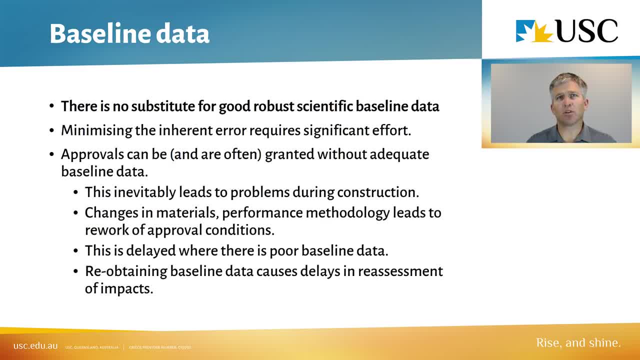 One example that really comes to mind is when I was doing a slurry pipeline from the Century Zinc Pazminco, Century Zinc up in the Gulf, running across to Kurumba, And we came to one waterway, a smaller waterway. 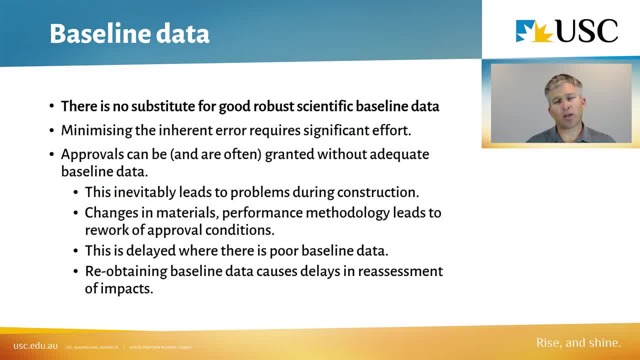 not one of the big rivers up there but a smaller waterway. And as we went down through the bank, cut through the shoulder of a warrior, an Aboriginal warrior, ancient warrior, had been buried in the bank of the creek there, obviously years and years and years ago. 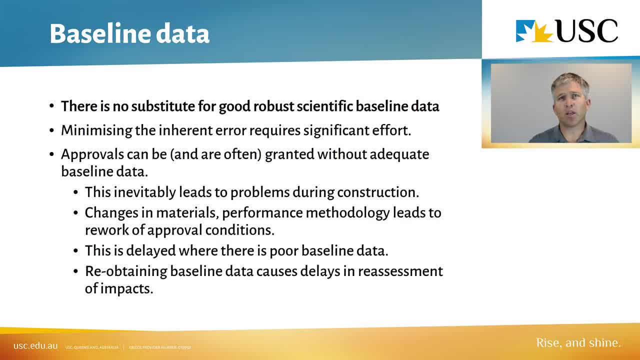 But his spear and his shield and that sort of thing were in there with him And we had to go back and re-divert that line. No one wants to go and dig up a grave or anything. I'd say, yeah, we had to go and re-divert that line. 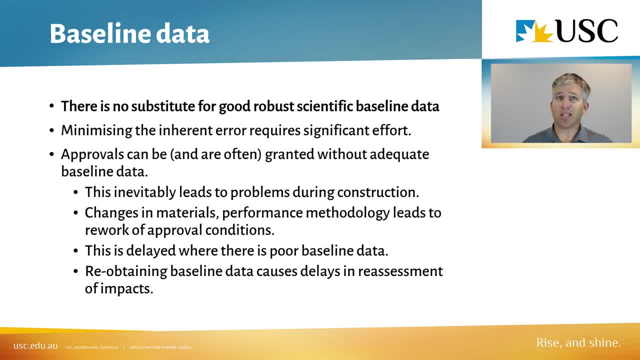 And that's an example. It's really hard to get that full, comprehensive data. There was no way of us telling that the grave was there unless we'd gone and done core samples every few 10 centimetres. But you want to try and get as comprehensive. 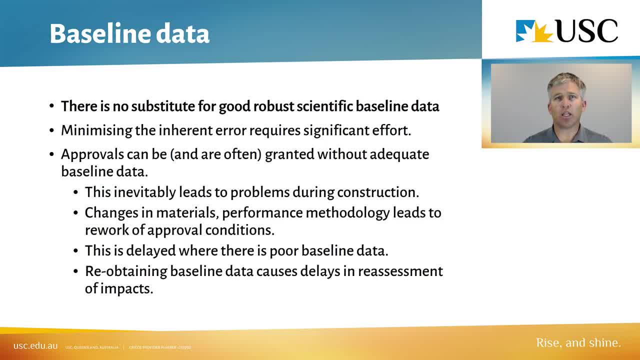 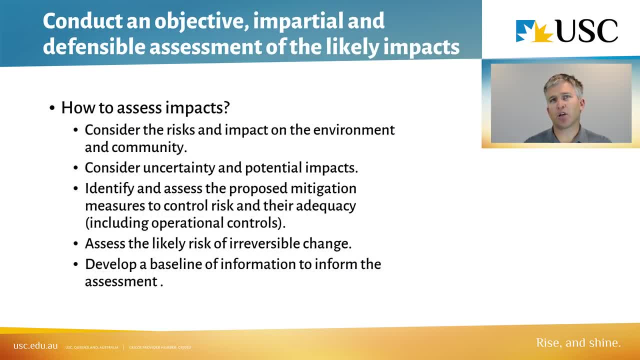 as a comprehensive data set as you possibly can within your baseline data collection. Now looking at how to go about assessing your likely impacts that you've got on that project. First of all, if you remember, back to the EMS module of this course, 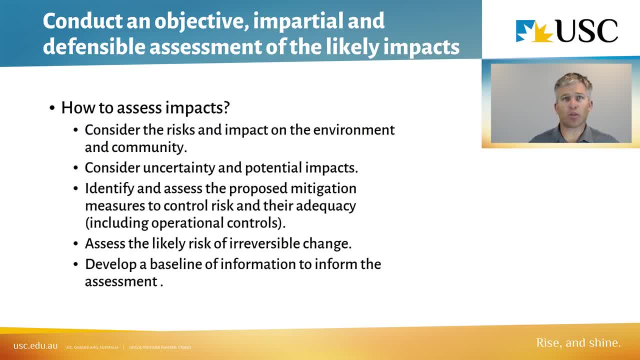 we did our risk assessment And we went through and we did an assessment of, well, initially the likelihood. There was the likelihood band that ran down. So considering uncertainty, certainty whether certain potential things are going to occur. Then we did the consequence. 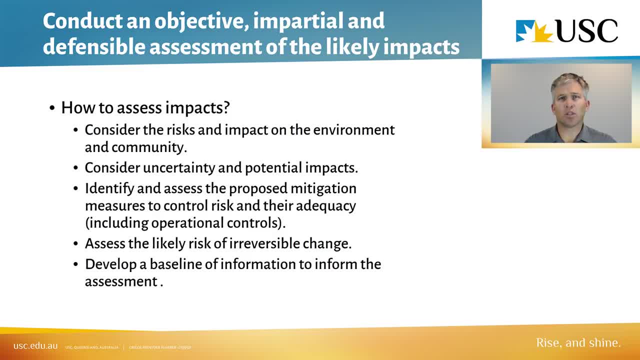 or the severity of those things, You know what sort of impact or what's the risks and the impact on the environment and the community, And then looking at the mitigation measures. So you're familiar with that process You go through and now we're looking at those mitigation measures. 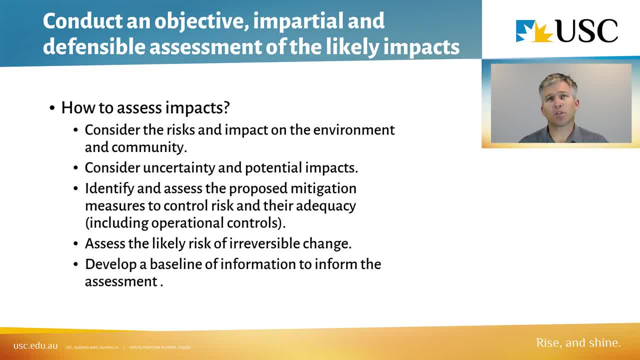 to see whether you know whether they are going to control the risk in the way that we want it to do, that, whether it's going to be adequate or not. So then, we're almost moving through to the next phase of looking at residual risk. 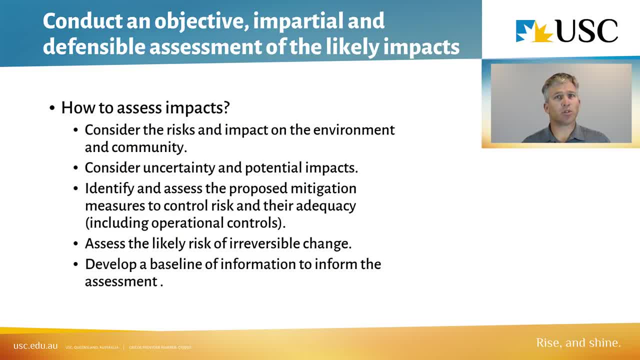 that's going to be left over, And is that acceptable to the project? Or, more likely, is that acceptable to the stakeholders and to the regulators in their assessment? Okay, We then also need to be looking at, you know, is there irreversible change? 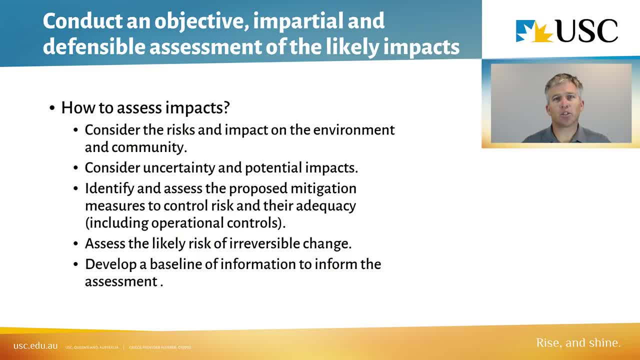 and what's the likely risk of that irreversible change, And is that acceptable? And so you know, we're developing a baseline assessment of all of this sort of information, pooling it all together and delivering that in one concise document, hopefully with some very clear 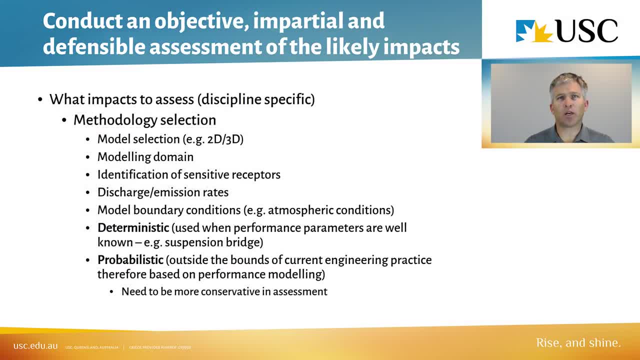 and informative outcomes. Okay, We're going to look at what impacts to assess and how to go about that. First of all, we'll look at the methodology selection. Now, this is massive in looking at the methodology, looking at the project and the likely impacts that can come from that. 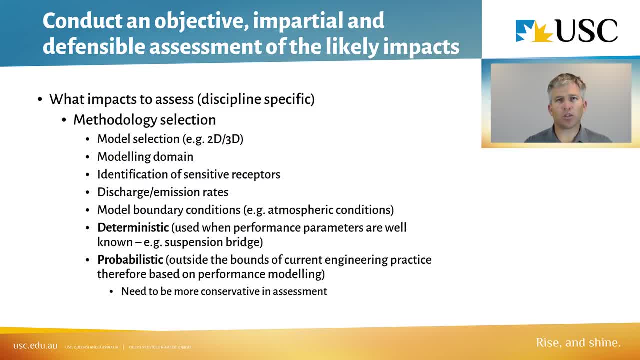 And there's a lot of different ways of going about doing this. It can involve a lot of modelling, be it 2D, 3D. It can go through looking at. you have to identify sensitive receptors, be it along the line. 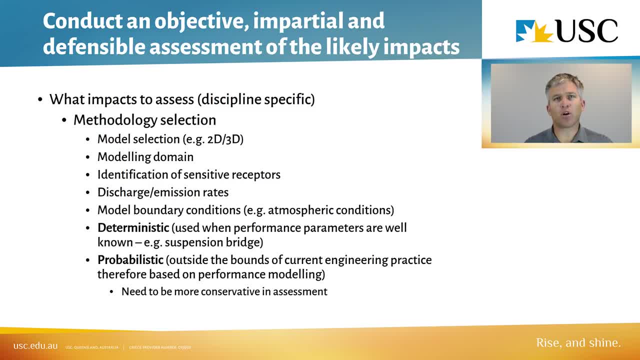 whether they're community or whether they're sort of environmental. You know we're looking at from the project's point of view what rates of discharge, emission and impact and what sort of things could be you could be impacting upon the environment. There's heaps. 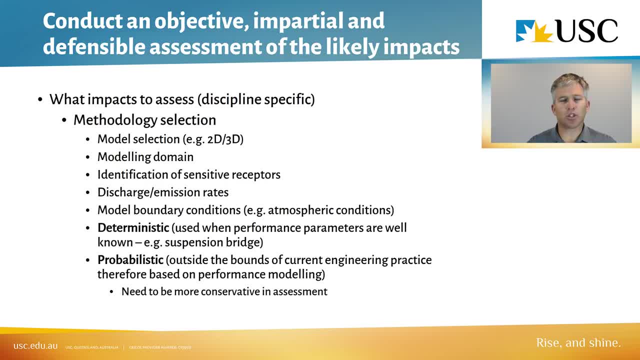 and there's two different main types within there. There's the deterministic methods which you can use in there And that's looking at things which are far more, I suppose, engineered, And you can go through there and calculate things. You've worked them out before on past. 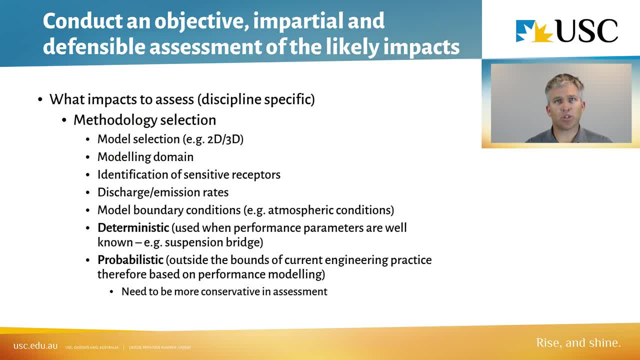 So, for example, a suspension bridge you can engineer, that You can go through and apply your mathematical models and come up with an answer as to those what outcomes you might have, as opposed to probabilistic, which are more on performance modelling. 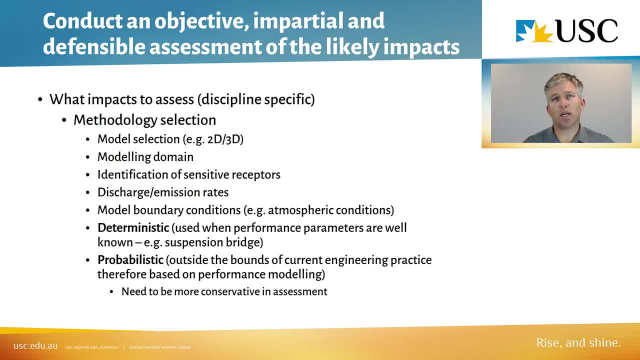 And you put in. you sort of have to build that model and think, okay, well, we can assume that this might happen. and assume that happened, run that model and then see what sort of outcomes can come of that. And I suppose an example of that. 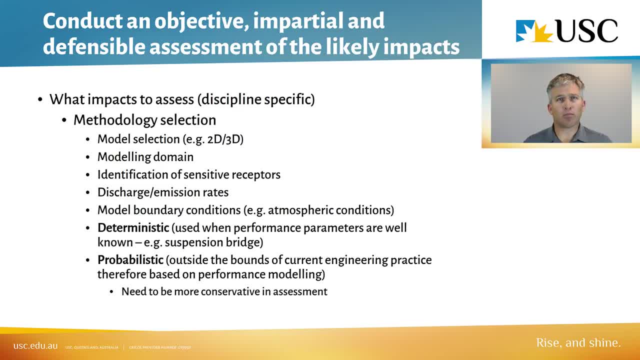 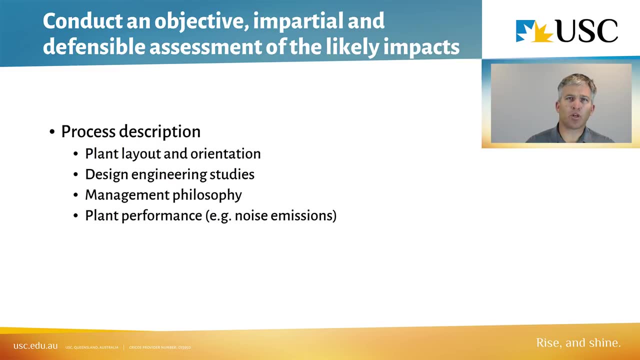 is probably more within weather, and be it climate modelling, that sort of a thing of going ahead, and there's there's so many, so many variables within the weather, So these sorts of things are based on best guess. Okay, moving on from the modelling. 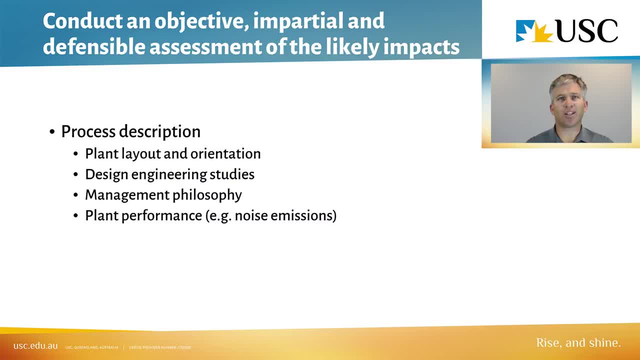 we're going to look at the process description and that's more, looking at your, say, your project description far more closely. You're working with the design engineers, you're working with your construction personnel, particularly within here, like the construction managers- a great resource. 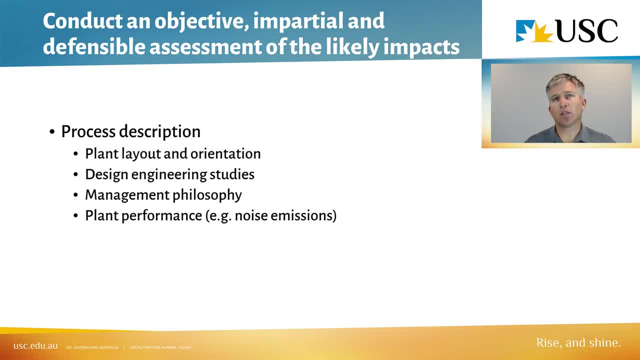 when you're going in and looking at impacts directly relating to your project, with how the how the project might be laid out, orientated, what sort of gear you might have there, what buildings, what machines, what structures, what different construction gear. 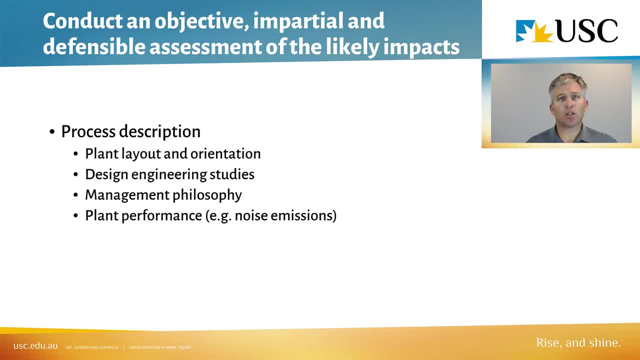 what engineering design and what studies, and you can do studies with regards to the different engineering designs and the impacts and what they might have on your environment management philosophy, the way in which your design, your management team can be structured, and you can look at the plant performance. 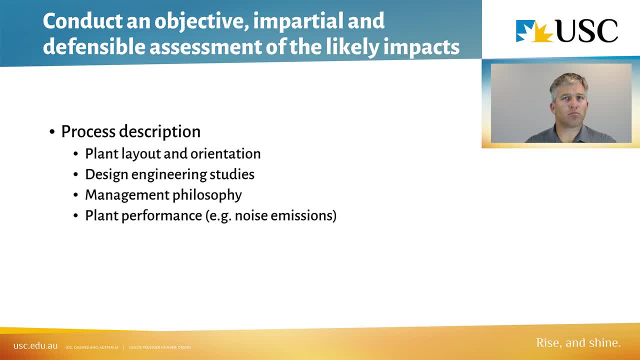 and with noise emissions and performance, vibration, modelling, all of those sorts of things come down into that sort of area. So this is very this area is very heavily the impacts are very heavily impacted by what machines you have got in site on site. 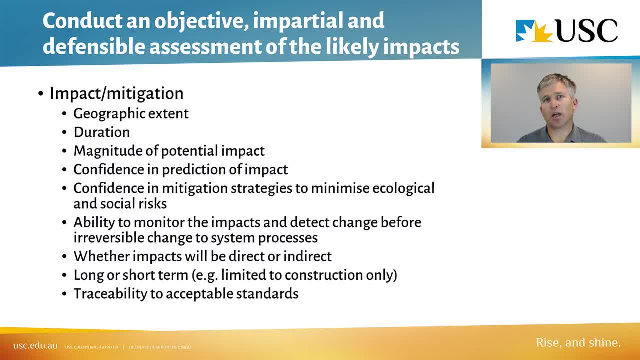 Now looking at your impact mitigation, there's a whole things, a whole heap of things, that we need to be taking into consideration here as well, And these include geographic extent- where you're going to be located, how long you're going to be located there for. 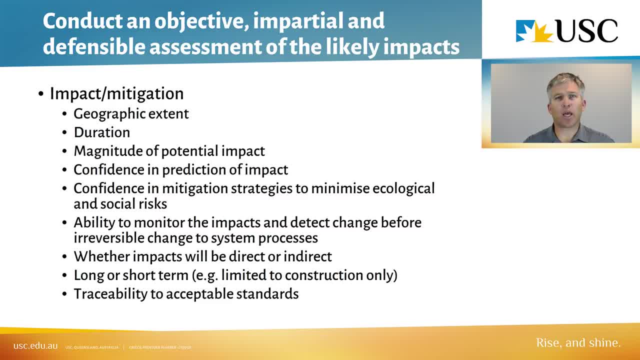 the size of the project. When looking at these impacts, you need to be looking at your, the surety of any, any assumptions that you've made, and your modelling and looking at so your confidence in those sorts of things, looking at those mitigation strategies. 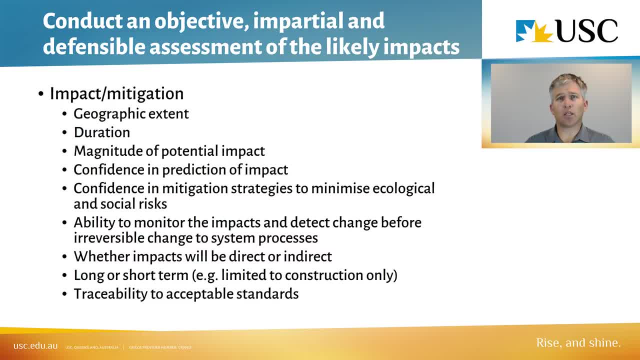 are they actually tried and true? Are you confident that they're going to be working and are they going to be effective and provide the results that you want? And are they practicable? Are they actually going to be implemented by the construction team? All of those sorts of things. 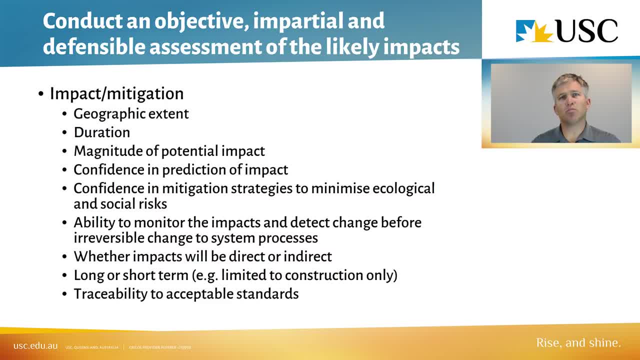 you need to be looking at your ability to be able to monitor these impacts, and it's no, no good if you've got some, some goals, but you also need some thresholds, KPIs. you don't want to go above this level. 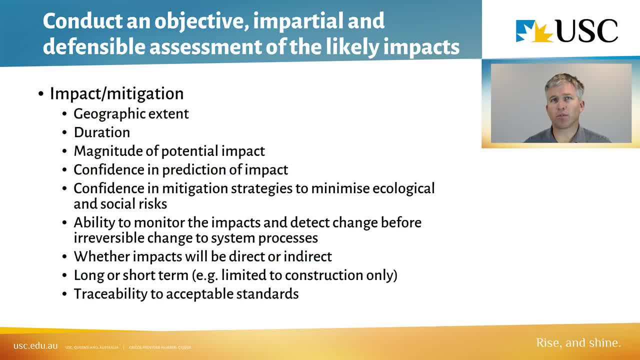 However, it's difficult to monitor and, oops, all of a sudden we've gone up and over that. You want to be able to be monitoring these things all the time. Oh look, direct and indirect impacts, all of the short, long-term impacts. 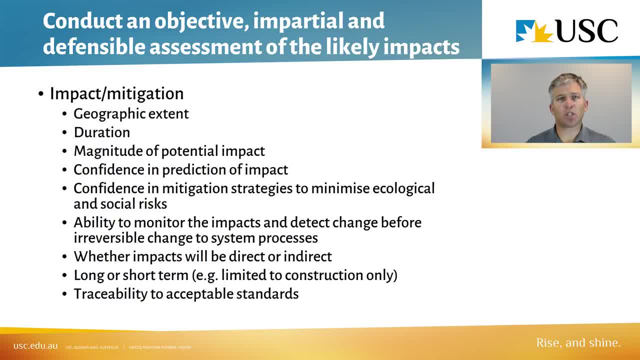 and there's a whole heap of different things which come into assessing the impacts and um that you are going to be imposing on the environment while you're there, But there's there's some examples of some things to be taking into consideration. 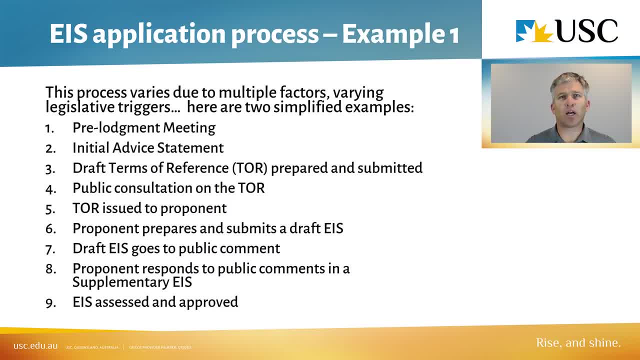 Okay now I know a lot have asked me just the other day about, uh, looking at the, that EIS application process and I thought I might just put that down and run that through. It's as I said the other day. 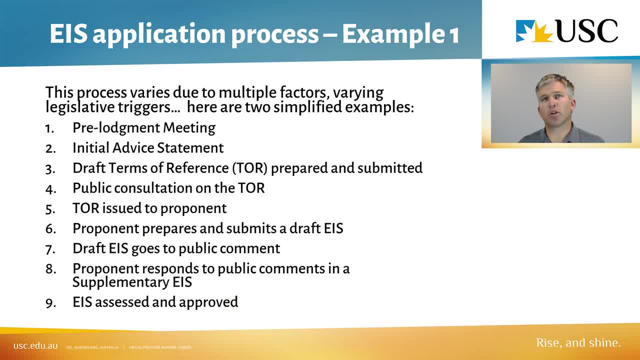 the. the actual process for an EIS to go from start to finish, I suppose, is very variable and impacted greatly by the, the legislation that that EIS triggers or that project triggers, and, and so there's varying levels um of legislation. 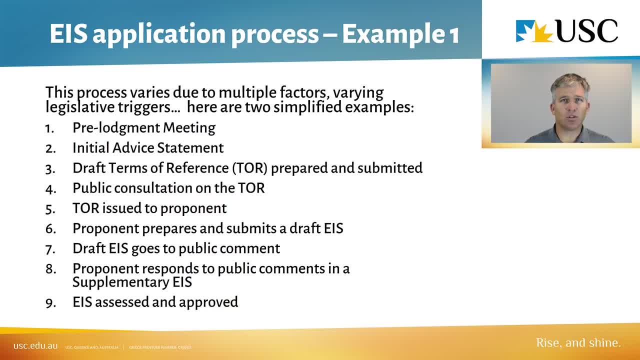 and and sort of regulatory processes that this thing could be going into may not. So I'm sort of guessing a little bit here, but I'm giving you, I'll give you a couple of examples. They're very simplified. Um, this one here: 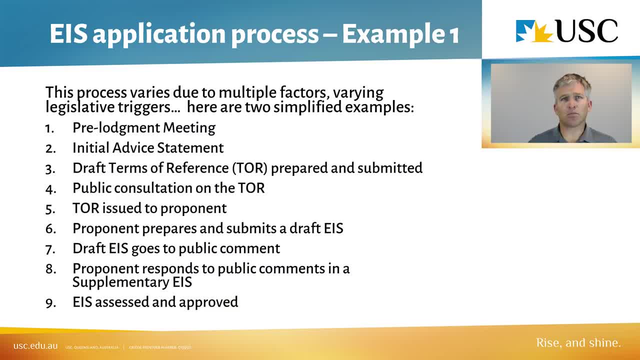 is going a little bit more from my experience on, on some probably like slightly smaller projects, whereas the second one will be slightly larger, um, which is like some of the more recent projects that I've been on Initially. yeah, there'd be a pre-logitment meeting. 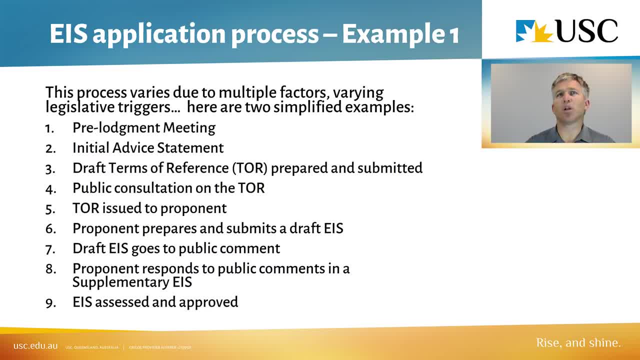 you'd go through, and that's just you. you can organise a pre-logitment meeting through with the government. You go in, you meet with them and you know you give pre-empt them and tell them that we want to meet about this. 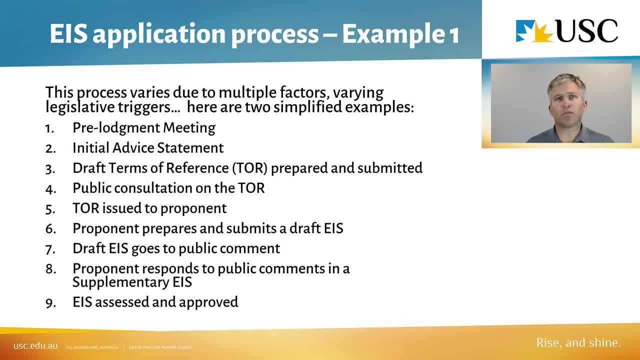 and um. you can go and have a talk with them about it. You might put in an initial advice statement, um, which is that initial advice? It's sort of telling the government what the project is, what it's going to be doing. 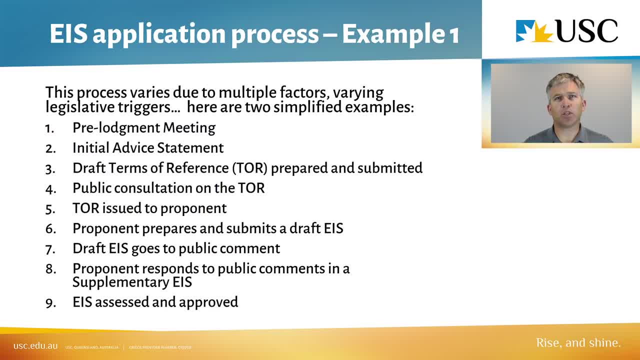 and you're trying to convince them that you're on top of this. You, you understand and you know the processes, you know the impacts, you can manage it. um, you're going to try and portray a strong level, um of competence. 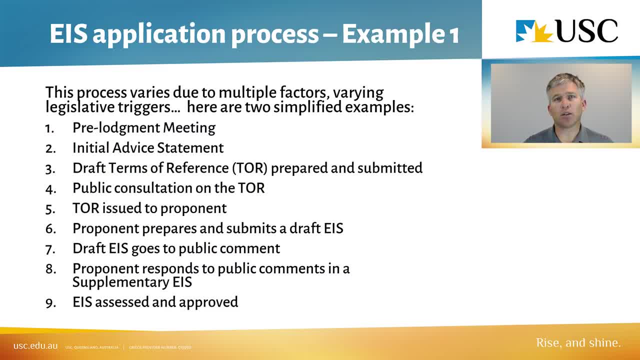 and try and win a lot of the government confidence. uh in in through that process, in developing this, this initial advice statement, or I IAS. Then you go through, some draft terms of reference will be prepared or a tour will be prepared. 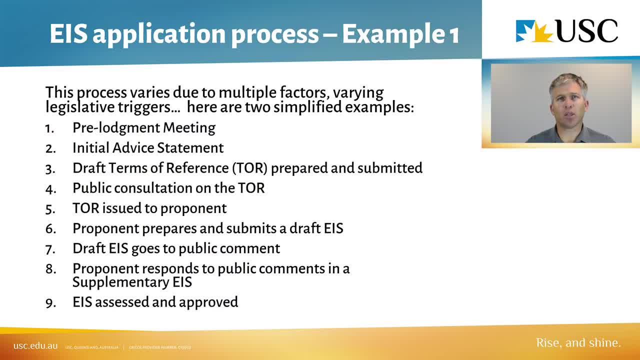 and submitted- Uh, I spoke a little bit about that, um, the other day as well. The a, a tour, generally would be uh, and historically would be put together by the proponent and submitted to the regulator, and the regulator would then go through a review process of that. 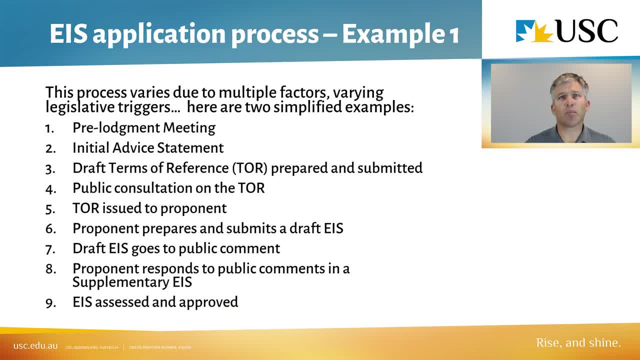 and may even go to um comment, public comment, and come back and and reissue that back. Uh, and then you would move on um and go through and go about the process of um or a draft EIS. 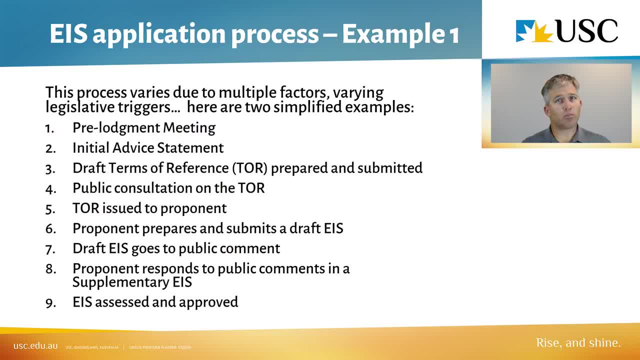 and that one then goes into the regulator and they, you can go to public comment, um, and then- and that's a a set defined timeframe- You go and present that to public groups, wait for the comments to come back, assess all of those comments. 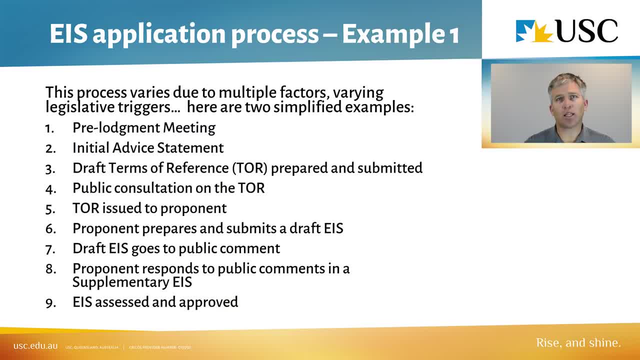 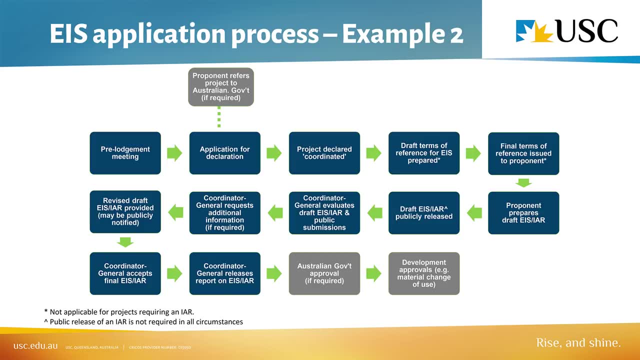 incorporate them into now a supplementary EIS and that EIS is then submitted back into the government and and goes through that assessment and hopefully is is finally approved. The second example I have uh for the EIS application process is uh. 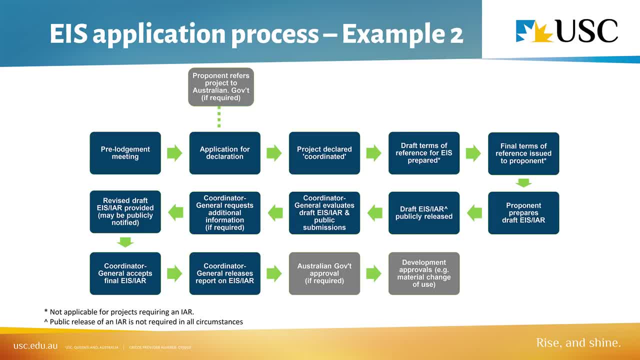 this flow chart that I've taken straight off the Department of State Development's website and it just it. it goes through. I'll run through, run you through that quickly, but I can't emphasise strongly enough for you to you know. 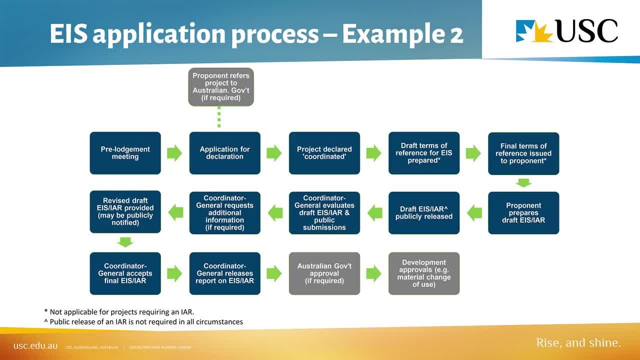 have how much. if you really want to understand this process, get on and have a look at on the Department of State Development, do a search for EIS application, um, all of those sorts of things, and and it'll send you straight there. 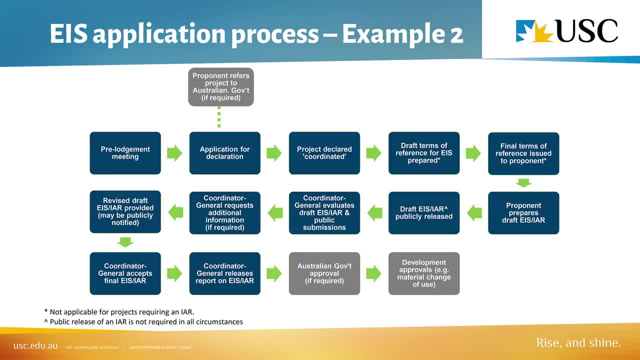 But this process, as mentioned before it's, it is very, it's very dependent on the different triggers that are hit through this um project development phase. But with your pre-lodgement meeting, uh, that you go in. 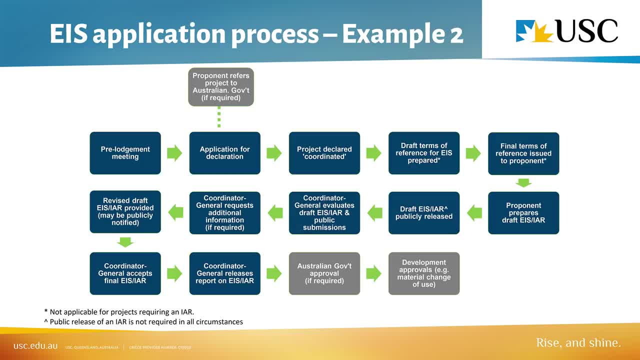 you're meeting with the, with the coordinator general and the and the Department of State Development, um, and you go through um, there may be some involvement from the Australian Government If, if required, it's no longer required um. 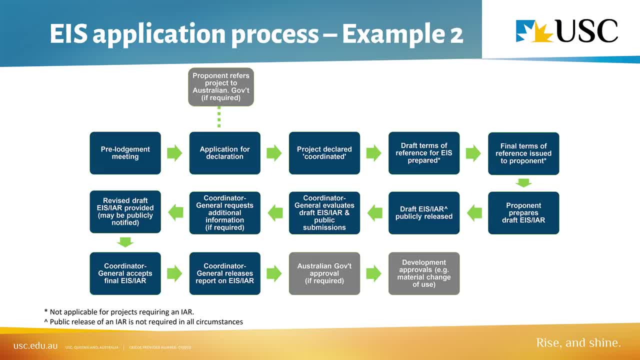 and then you go through this, this application process for declaration, um, and okay, so then it may be declared coordinated and and it goes through um and you prepare the, the terms of reference, The. the regulator will go and. 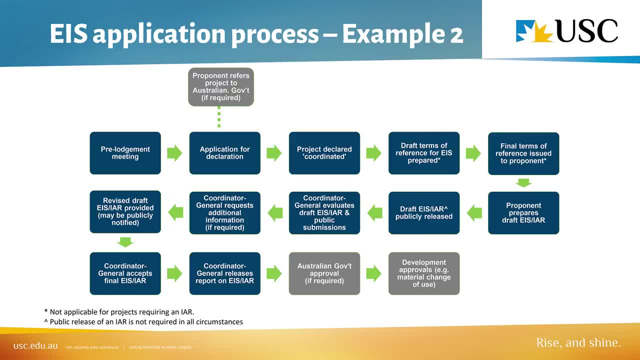 and request feedback from the public and from other uh internal agencies, and then they get issued to you. You go ahead and prepare your draft EIS That will go and be released publicly and and um, and then you'll receive comments back. 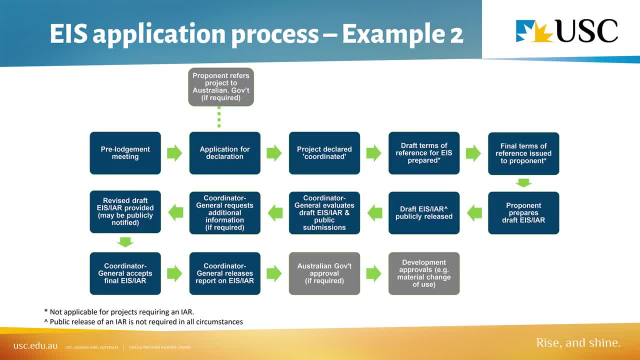 You can go and um formalise your responses to those public comments, um, and they go through, and the coordinator general is involved in moving this process uh through. as a as a facilitator, I, I suppose, is probably the best word for it. 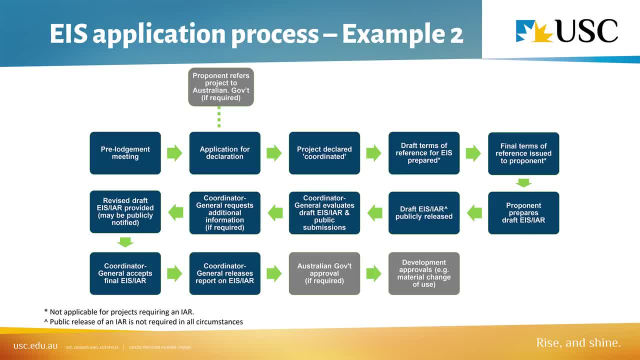 and, and then they move through and uh, you can read those things, you know it. then it goes through your final EIS, um awarded, and then they go away, and and you've got your approval. But in that process 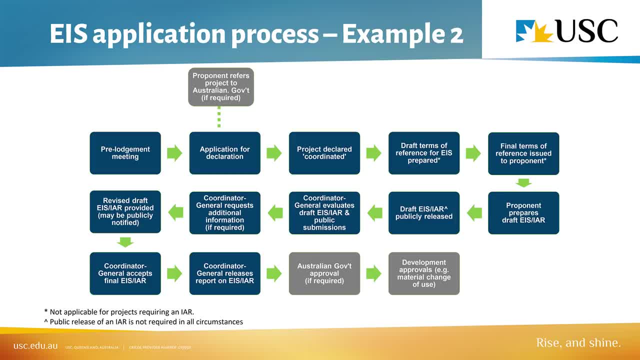 on this sort of level. you'll be issued a coordinator general's report, which will be an assessment on that, and you'll also get that EIS approval, and then there's all the other subsequent approvals that you need to go and get, Okay. So 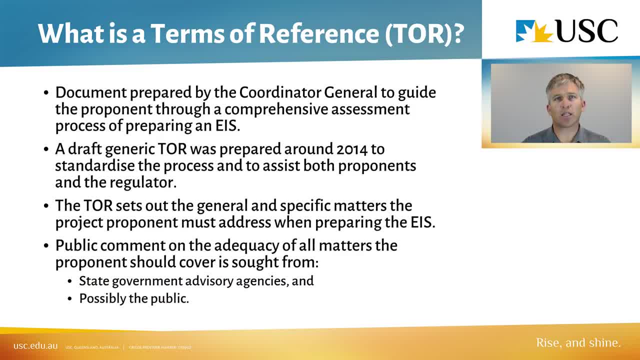 what is a terms of reference? Now, we we spoke about it briefly the other day when um in the class um, but I thought we'd just provide a little bit more information here and formalise that It it's a. 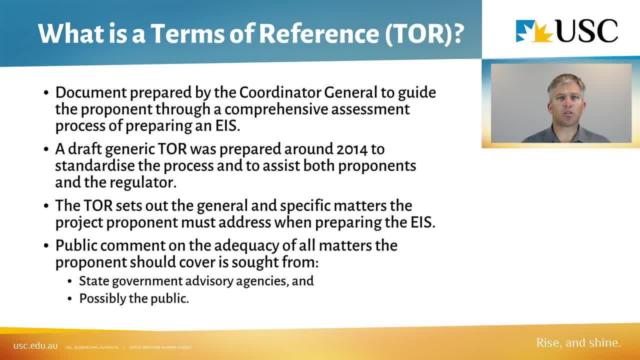 it's, it's put together and it it's something that, uh, traditionally was always put together by the proponent as a draft. Uh, formally, it should have been prepared by the regulator. However, if you were to provide that draft to the regulator, 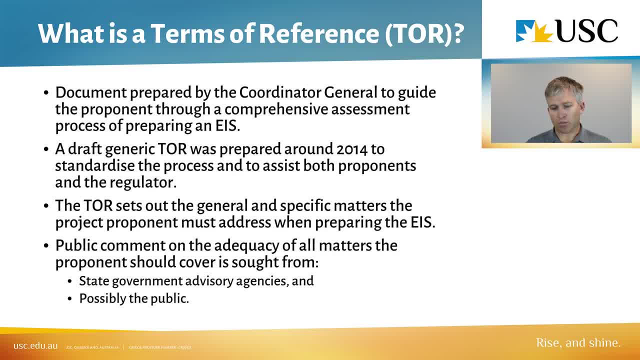 then, um, they didn't have to do as much thinking. They would simply be able to go through and and and come up with- uh, you know, and build upon the submission that you had put in, They might go to public comment. 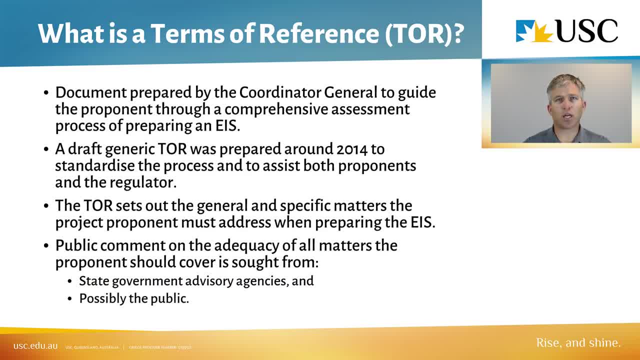 and take this, that information back and and build out a, a complete terms of reference. But the the issue back then, before there was a generic one, was that um, different proponents would come with varying levels of. I suppose. 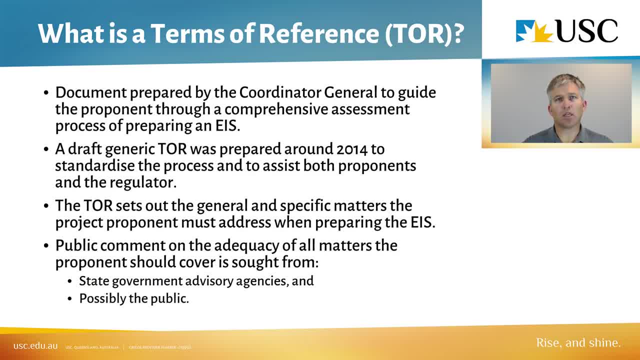 uh, comprehensiveness, in, in, in, in those terms of references, This, um diligent proponent might come with a really, really thorough uh terms of reference, Whereas the the next one might come with with a bare bones. 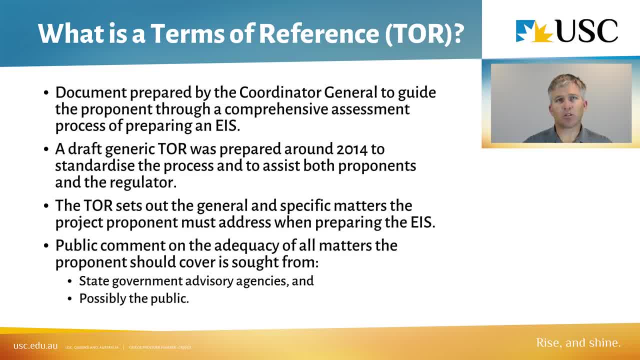 And, and so there was a, a big variation between terms of references, And, um, and it was a. you know that can extend and prolong the process. So with having a, a, a generic terms of reference now, 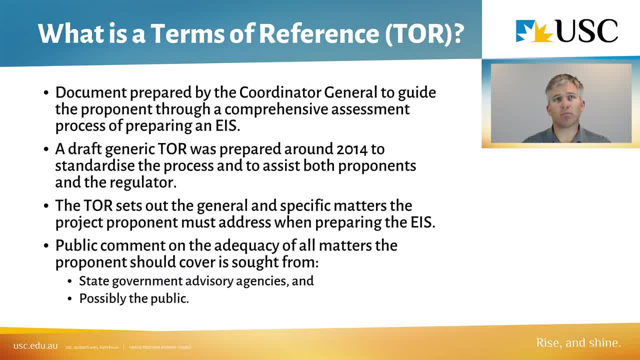 it. it's not um often requesting resources or, you know, reses, requesting intelligence from the regulator that may not have that particular specialty in the in assessing that particular type of of project, Because a a a regulator is. 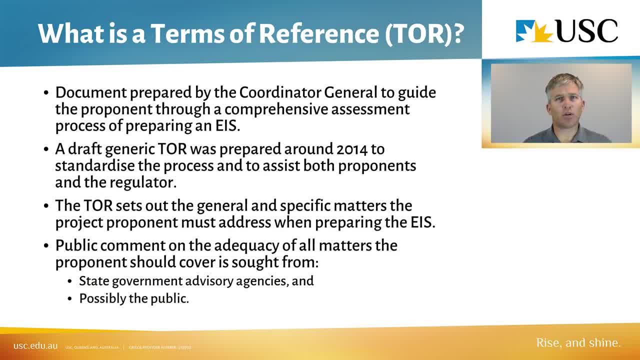 is only going to have a certain amount of expertise in a certain number of areas And and they don't have a massive resource pool to pull upon. uh within the government, Um, most of the intellectual um experience is going to be sitting out within the 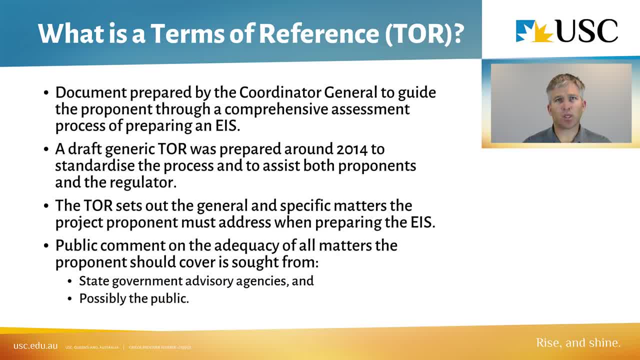 within the, the, the private sector, Um, and, and so these guys in there have only got a a limited amount of ability. So in providing that information and having a generic one set there means that they now can go and seek. 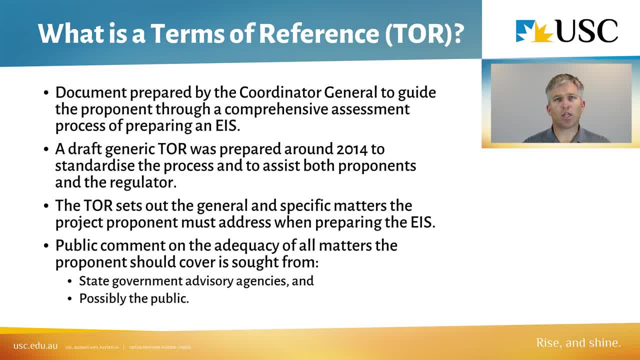 um further advice where necessary, uh, public comment and and pull that information together and then submit that out um to the proponent So that proponent can then go about going and doing that assessment and providing the most comprehensive EIS they can. 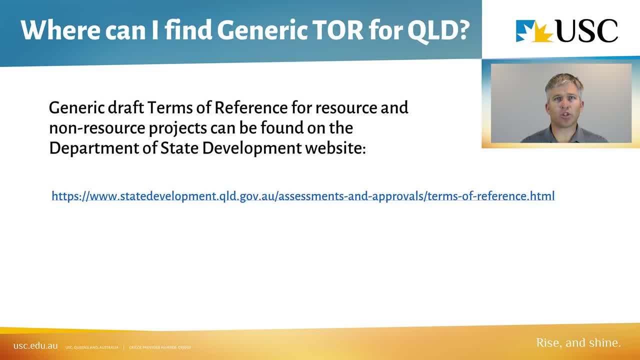 And here's a website where you can go to to find these terms of reference. On this site you'll find both um, the generic terms of references, the, the terms of reference for uh- resource-based projects- and TOR for non-resource-based projects. 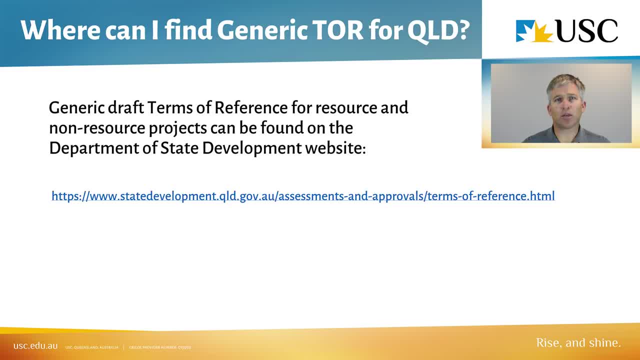 You will need the non-resource-based general- uh generic- terms of reference for the second assessment. So I would really strongly recommend you get on there and look at it and review it and become quite familiar with it Throughout this process of developing an EIS. 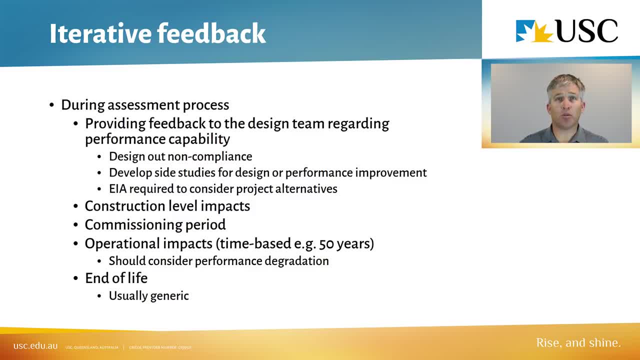 and doing the study and looking at the values, the impacts and your mitigation measures, all of those sorts of areas. you're going to be working with an engineering and a construction team and um, and to try and and pull this information together. 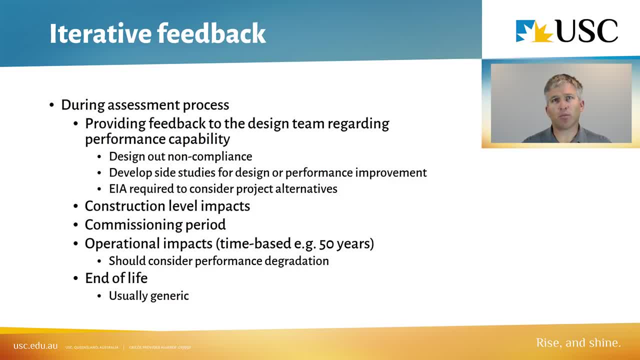 um to to get the best design um the best construction processes, uh and the best assessment, environmental impact assessment, uh and mitigation measures- out of this whole um design and and planning phase of the project. So 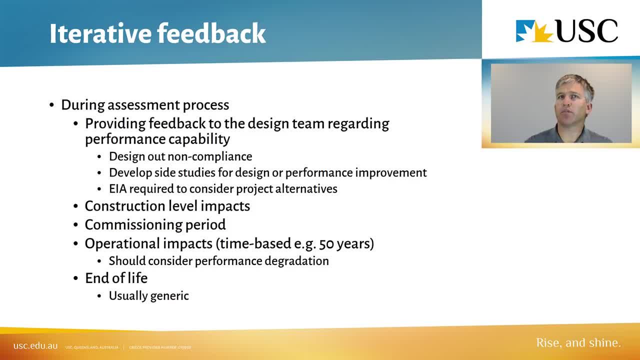 now in there there's a lot of opportunity for that iterative feedback to be able to work and and provide feedback um back to the engineers and um and construction personnel. So you might, where there is opportunity, um or risk. 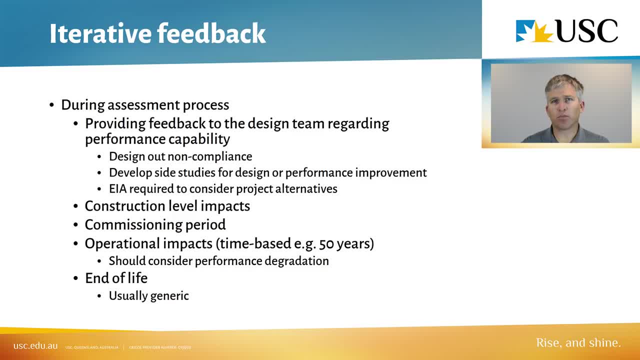 I suppose more so, for for areas of non-compliance or things going wrong, you can go back in there and have them actually design those things out. That might be a sort of avoidance. that's, instead of going through this area, we'll miss that area and we'll go over here. 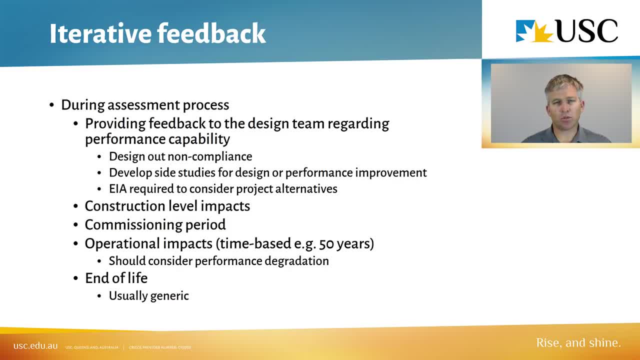 Uh, it might involve um physical designs and um people coming up with clever, uh ways, intuitive ways of minimizing risk purely through the design of the or whatever project that might be, And uh, other examples of that might be where for a. 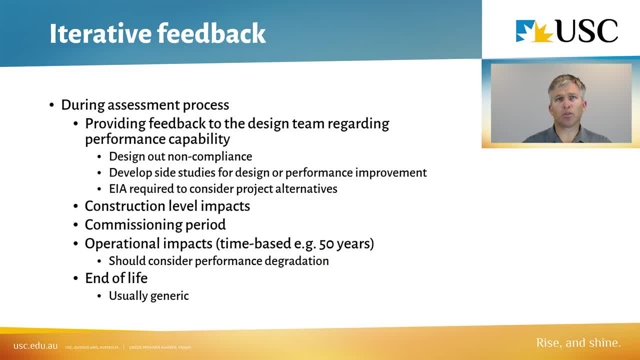 uh a corridor, for example, a road going through, to be able to design in at that point in time to put uh corridors for um or mechanisms for animals to be able to pass through, be it under or over that road. 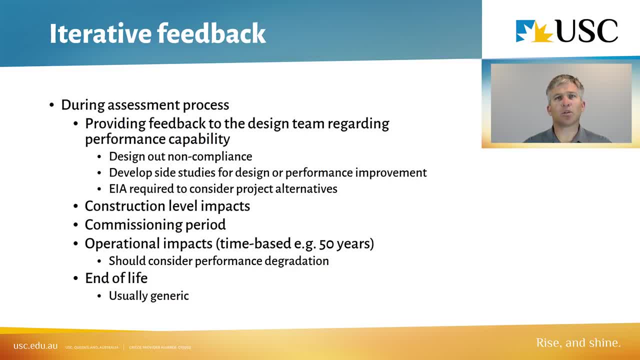 Um. so there's there's opportunity in there to to look at designing um and and coming up with, I suppose, the optimal design uh in this process so that you can ultimately minimize your impacts. uh, looking at and possibly removing the need to have certain mitigation measures in there, because no longer is that impact. 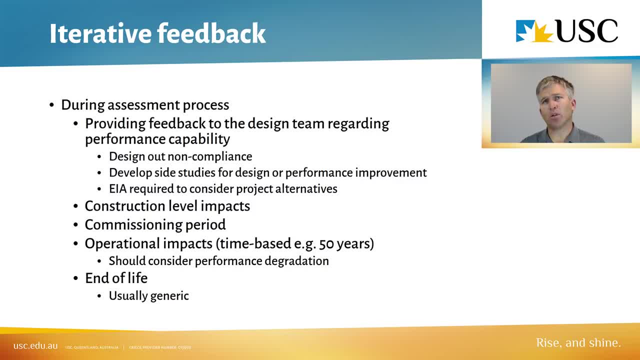 that impact relevant And that'll go right through for the whole life of the project. You want to be looking at sort of the operational phase and right through to the end of life, where it might have, you know, the decommissioning process. 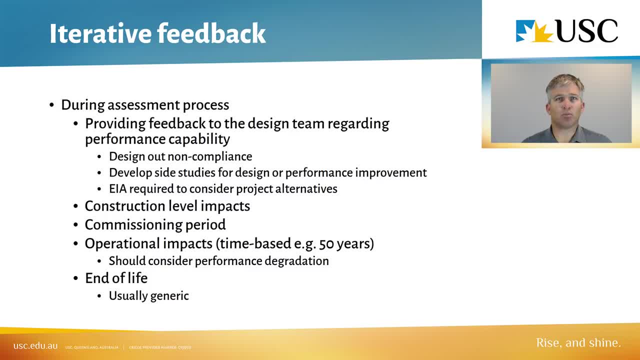 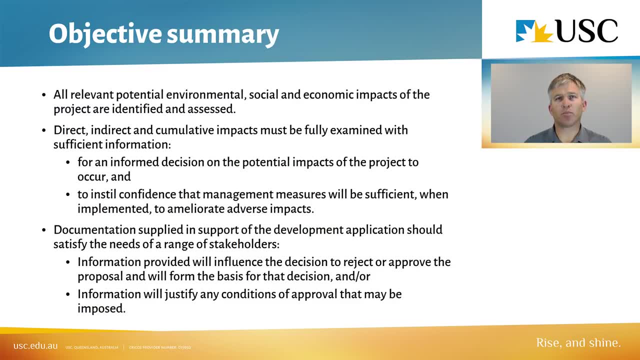 um and and how you'll go about removing that project if that's what has to happen. To give you an overall summary? um of the process, now that we've gone through the majority of the different elements of EIS preparation, we need to be looking at the identification of those values and looking at those potential environmental. 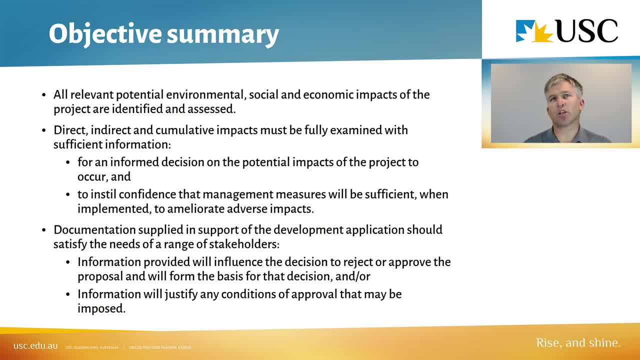 social and economic impacts that can be going on that could be imposed by your project. They might be direct, they might be indirect, they might be cumulative impacts and you need to be going right through and trying to examine the full extent of that information. 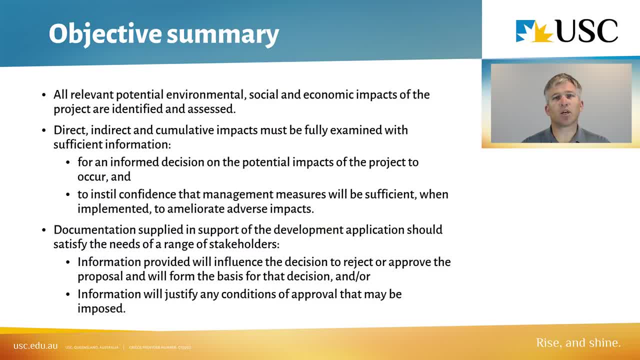 uh and with the ultimate goal of coming up with those uh- appropriate and- um, I suppose, comprehensive mitigation measures that have been able to go through that will be able to be actually and practically implemented within that project uh, ultimately to avoid any sort of adverse impacts. 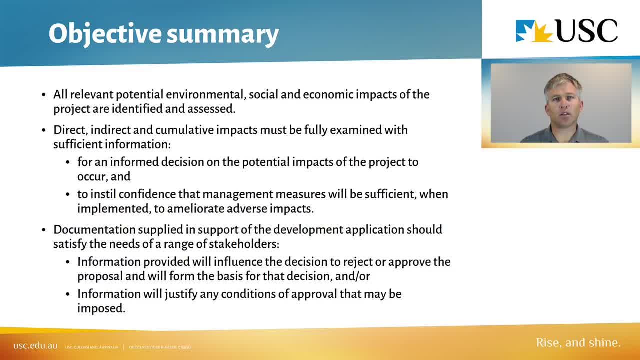 um, wherever possible, And then the the. the end result of this EIS process is that you are going to have a document, a, uh, a succinct, hopefully, um, and comprehensive document. That's going to be, that's going to. 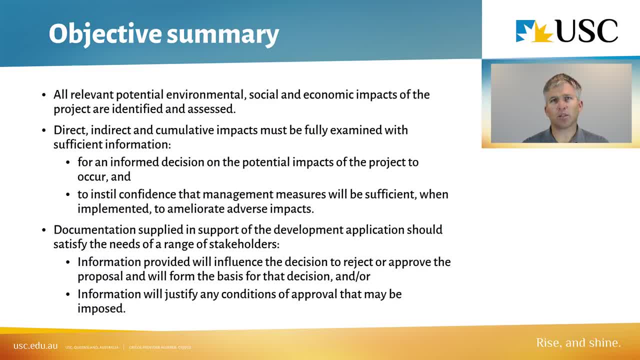 that has withstood the scrutiny of the general public and the regulators, And um. and then that whole process becomes a justification for approval, because the the regulator has to be able to justify why that project is allowed to go ahead And um. 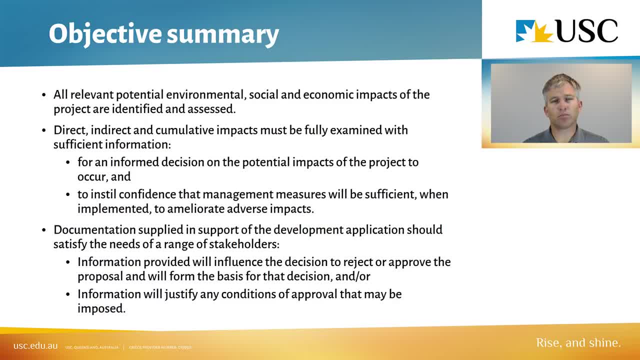 and so you know, it sort of it provides information for, for all, all parties, uh, ultimately, for that decision to be made, to go ahead and construct this project. The process also allows, uh or ensures, that stakeholders are being respected and 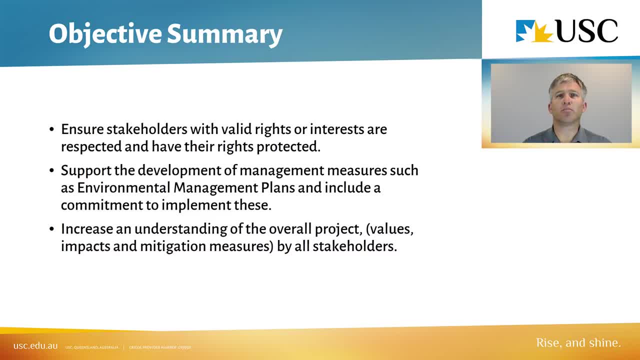 uh and have that uh rightfully consulted and had their, their interests validated And that's sort of a thing right through this process. It needs to um this, this EIS process also, and importantly from my point of view. 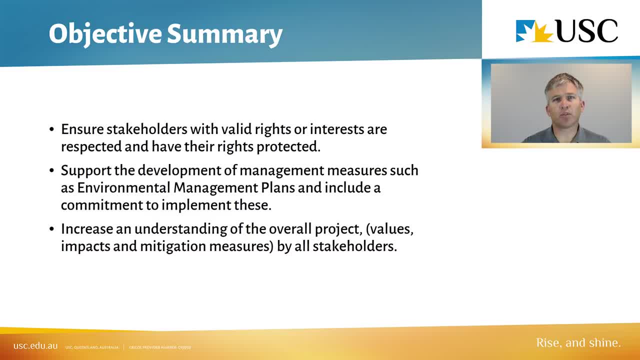 uh is it's. it gives rise to the development of the environmental management plan, which becomes a document That uh the construction team and um process live by. They then go about um implementing that environmental management plan. 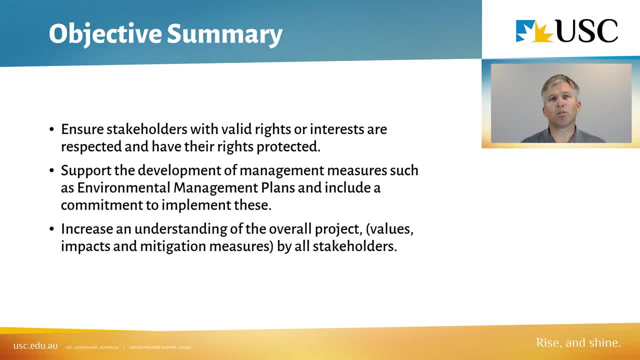 And that is what will give you that end result of minimal impact through that construction process. Um, and I suppose uh, last of all, it goes about increasing an understanding of that project, uh, increases the understanding of the environment out there. 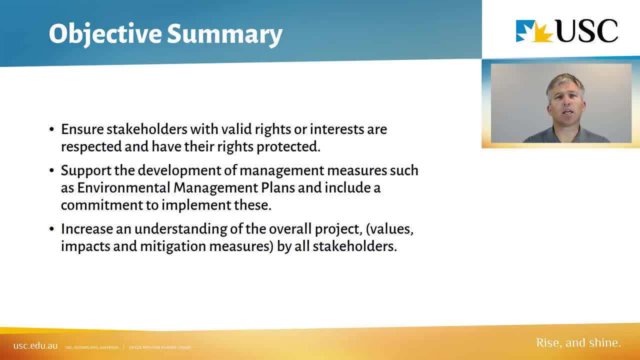 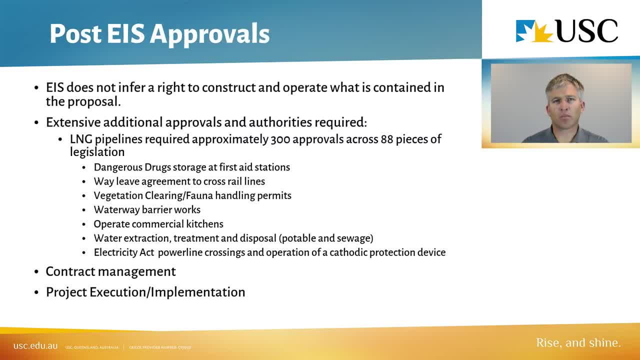 um, and then how these things can be managed. The development of an EIS doesn't necessarily uh give the immediate right uh for a project to go ahead, Uh, or the the immediate tick in the box, and nor does the approval of that EIS grant the immediate. 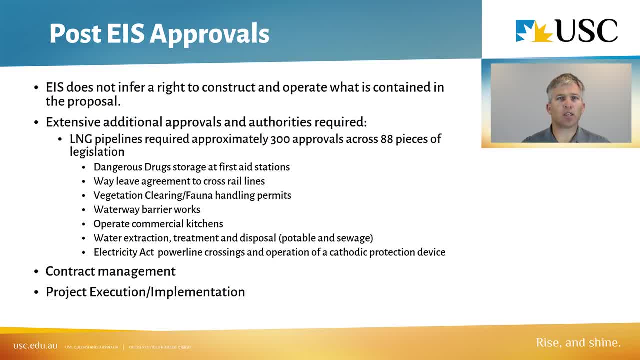 um approval to commence work. There, uh, a lot of extra approvals that are required as part of this planning and approval acquisition process, and the EIS is just one approval. it's a major approval, but it's just one approval that's required out of this quite extensive and lengthy process, and further approvals that can be required. 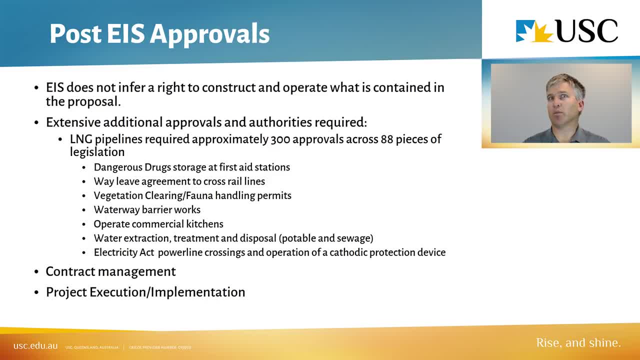 can be quite thick, almost EISs in themselves. quick, thick documents: significant species management plans, aquatic values management plans, all sorts of different values management plans, be it flora, fauna, soils, acid sulfate soil management plans. there's a huge amount of management plans and further approvals that are required post the approval of an EIS. 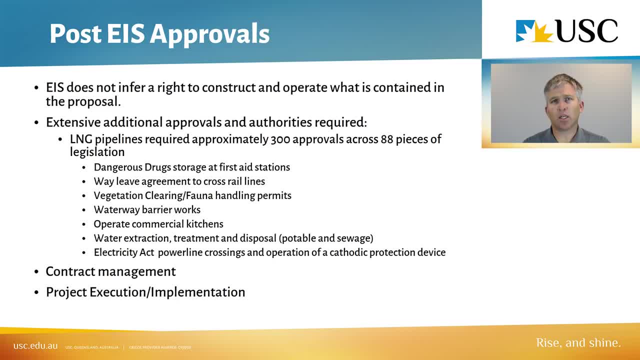 and then the EIS can be quite thick, almost EISs in themselves. quick, thick documents, significant EIS and an example: I think we had over 300 different approvals across 88 or 90 pieces of legislation within the LNG projects. that occurred in 2011,, 2012,, 2013 and they were ongoing. you might. 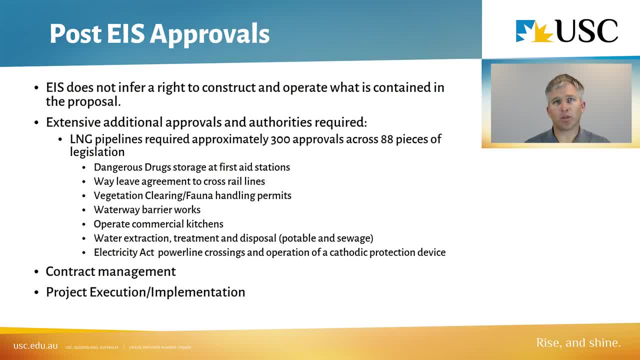 get all your approvals now, but tomorrow and the next day you'll be working in a new area and so the EIS can be quite thick, almost EISs in themselves. quick, thick documents, significant. then again you'll need to be going and getting more approvals. so there was a really extensive 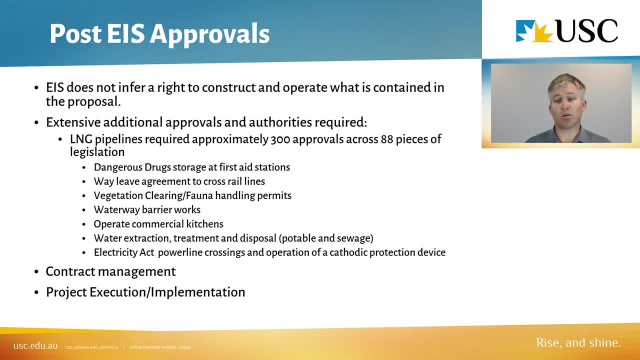 planning process that we all had to maintain. we had to be schedule it and and manage this process so that we had all the right approvals at the right times, and and that required a lot of resources. then the contract management aspect of it: once you have that EIS approved, that then goes in. 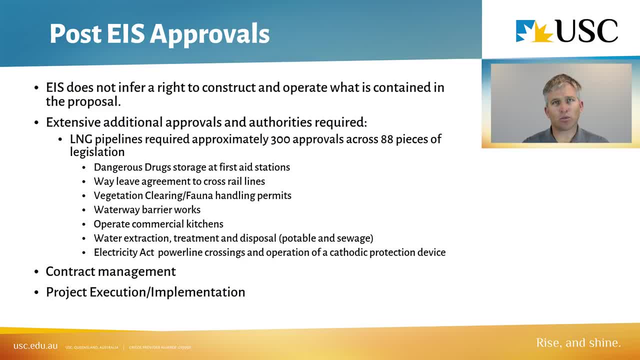 particularly the environmental management plan and the consequent approvals from that and conditions that fall out of environmental authorities. all of those sorts of things need to go into a contract, because it's one thing to go ahead and commit and say that, yes, you will do all of those things. however, you need to have that bound within a contract so that the contractor 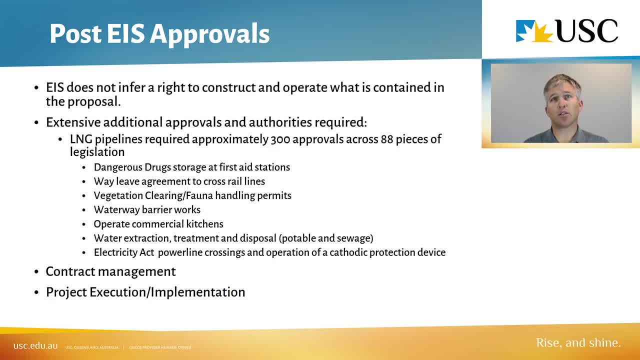 will go ahead and do it for the price that they said they would do it for. otherwise you'll be in that uncomfortable situation where you have to do these things and the contractor is not necessarily obligated to do it and you have to pay extra for him to do that. so it's paramount that in that 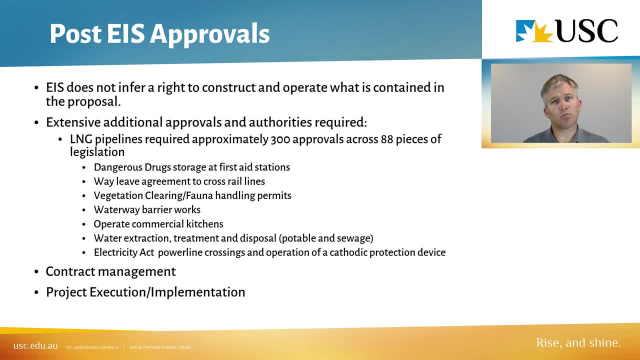 planning phase of a project and before you go ahead and acquire a contractor, that you go ahead and get these approvals so that you can put them into that contract and and and work with that contractor to to come up with a fair and equitable process to make sure all of those obligations can. 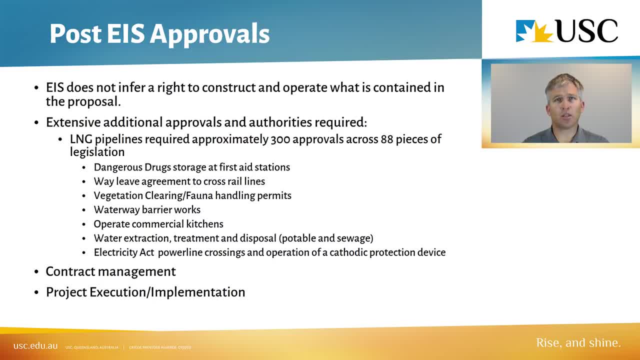 be met and then you can sort of get to the the pointy end of the stick and finally you'll be able to go about and actually execute that project at that project and implement it, go ahead and and put all of your hard work to use. this little picture has been put together to try and demonstrate the fact. 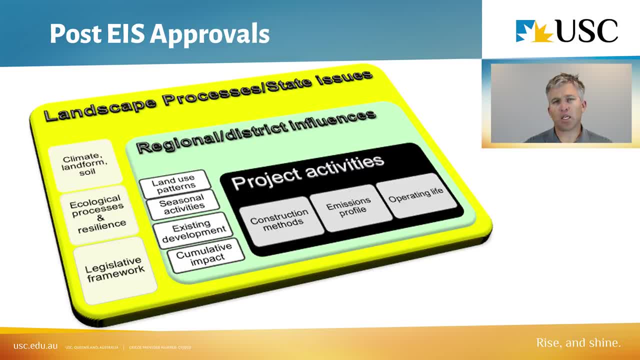 that you know there are many fields of influence within an eis process and the and overall that approvals process, and you need to be able to remain across them all. now there's a lot going on within the project and so you're dealing with the construction processes, the operational processes that might be coming up and the different impacts that might be. 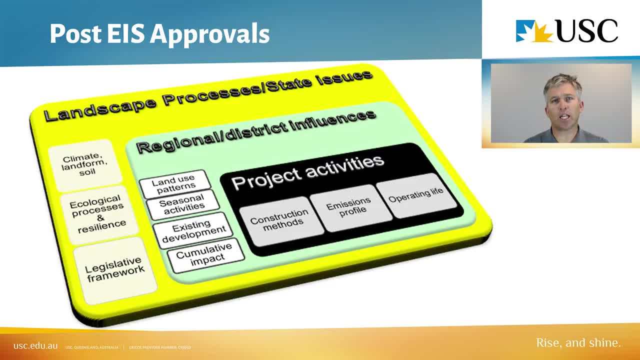 immediate for the team right then and there. but then if you're moving out into that regional district sort of a level, there's influences coming in from the, the land use, seasonal activities, existing development, cumulative impact, other projects going on in the area, other other influences from that more. 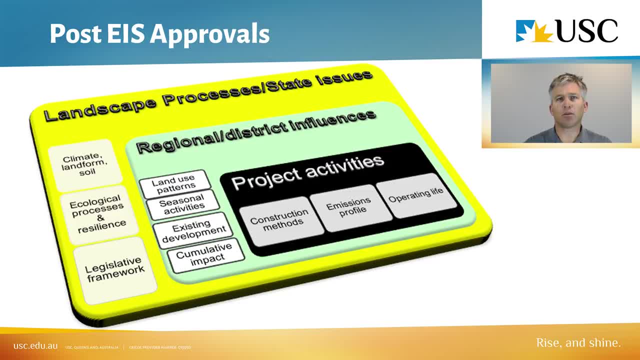 regional level and then if you go even further out to a state sort of level, and we're looking at the climate, the landform, things you need to be taking into consideration, should we be opening up this Creek now, given that it's likely to rain next week? probably not, you know. you need to be planning. 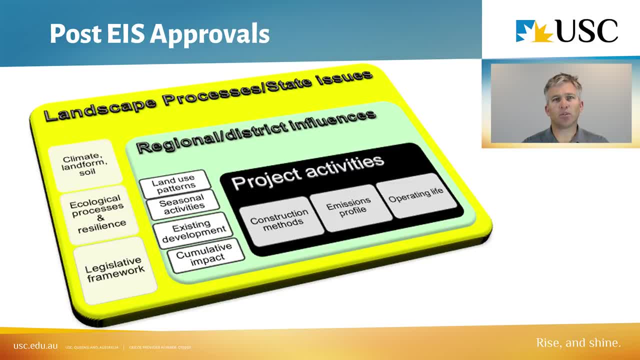 and looking at that greater level of influence right through to legislative frameworks and things that are at play. but so there's a multiple levels of influence within this process and you'll be continually juggling it and continually managing it post approvals. because of that, you generally on particularly linear infrastructure where you are moving at a fast pace. 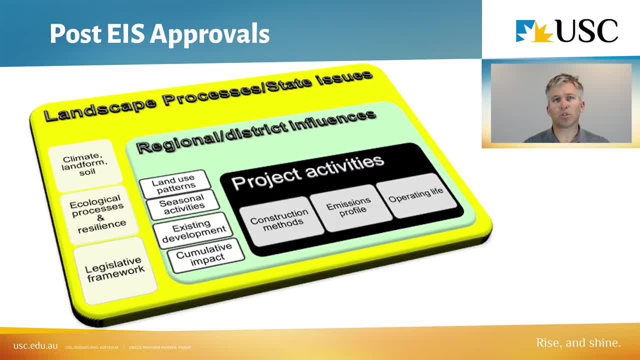 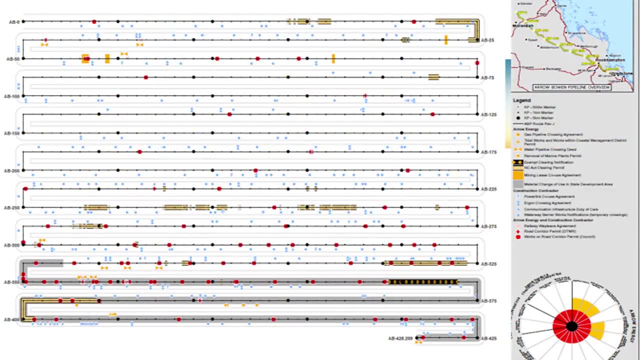 you'll be coming across new things regularly: new environments, new, as I say, all of those things there on that slide, this slide off, incorporated just to sort of demonstrate some of the how information can be displayed and and used, and, as the consequence, slides are the same as well. 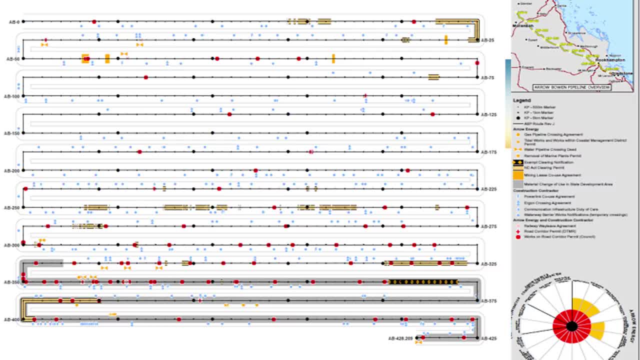 and we'll run through these. but this, this is a snake diagram. it's from a pipeline project. obviously the pipeline wasn't shaped like that, but it's been put into this so that we can see on a kilometer by kilometer basis what uh different risks or values or what. 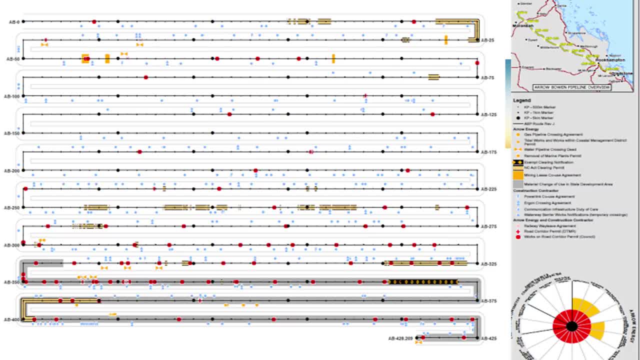 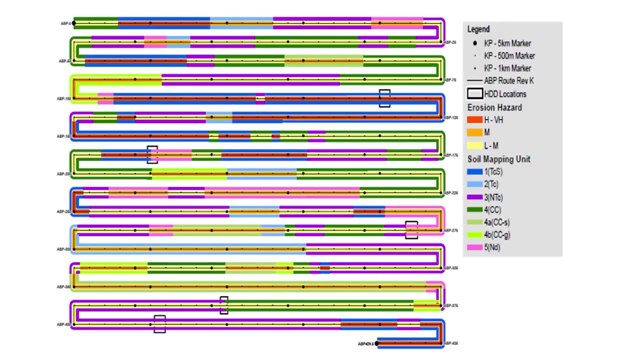 issues might be coming up so that they can be managed accordingly, and and so, as you have progress moving through, you can see that we've got all of these different issues that will need management of some sort. then we go down to the next slide, and it's just another way of displaying all this sort of uh information on the 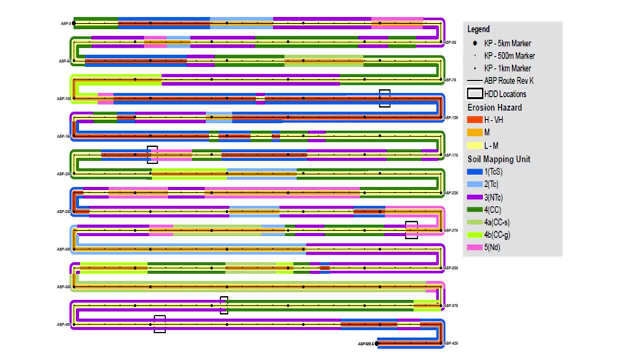 right hand side. I've sort of left it a bit blur. I didn't want to disclose you know which project was using this sort of information, um, or you know too much as to where it was, but we're sort of looking at, um, there's erosion hazards, we've got soil mapping units and things, so it allows this. 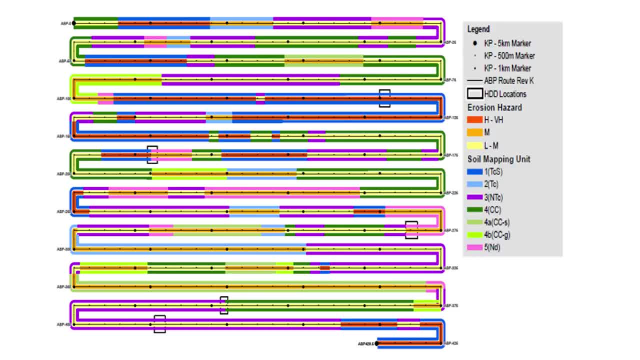 sort of information displayed in this way allows us to be able to think: okay, this is the sort of stuff we've got coming up. this is what we need to manage. we need to have approvals or we need to have. we might need to have gypsum in place waiting for that. 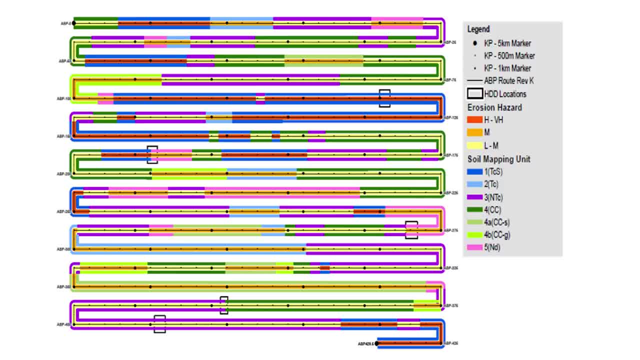 thing, or we might need to have, um, you know, alert a landowner or um, yeah, so all sorts of things that might need to be done when we get to a certain area. but it allows planning and um, and I suppose, ultimately, that's what an EIS is intended to try and do, apart from allow an approval process. it'll. 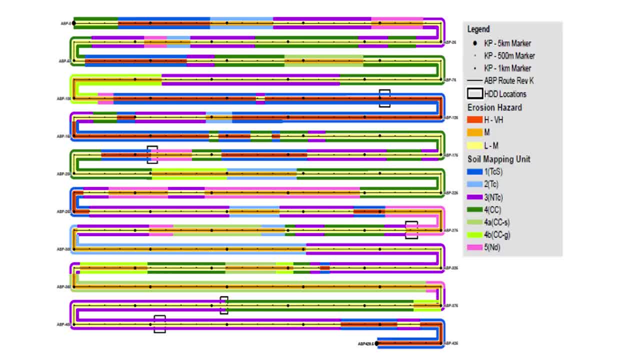 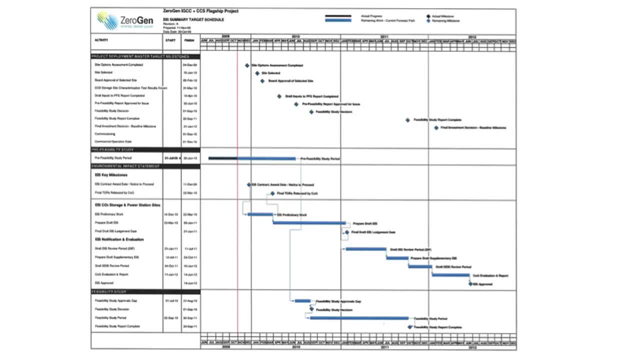 it encourages planning so that you can go about managing your risks and applying the correct measures as needed. here is a Gantt chart. well, I've already introduced you to the concept of a of a Gantt chart, but that again allows planning um and and and Gantt chart. 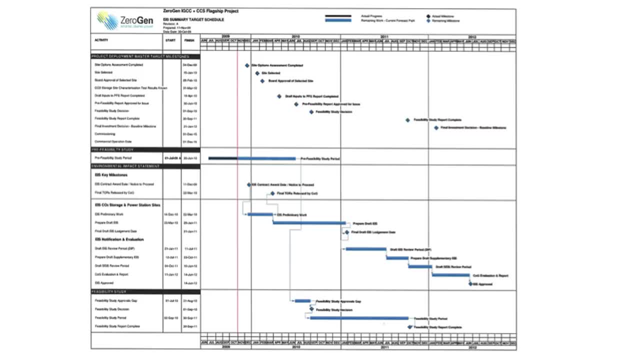 so. so that time, resource and and can be um, um financial, but you know the cost. but we're looking at um how we're going to manage resources within certain time frames and meet milestones and achieve certain things. might be you might have allocated certain approvals to be awarded by certain dates, so 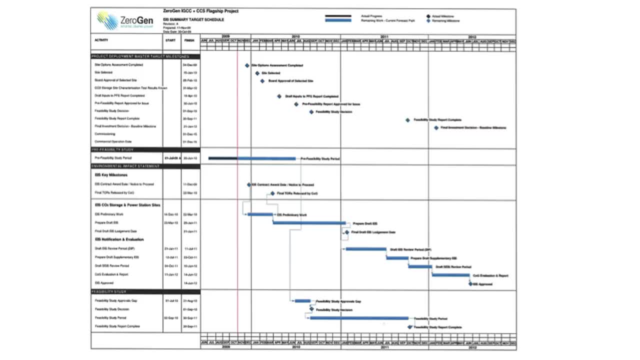 um again, charts are other mechanisms that are used throughout this approval process, and there are heaps more. they're just a few examples I just wanted to sort of present for everyone to have a quick look at and consider, and I've got a couple of stories where you go about through that. 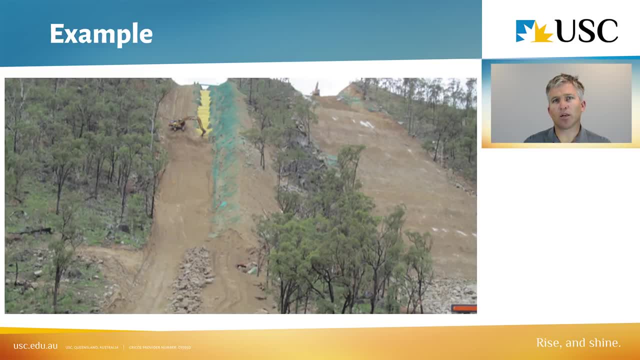 implementation. these are a couple of pipelines that were installed towards um, or heading from the, the Coliseum gas areas, and that went through to Gladstone. um, as you can see, they're going through um. the yellow things being installed up there on the, the pipeline corridor on the left, um they're trench breakers and they sort of go through and 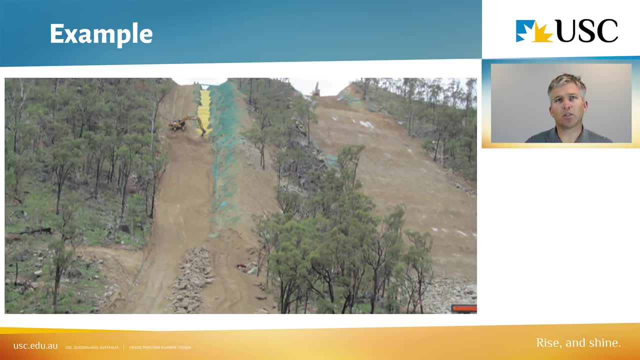 they have to to manage the loose soil that's placed back into the trench, to try and manage the so that prevent that water from going and washing it out too much, because obviously if you've got an undisturbed area where the soil has been removed and then placed back in, uh so or disturbed, 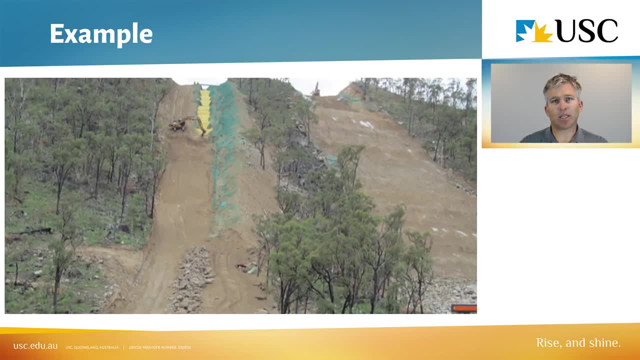 sorry area where the soil's been removed and then placed back in around a, a long cylindrical object that runs all the way down the hill. that's where the water is going to want to run and it's going to go through and it's going to take out that soil. so so in doing that, there was a lot of planning. 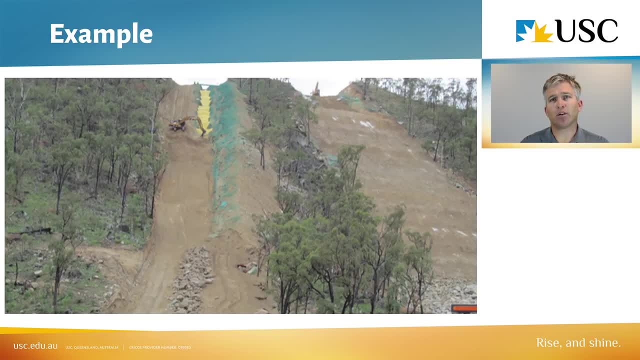 um for certain measures there. however, this area came across um some massive problems because of the. so, ultimately, a lack of approvals and a lack of planning, and we'll just go through and have a bit more of a look, okay. so this picture here is that pipeline that was on the on the right. okay, 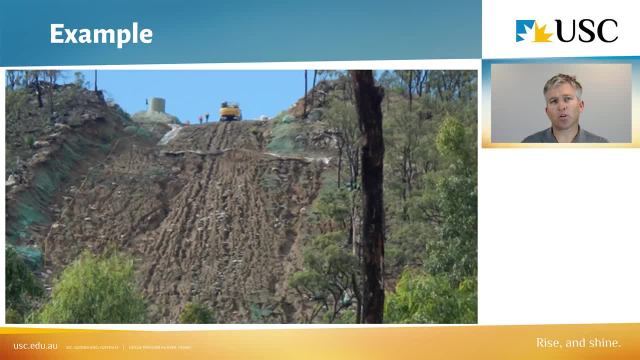 there's the the right of way, that's on the on the right hand side there. now that was the first rain event that occurred and now there was quite a significant amount of scouring and movement of soil off the right of way and and down into the creek, and there had been with this particular 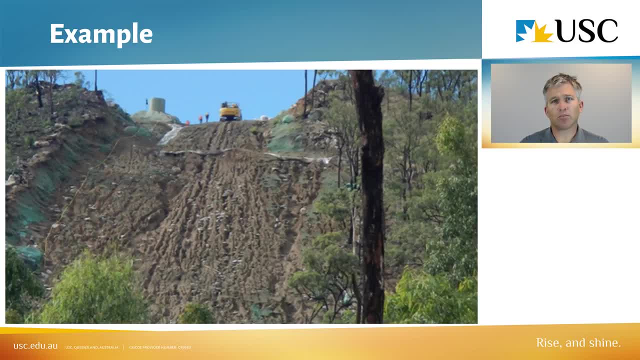 project. there had been very little. um, well, there'd been a certain amount of planning going there, but the requirement there was that there needed to be certified erosion and sediment control plans put together by a, a certified practitioner of erosion and sediment control, and and that didn't. 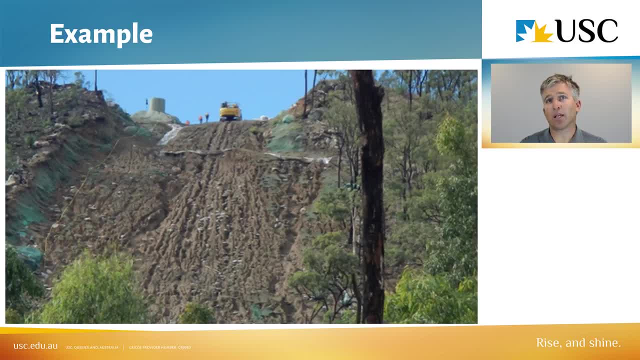 happen, and then the proponent allowed the contractor to go ahead without doing that. so i, i, you know sort of um, there were issues there from uh, both sides. it shouldn't have been allowed to go ahead, but it did and it rained and uh, and so consequently, we ended up having a lot of scouring. 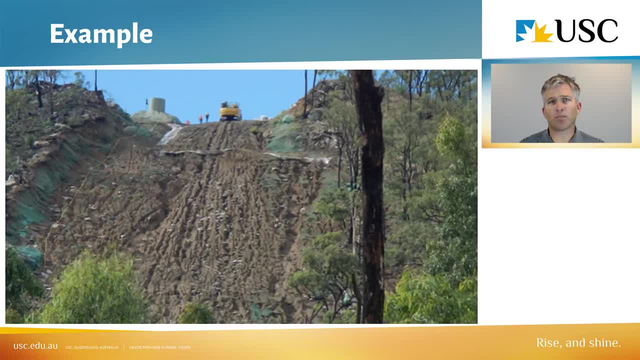 there, they went back and they fixed that and then it sort of they that was sort of- after they fixed it again and then it rained again and so this significant amount of of scouring and damage occurred to that area yet again and, um, and that's still ongoing and i think that will be ongoing for. 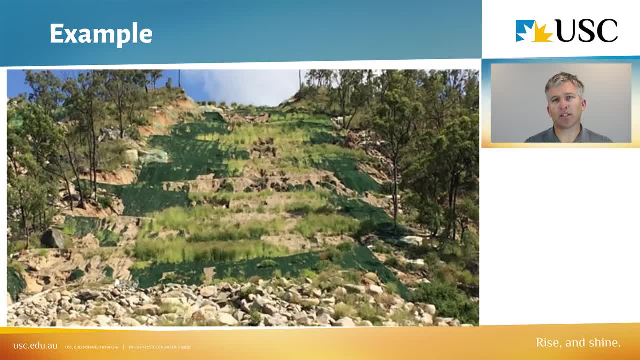 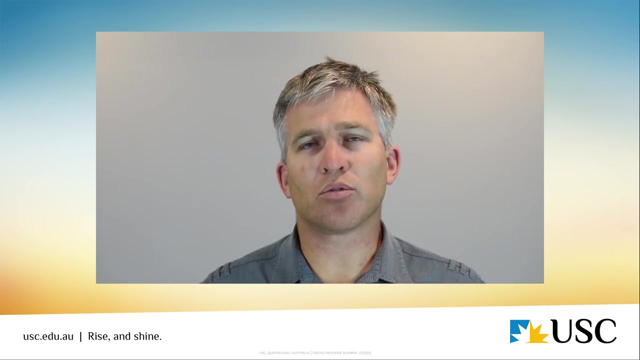 a very long time because of the lack of planning that occurred on this project. uh, with regards to this particular area, it's it's created a legacy of um, a very problematic area that's going to have issues that are going to persist for a very long time. as a as a conclusion to this whole process, i want to strongly suggest: 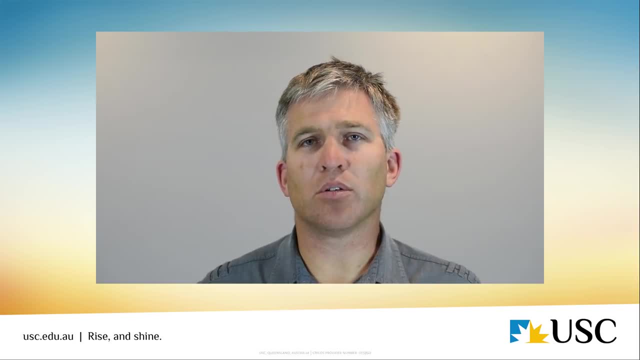 that you go through and do the most comprehensive form of assessment that you possibly can, identifying all of those values out there, those impacts that could be imposed and um, and to properly assess and evaluate those those impacts and come up with detailed, strong and and robust mitigation measures that can go about the overall management of this, of those impacts that may be.